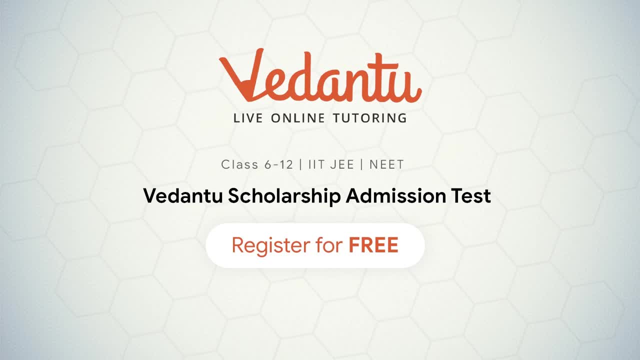 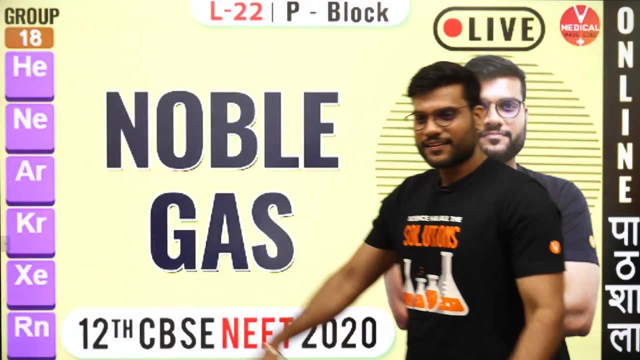 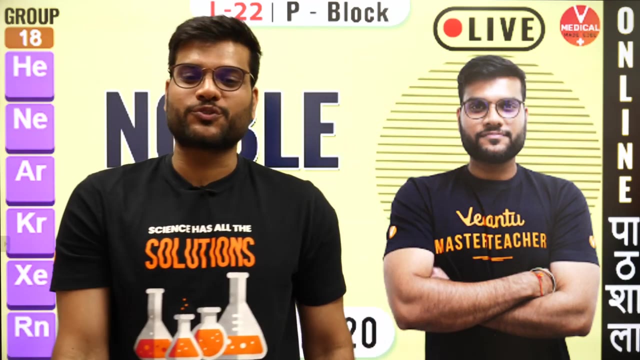 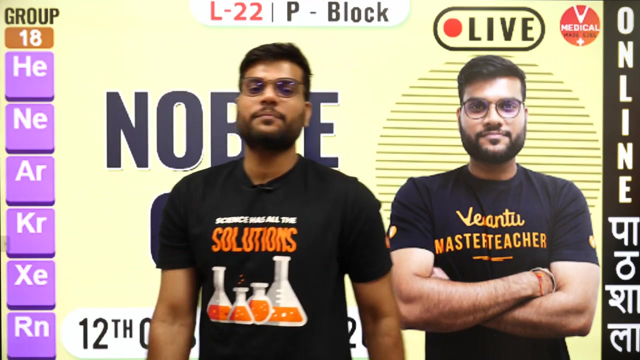 made learning a very fantastic experience for us. How are you all? I am very happy, and today is a very big celebration day for us in Vedantu. That celebration day is so big that I want to share that good news with you all. I will. 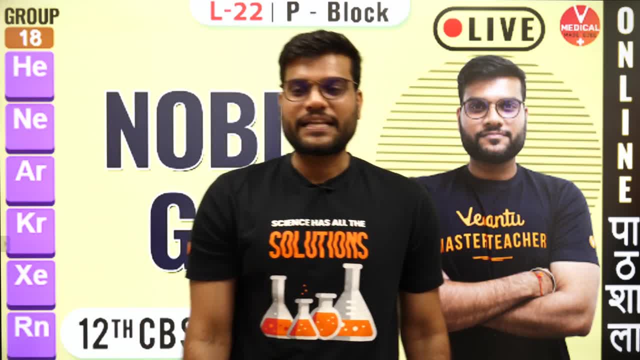 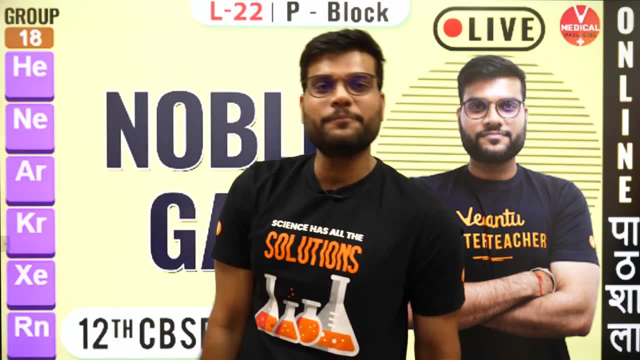 share it in some time. How are you all? Do you know what we are going to do today? Today is group number 18, lecture number 2.. We are going to talk about the topic of the day. 122 is the last lecture of P-Bloc. After this, our P-Bloc is finished. Now we will. 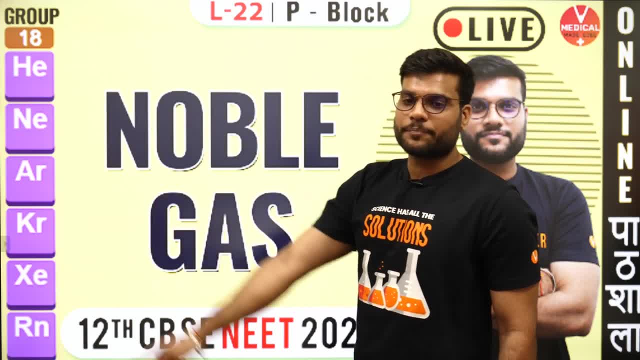 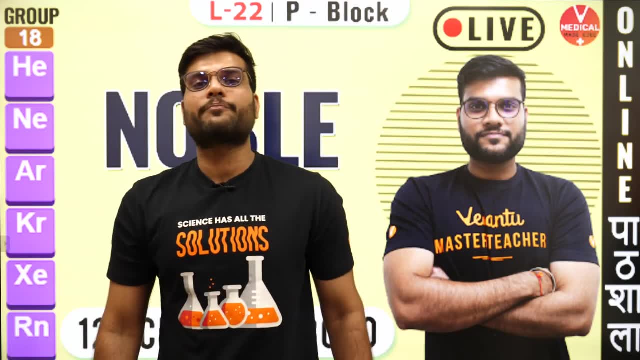 move ahead. What are the gases? Helium, Neon, Organ, Krypton, Xenon and Radon are the noble gases and this is going on online, India's biggest program, in which we are getting you prepared for NEET BOARD, and JEE 10th and 9th are also going on. Everything is going. 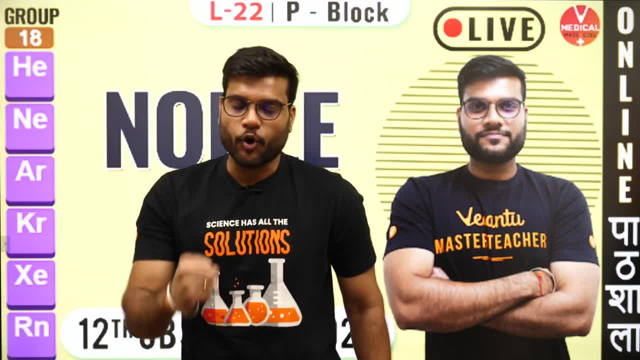 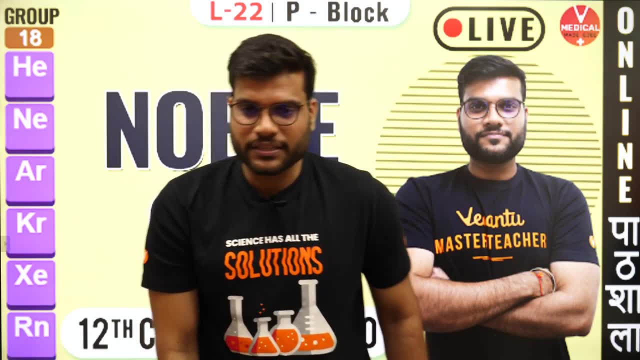 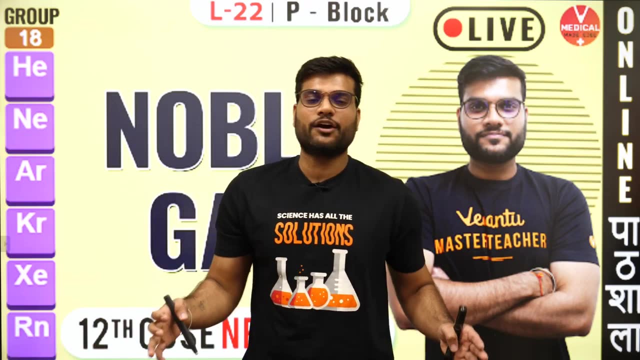 on. But what do you have to do? You have to support the curriculum of this online school so that we can teach you very well. Let's quickly start. But what is the good news? Do you want to listen? Today is a very big celebration day in Vedantu. It is a very big good news, So I will tell you in. 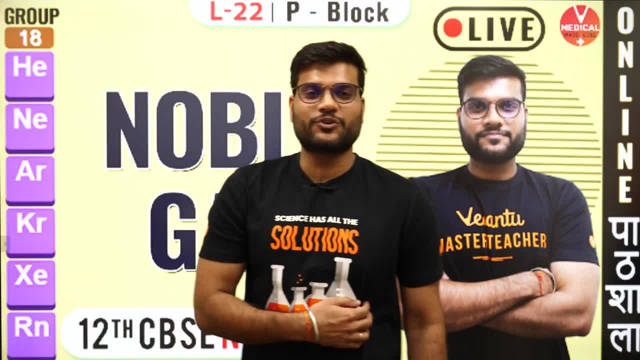 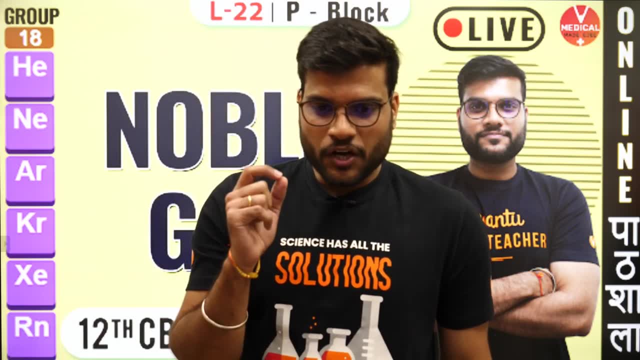 some time, But all of you who are watching the live session, you have to take their name, So let's take it quickly. I can see Kavya Nitika, Neha Bharraskar, Dilip Kaul, Faiz Meera. 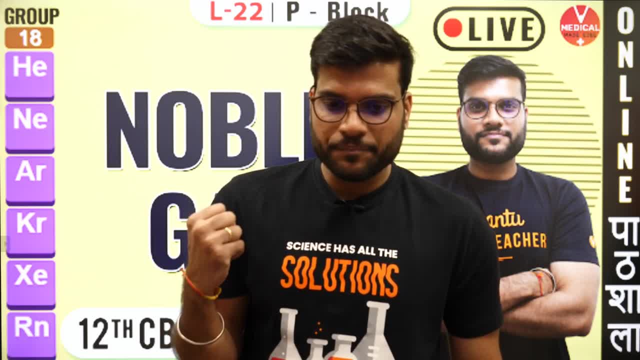 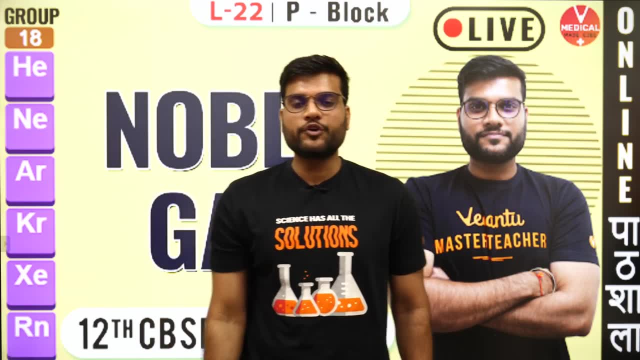 Shipra, Sonam Okay And Ayush Sneha. Wow, Thank you so much for coming, Shipra, Very good. Thank you so much for coming, guys. Love you all guys. Thank you so much for coming Now I. 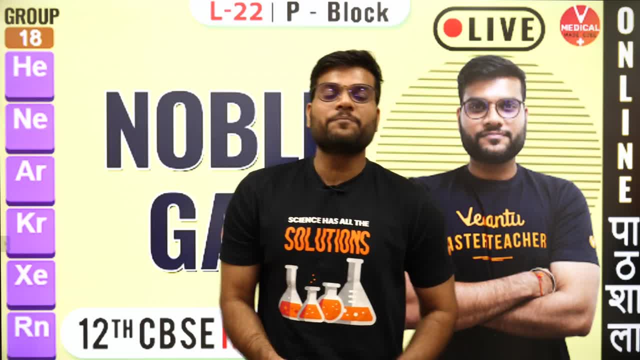 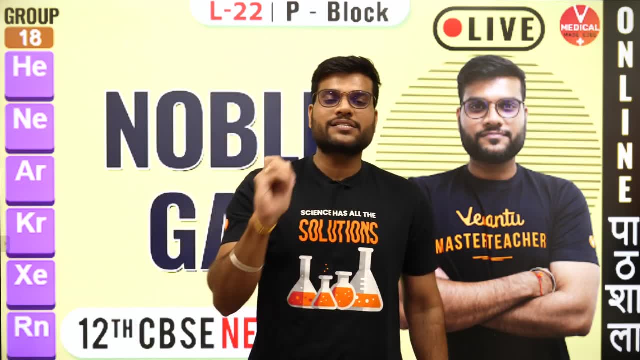 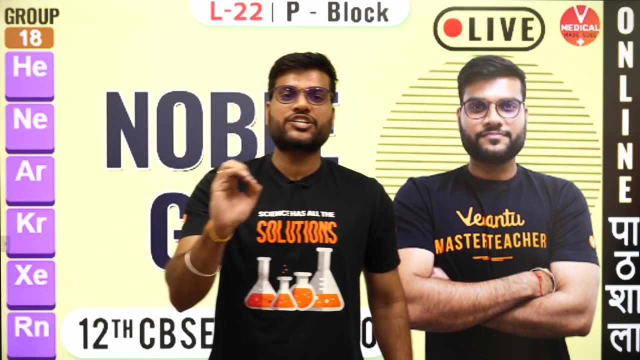 am going to tell you a very big news. In the entire history, in the complete history, till today, this has never happened. Vedantu is the only startup company which has got such a big funding. Yes, In all the education industries. in today's time, education is. 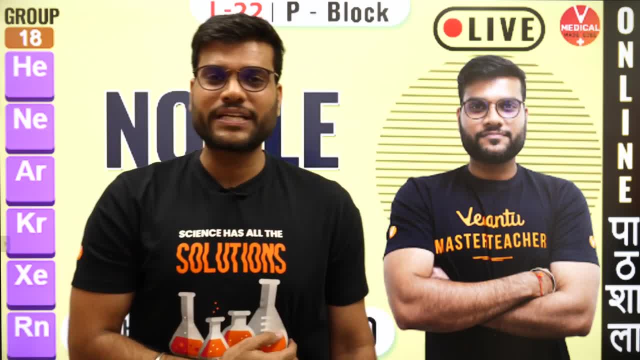 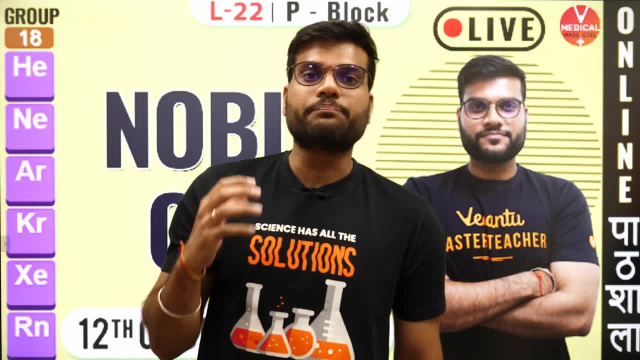 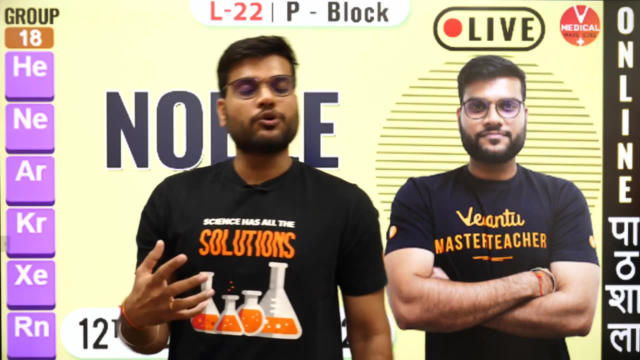 being delivered to the children. Talk about online education. offline Never got such a big funding. Vedantu has got a lot of funding on an international level: Funding of 41 million dollars, Which is a very big thing. Funding means you search that. Okay, I will leave. 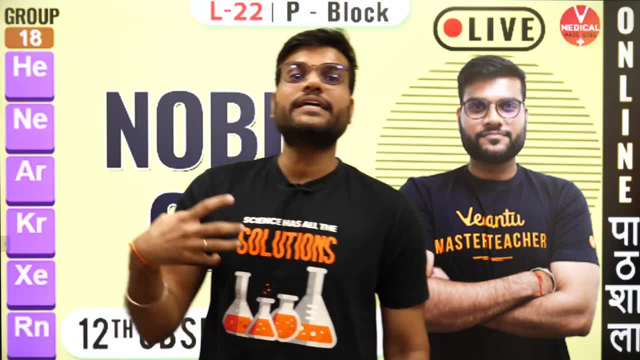 it there. But there is a very big support which is a slap on the initiative of Vedantu, that Vedantu is going in a lot of directions. Really, Vedantu is going in a lot of directions. Vedantu is going in a lot of directions. Really, Vedantu is going in a lot of directions. 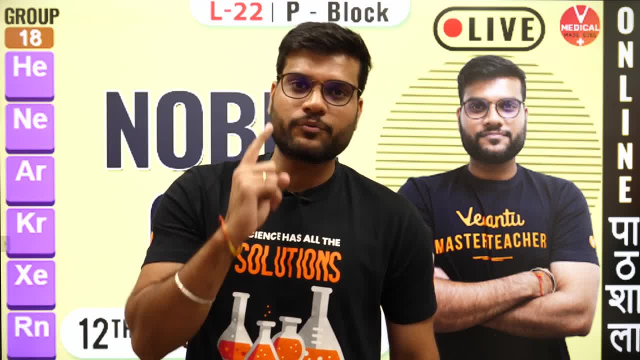 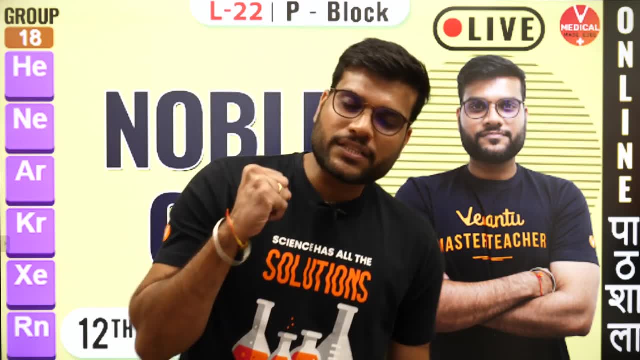 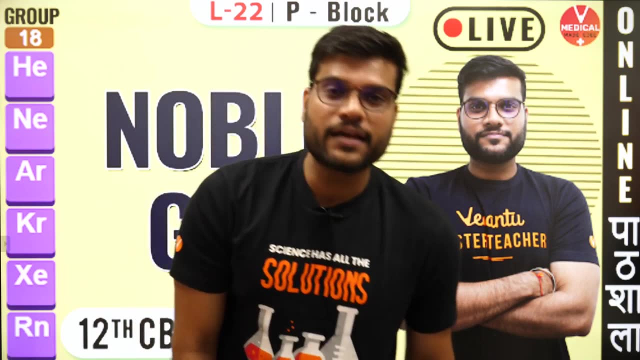 It is doing a very good work and you have to take this work forward And you have to support Arvind Arora Vedantu so much that the names of Vedantu should be on the children's tongue, And for this the founders of this company are the heads of. I salute them very. 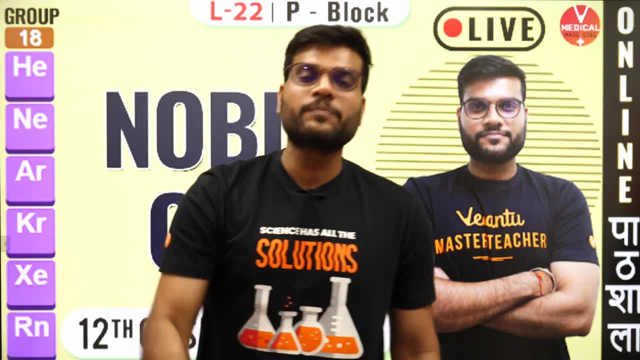 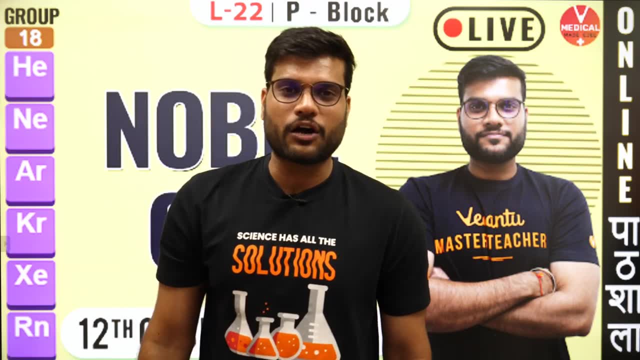 very, very, very respectfully. Anand, sir Vamsi, sir Pulkit sir, because of whom, really, our dream, my dream, is being fulfilled- to connect with you, And the name of Vedantu is being spread far and wide, The biggest, in fact. this data is also coming out that it is the 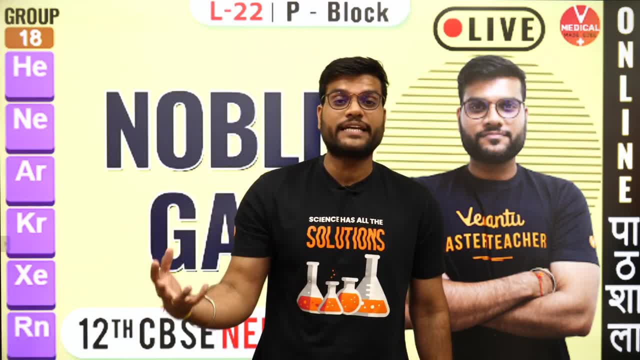 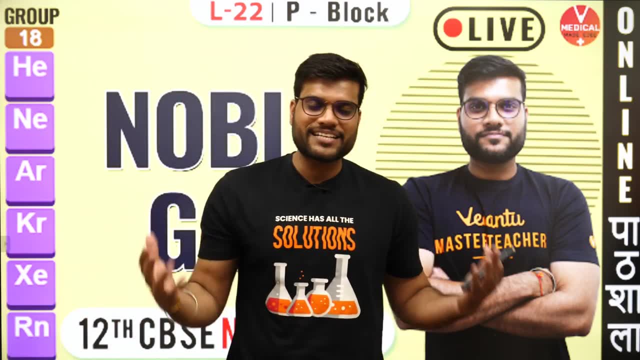 biggest company of the world which has got such a big funding at C level. Such a big funding has never been given to any company. So these are your blessings which are raining, And if you people would not have given so many blessings, then maybe Vedantu I okay. 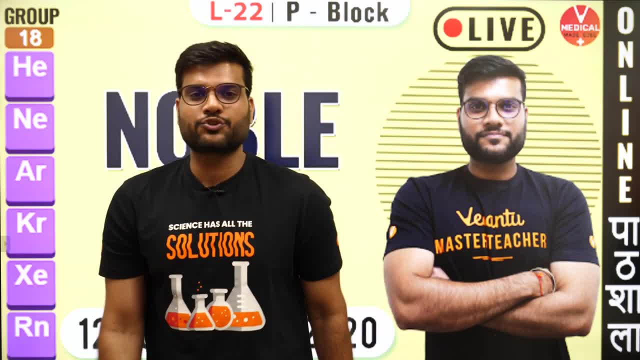 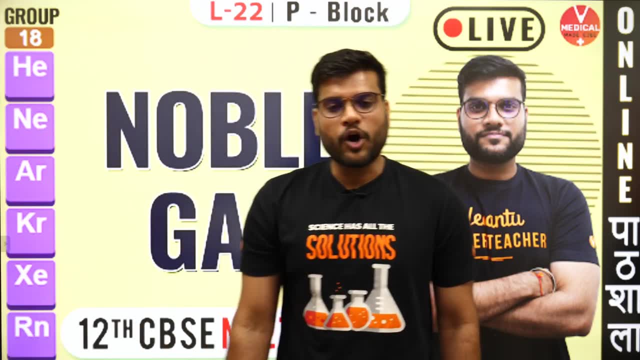 we people might not have reached here. So let's quickly start today's session with this good news. Thank you so much for supporting us like this guys. Thank you so much for supporting us like this guys. Let's go. So this was a very big good news. Now let's. 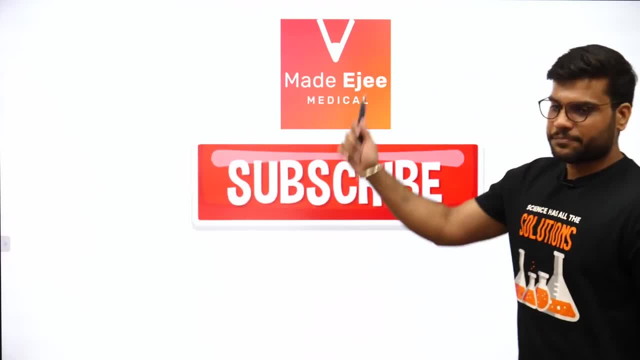 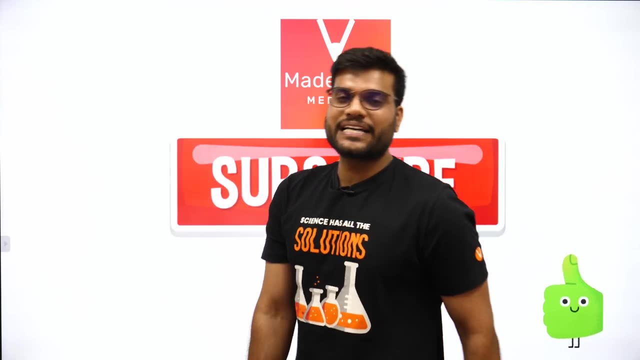 move ahead. I have told you the good news, But I say again, it is the day of good news. Okay, It is a very big day And what you people have to do is you have to become a part of this Vedantu family, You have to become a Vedant, And if you people want to become a Vedant, 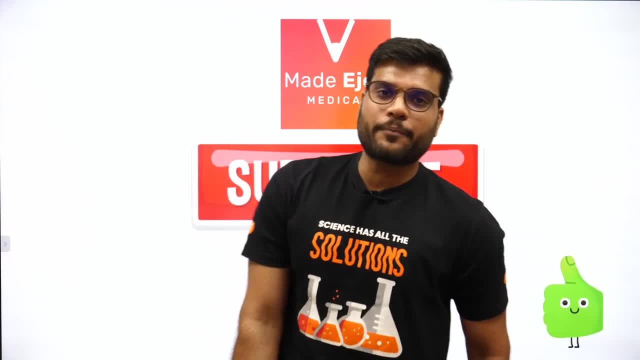 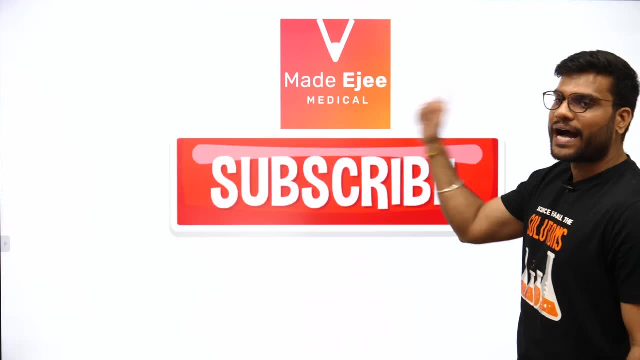 then please subscribe to the channel. The biggest, the biggest program is online reading. There is no bigger program than this. So, guys, I am requesting all of you that, please, you can move forward with this initiative And Vedantu Medical Made Easy Channel, which. 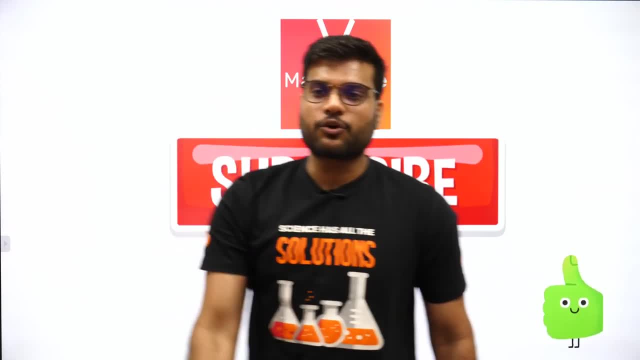 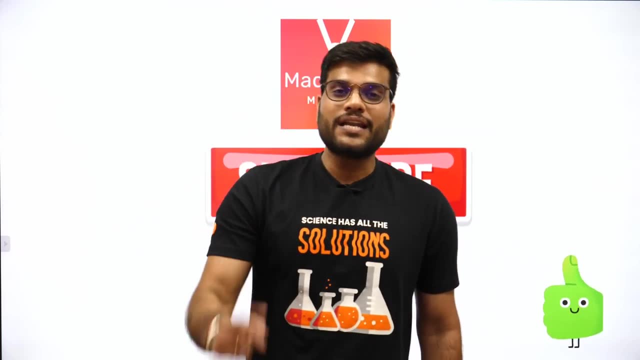 is the number one channel in NEET in India. please subscribe to this channel because by subscribing to you people, our relationship with you will be made, And not only our relationship will be made. we will take Hashtag Coaching Free India far away. So I am requesting all: 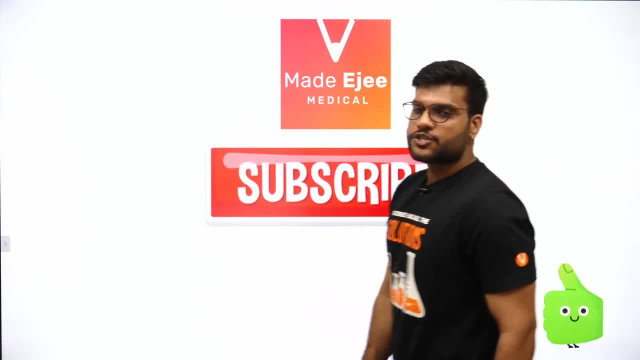 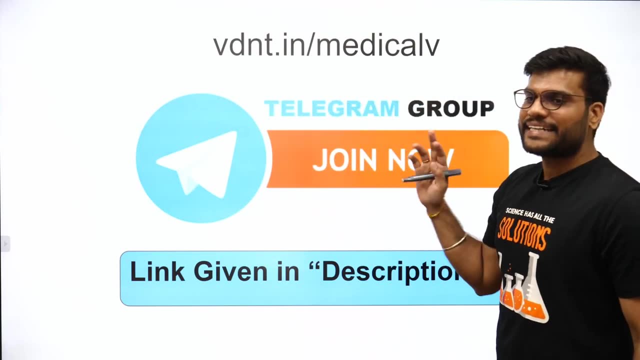 of you that please? you people must subscribe to this channel, So I think you people must have subscribed And, apart from this, you can also subscribe to VD&T dot IN slash Medical V. This is a telegram group which has been joined by more than 5000 children, So please join. 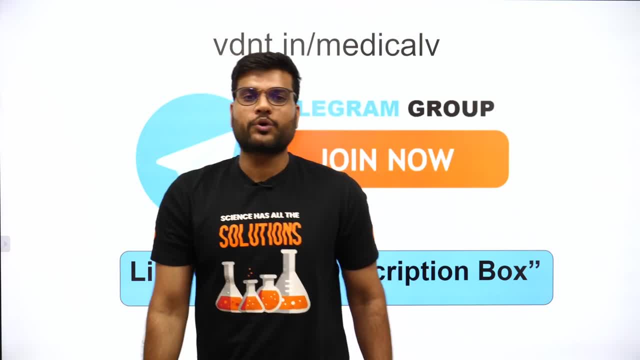 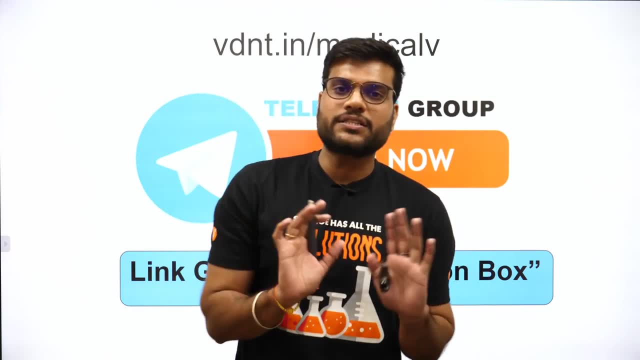 it. Come on, guys, let's start group number 18.. It is very interesting And today I will finish it. Okay, So look very carefully. I will make you do all the important things in it And after that we will start a new chapter. So today is the last day. Yes, the. 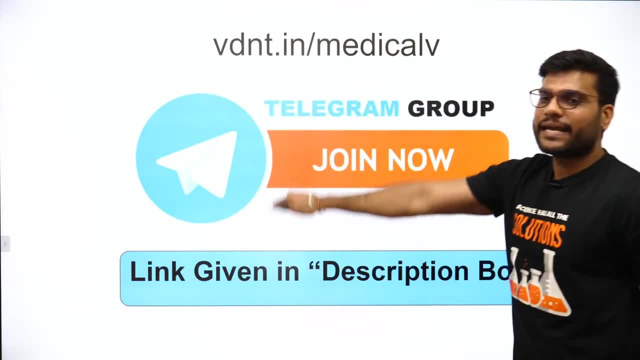 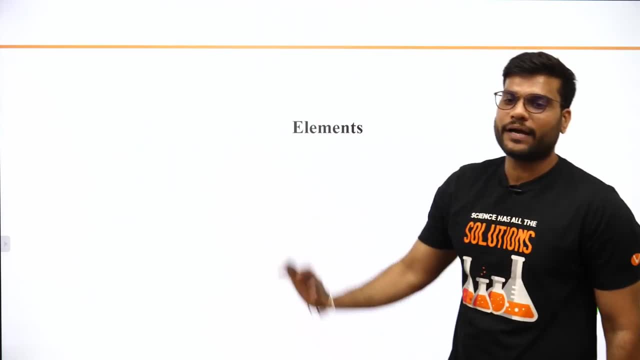 last day of P-Blog, So let's start quickly, But I tell everyone to join the group quickly. You will be able to be directly attached to us. Come on, guys. First of all, I will give you a glimpse of the elements. Okay, And here is a property that you have to pay attention. 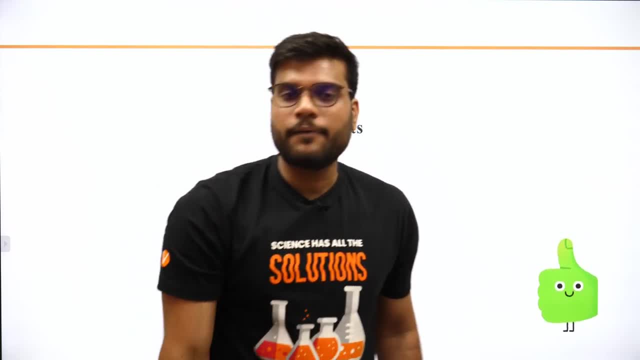 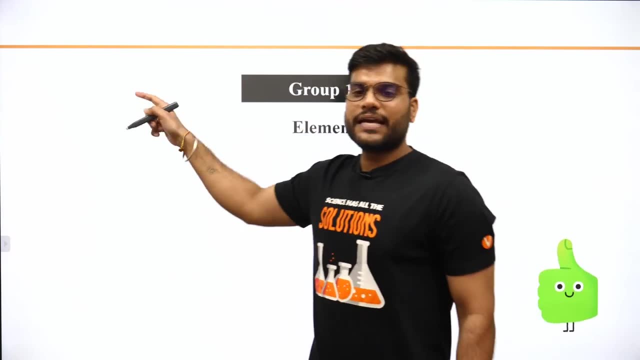 to Here. I will write a property along with the element And actually there is a question on that property. You guys pay attention. What are the elements of group number 18?? Yes, Helium, Okay, Of group number 18.. Please check carefully Which are the elements. 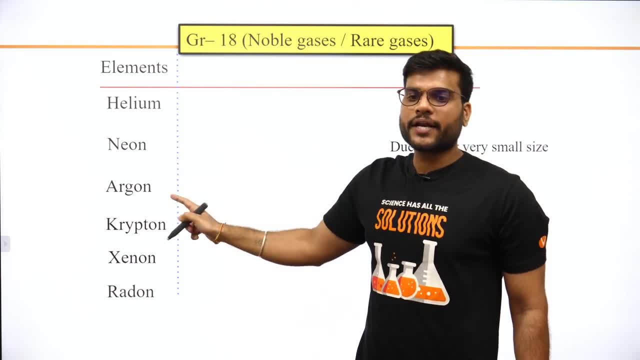 Yes, First of all Helium Neon Organ, Krypton, Xenon, Radon. Okay, Now here, everyone knows this, We call them Nobel Gases. Okay, So first of all Helium Neon Organ, Krypton, Xenon, Radon. Okay, So first of all we call them Nobel Gases. Okay, So first of all Helium Neon, Organ, Krypton, Xenon, Radon. Okay, So, first of all Helium Neon, Aeron Cyanon. Okay. 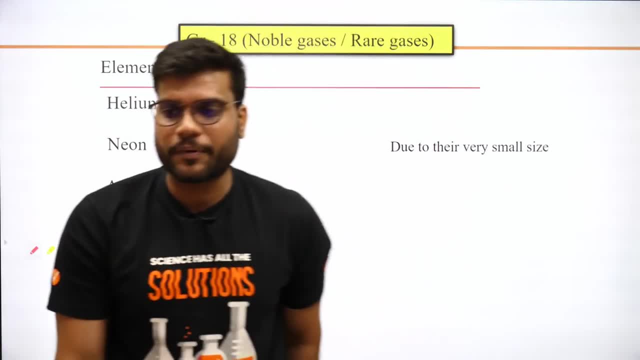 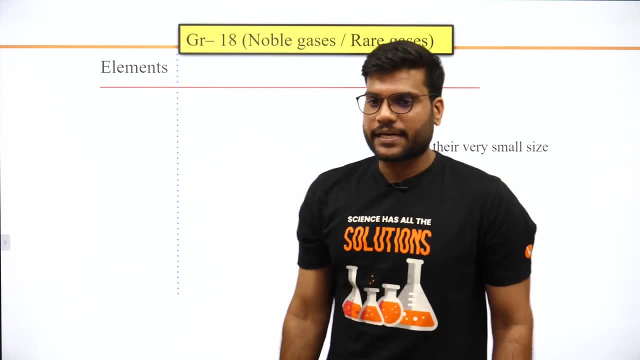 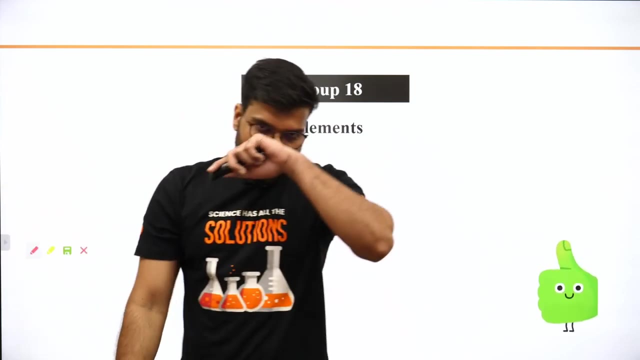 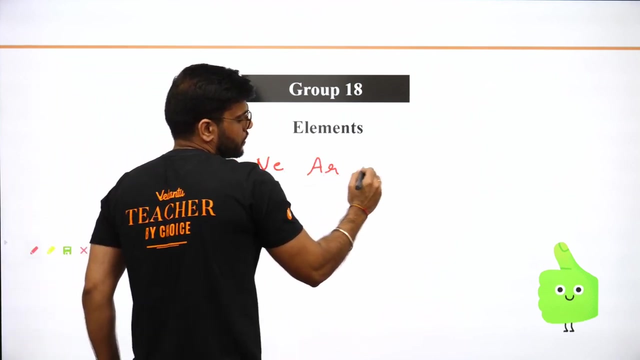 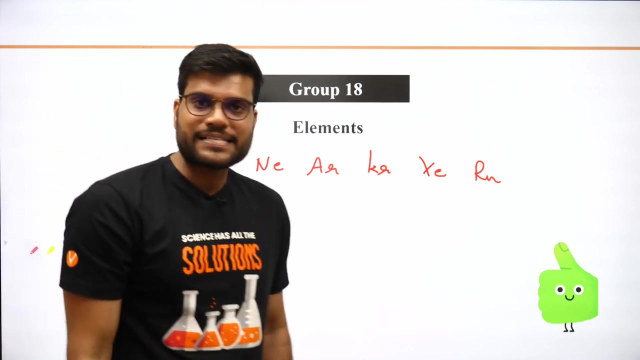 First of all, Helium, Neon, Neon, Carbon, näch adjustment a algumas erg, Sofia On on medur Radon. This is it. Yes, So We have this element. Now see in this. It's fun We are going. This is from top to bottom. I have written it like this: 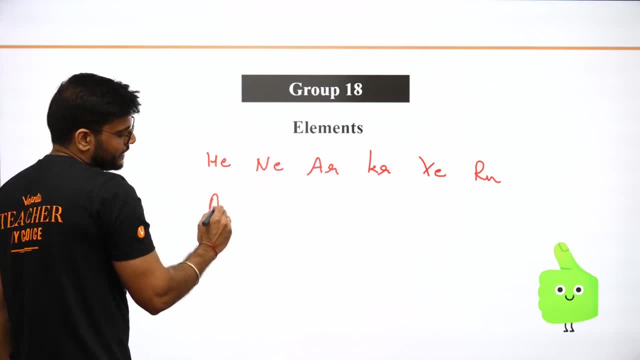 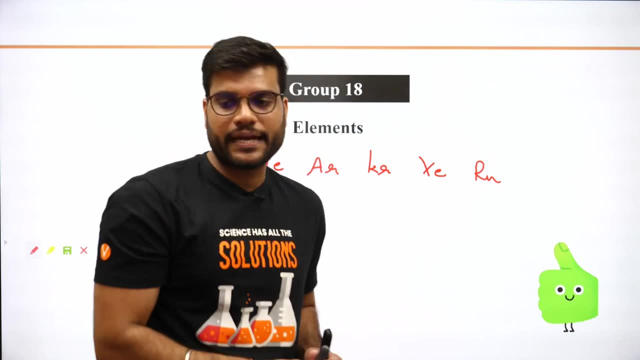 But this is top to bottom. So from top to bottom. First of all, Let's talk about atomic radius. Atomic radius, What difference does it make? Atomic radius? Who is the smallest Helium? Okay, So atomic radius From top to bottom. You guys write From Top to bottom, Okay. 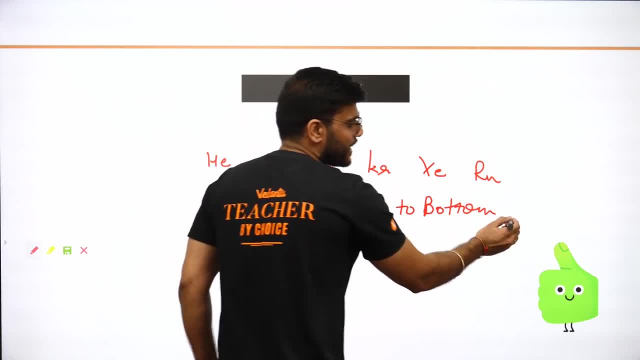 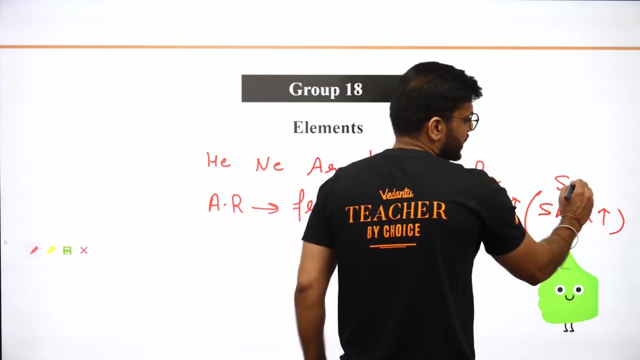 From top to bottom. What is atomic radius Increase. So everyone knows It's very easy. It's very easy, Yes. Now why is it increased? What reason will you give? This is the reason: Due to increase in shell. Shell increases, My dear children, Shell increases. You can say Screening effect increases. 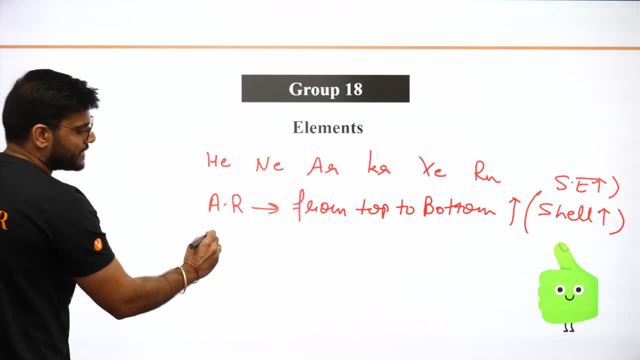 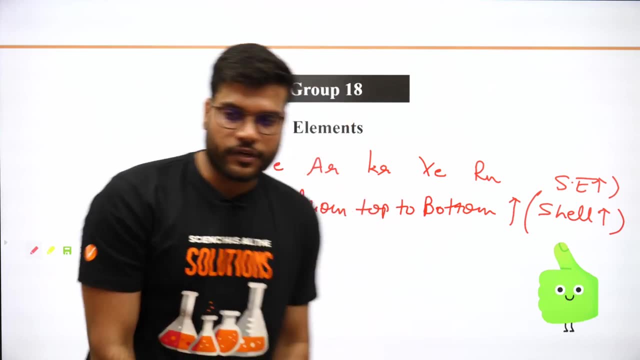 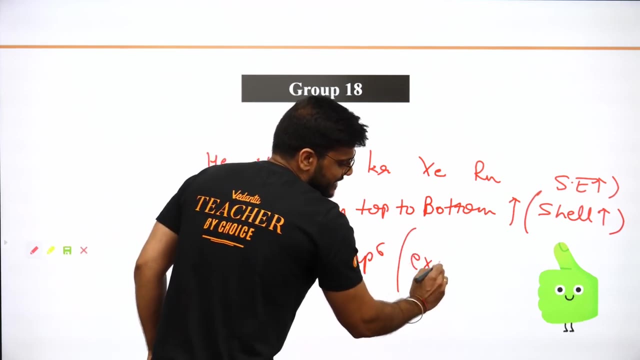 These things are very common. Second thing About this: You can write Electronic configuration, Their generalized Electronic configuration. GEC Generalized Electronic configuration. So their generalized Electronic configuration. What is GEC, NS2, NP6 Except Helium? Write it Except Helium. If we leave Helium, Then what happens to the rest? 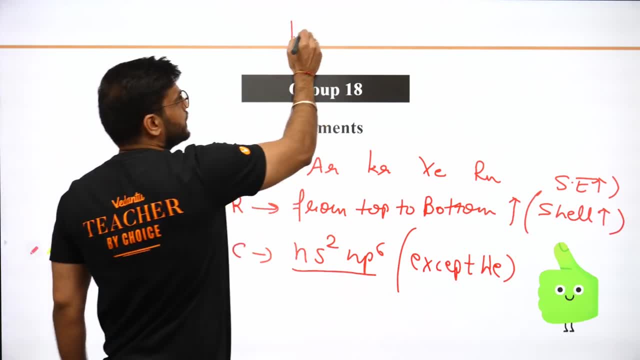 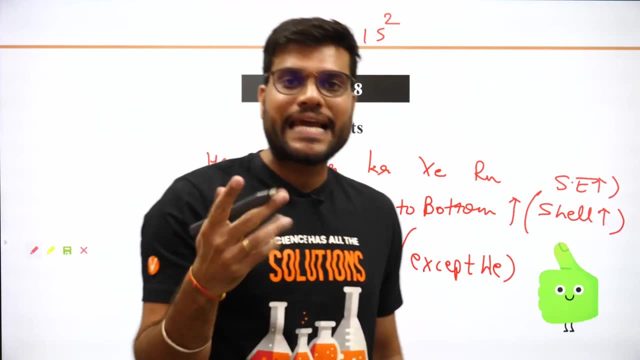 NS2 NP6. This is generalized Electronic configuration. Helium has 1S2. Okay, So we know this. It is an inert gas. It should be in it, But its properties Matches with inert. That's why it is kept Here. Everyone understood It's so easy Clear. 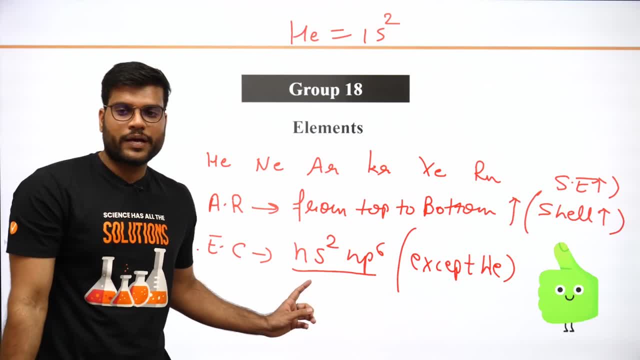 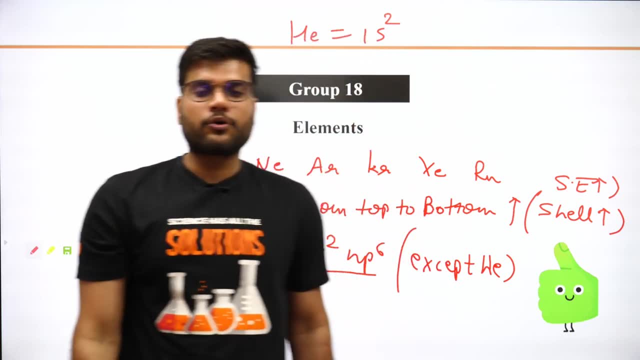 So here you check: Generalized electronic Configuration: NS2, NP6 And Helium. It is valid with everyone, It is clear to everyone. So here Another property We understand, Which is very important. That's really brilliant. Now I will tell you A very important thing. This was a common thing. 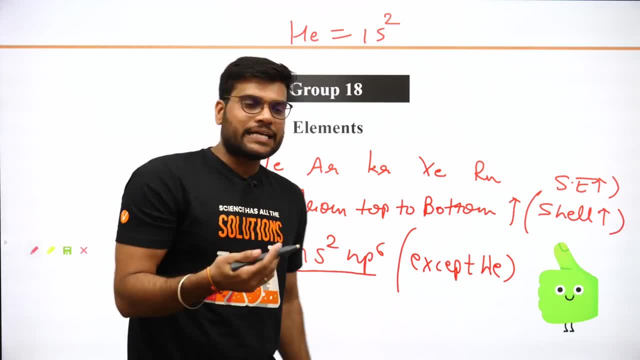 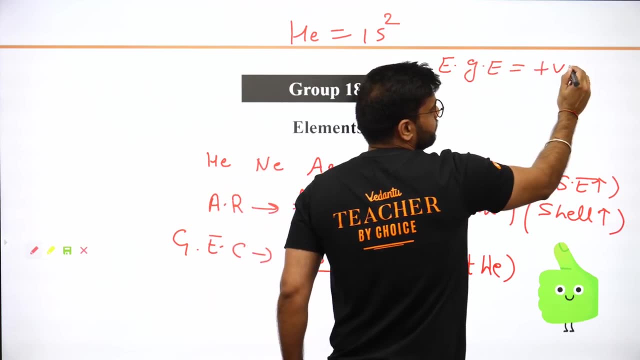 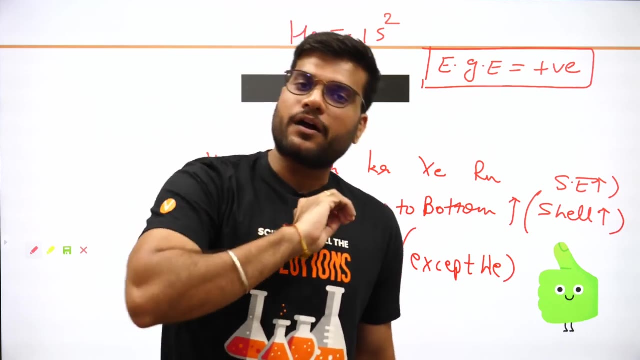 Which you know, If we talk about Here, Their Electron gain Enthalpy, Their electron Gain Enthalpy In the entire periodic table Is the most positive. In fact It is positive. You write it. It will be useful For noble gas, Electron gain enthalpy, Enthalpy. 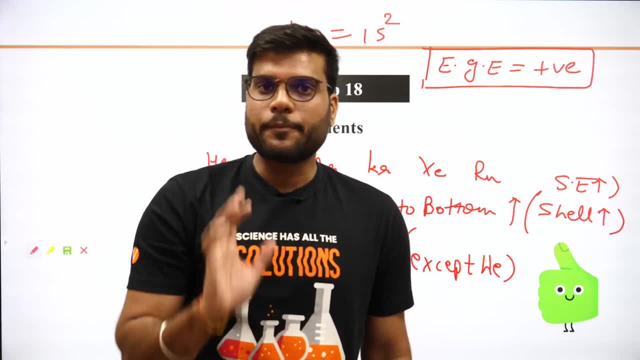 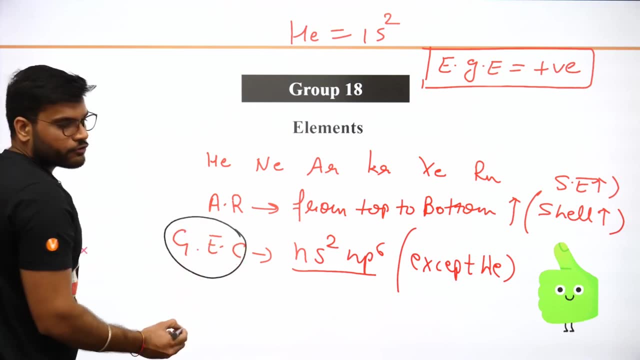 Always positive. In fact, It is positive. Now why Electron gain enthalpy? Why? Because All of these. How are You look carefully? Electronic configuration: It is fully filled. What is it Fully filled? You just check: It is fully filled. Ok, Now it is fully filled, So they have no need. 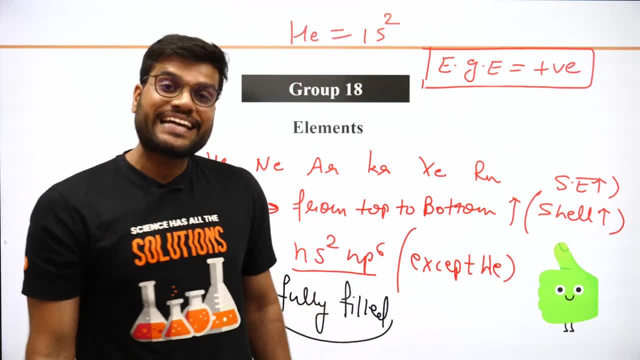 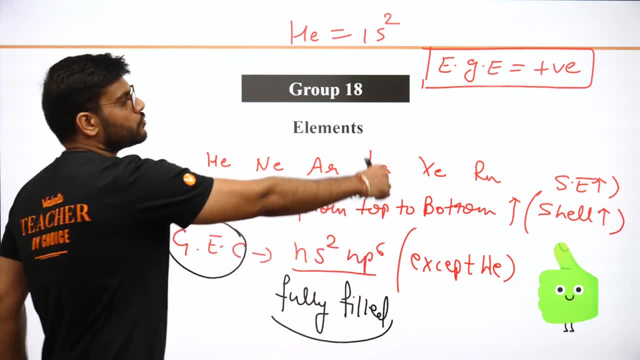 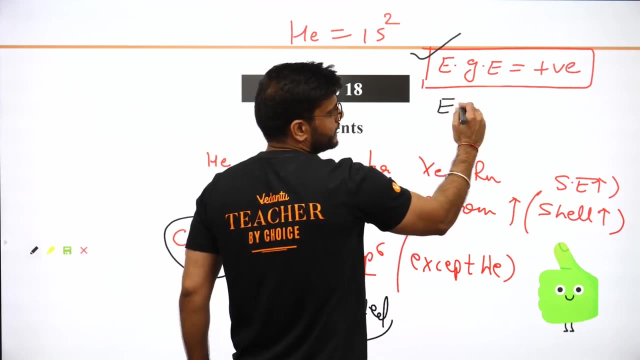 Of electrons. Ok, In this case They take a lot of Amount of energy If you have to give them Electron. So here Their Electron Gain Enthalpy Is positive. This is a very important concept. If we talk about Electronegativity Along with size, Then There is no exception. 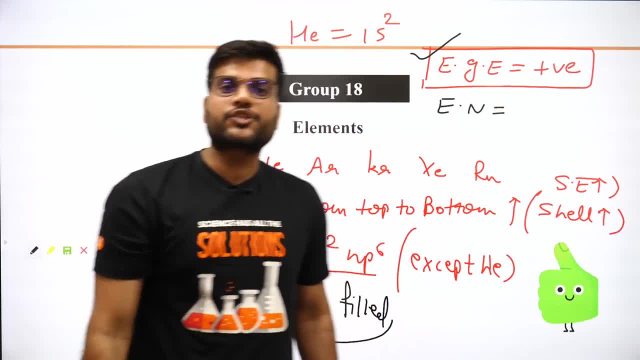 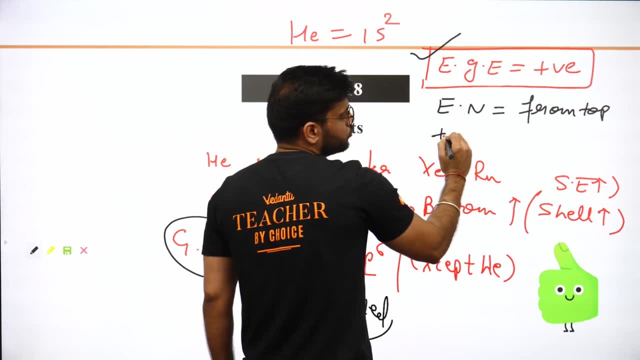 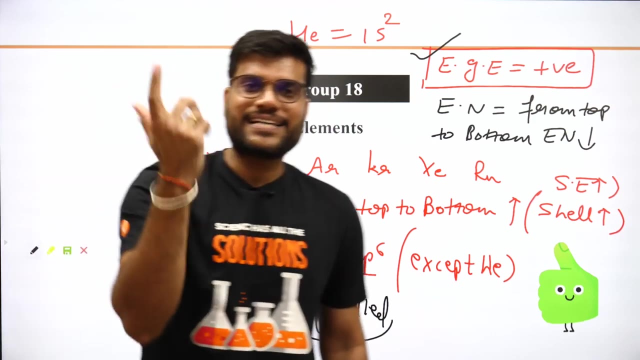 In this: If you go from top to bottom, Then Electronegativity Starts to decrease. So You also write this: From Top To Bottom. From Top To Bottom, Ok, Electronegativity Decreases, And anyway, They don't need Electronegativity. So now There are some things. 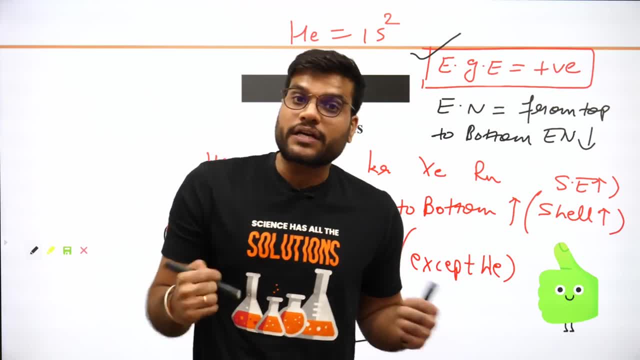 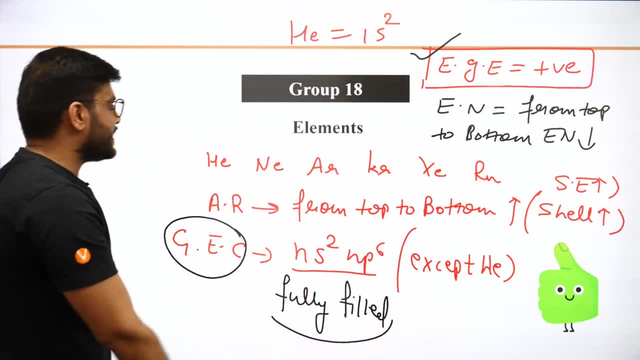 Now, These are inert gases. These inert gases Won't react. If they don't react, Then what are we reading? Why are we reading? It's not like this. Some of these gases Are like this, Which also react And also make Compounds In which The most important Name is: 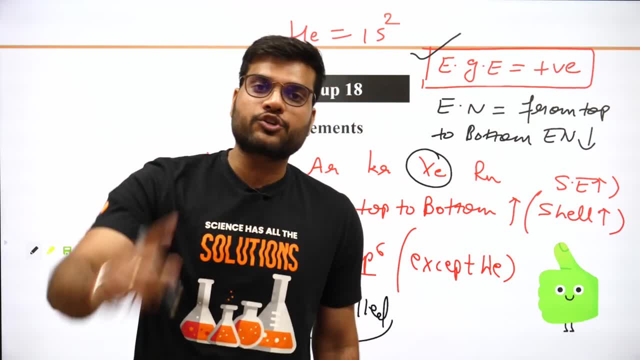 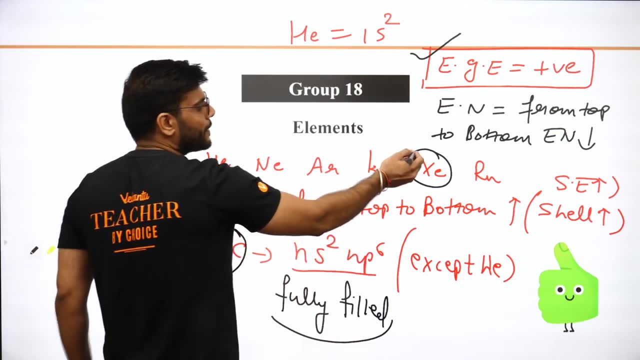 Xenon: We have to read About it. There are questions On their compounds. I will tell you How to remember Their chemical reaction- Everyone understands. So what are we going to read? What are we going to read? Xenon's Compounds, Which we are gonna read. Compounds. 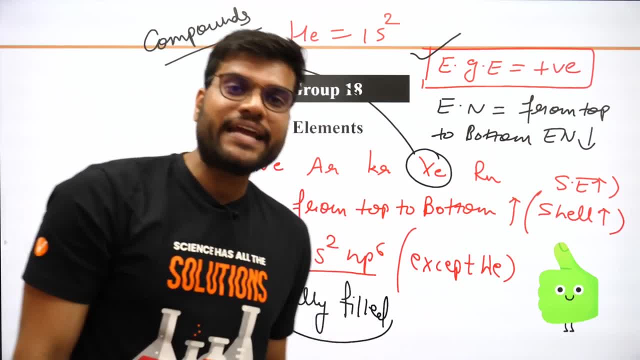 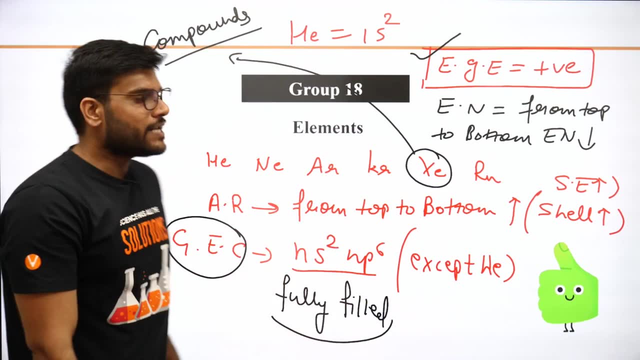 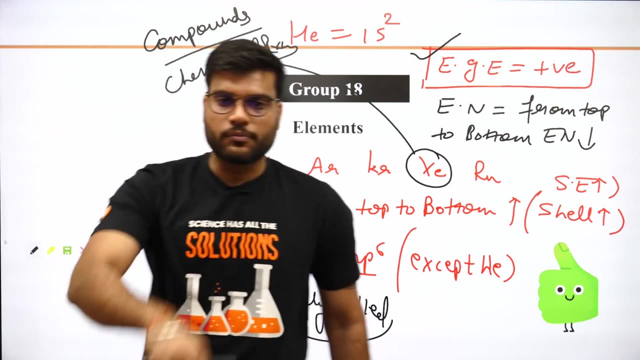 Which we are gonna read From Xenon. Now this is really Very important. Ok, And These compounds Will be read With their chemical reactions. It becomes clear To everyone. Will be read Their chemical reactions. So are you Guys Ready, Tell me Their chemical reactions And so on. Are you guys ready? 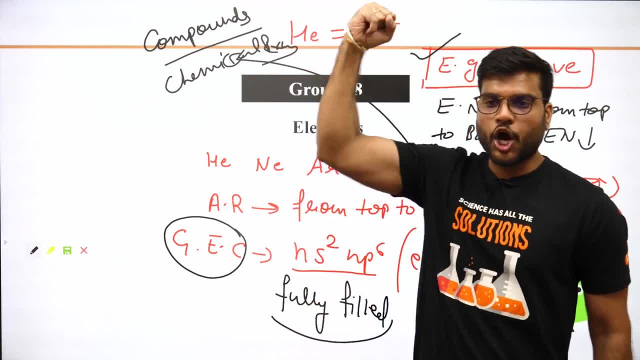 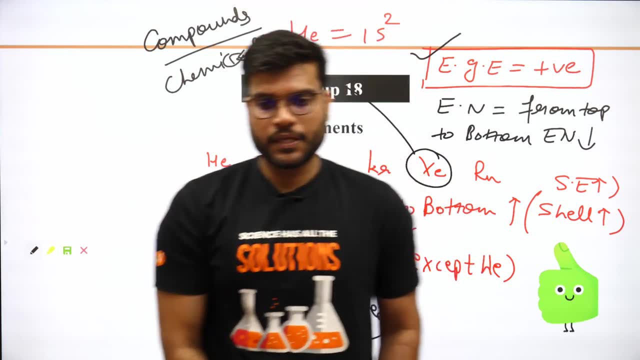 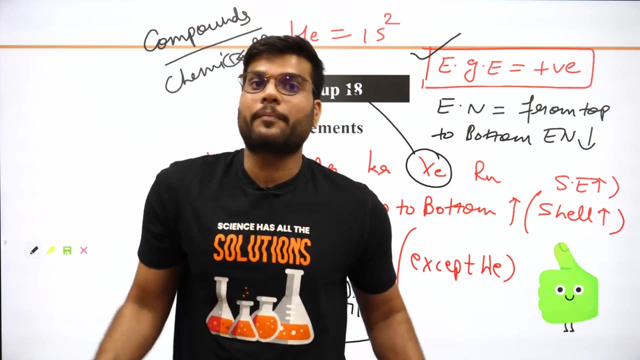 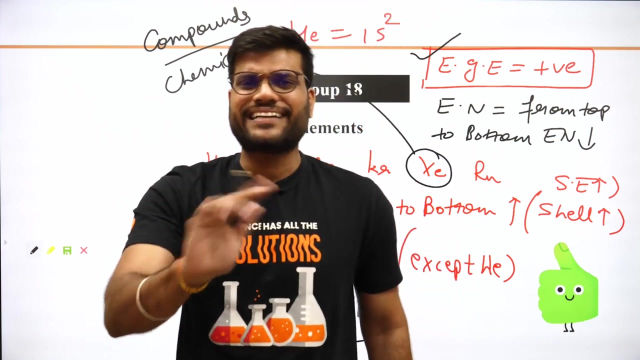 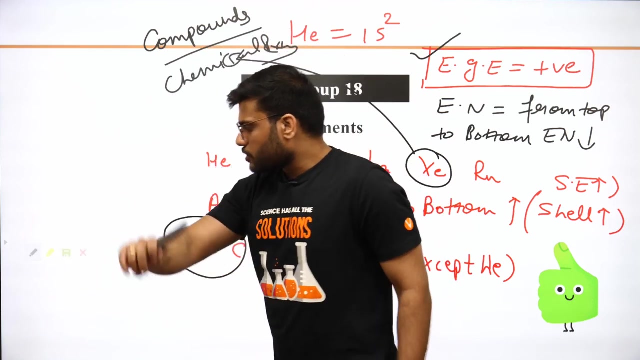 Are you guys ready? Are you guys ready? How is our enthusiasm mais, Obviously, How's the joy? Well done, my dear children. Very good, That's really awesome, That's really brilliant. Now let's go ahead. I am saying again and again about a very important property that I am going to tell you. I am going to tell you, I am going to tell you Now, I will tell you finally- And there is a question on it- Neat almost 2008.. It is a question of 2008.. It is a question of 7 or 8.. The question has been asked in the medical exam And you guys understand very well. You guys look carefully. These were small properties. 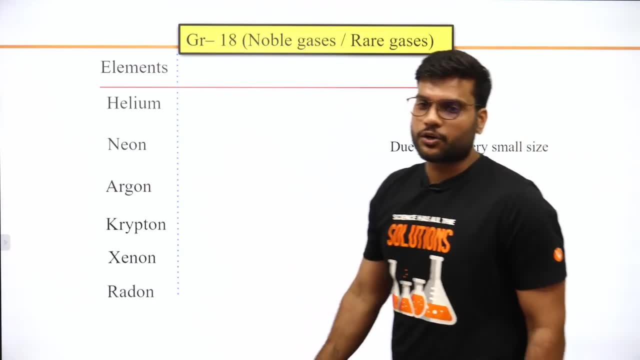 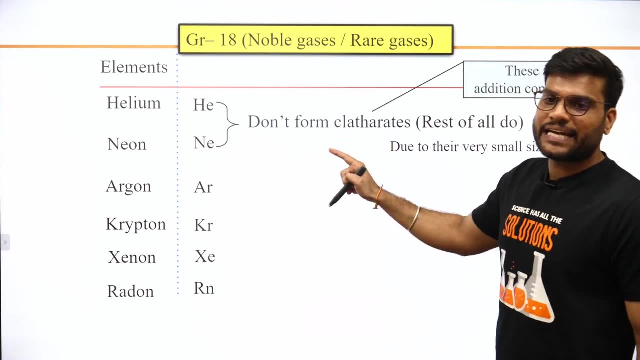 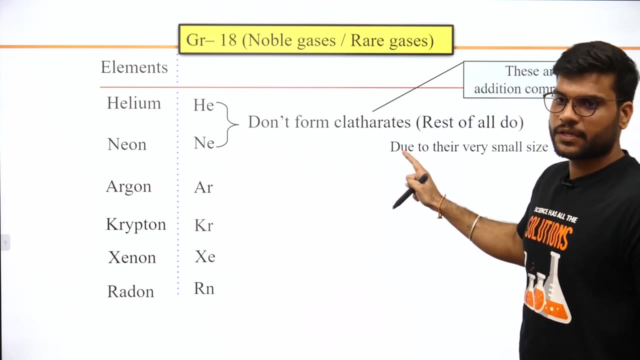 Now I am telling you a very important property about them. Check it out. These are the gases And there is a property in it. Their symbolic representation is this: Everyone knows Now there is a property here, Write it. Helium and neon don't form clathrates. Rest of them make clathrates. This is a very important property, children. 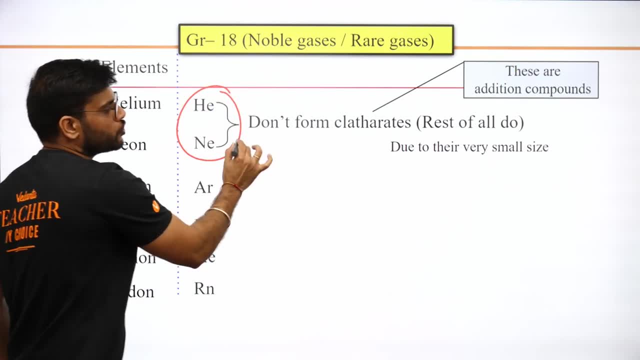 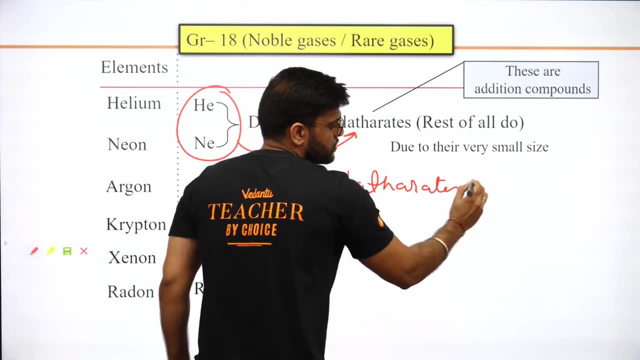 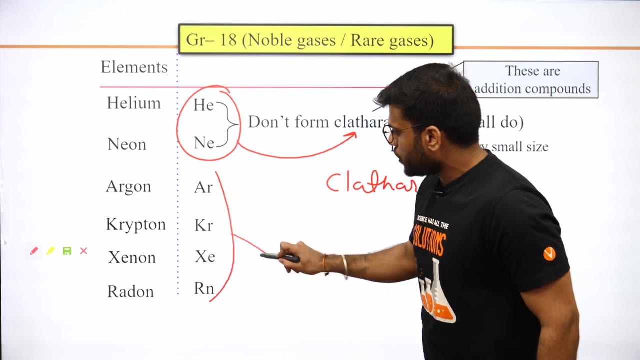 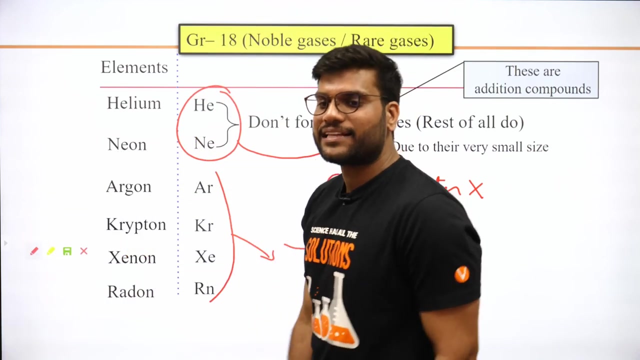 Helium and neon don't make clathrates. Ok, These two don't make clathrates. Rest of the gases are made of organs, cryptons, xenones. All of them make clathrates. Now the question is: what is the meaning of clathrates, In which the most property of clathrates is seen in xenone? 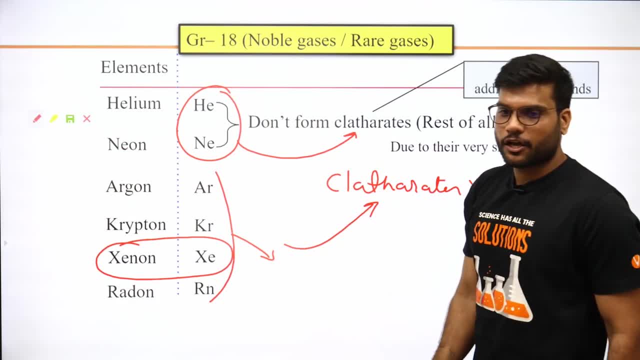 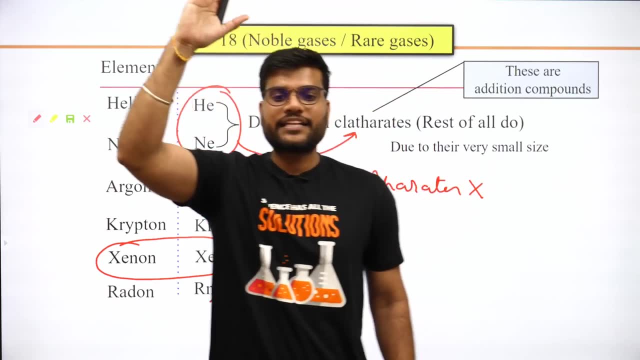 ok, so we have learned that this is a common feature in a product, so i will clear this. now the question is: what are clathrates and who is the one who will tell in the chat section about clathrates and what is the meaning of clathrates? 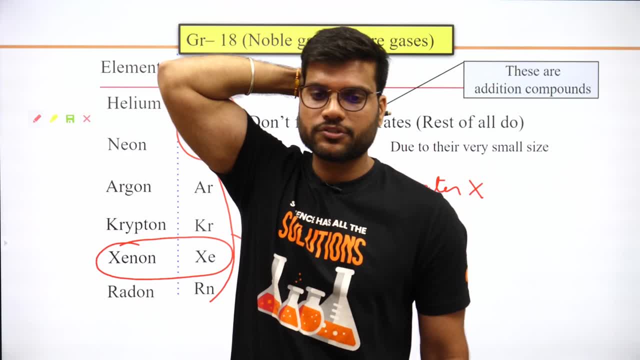 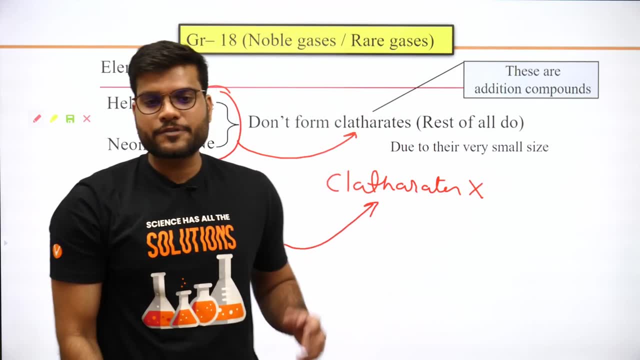 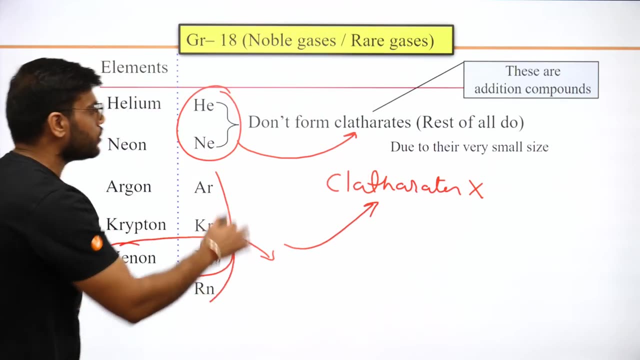 can you answer this question? what is the meaning of clathrate? can you answer this question? can you answer this question, guys? Ayesha is asking: what is clethrate? I am only asking you. I will answer you. But look, the first thing is that Helium and Neon don't make clethrate. 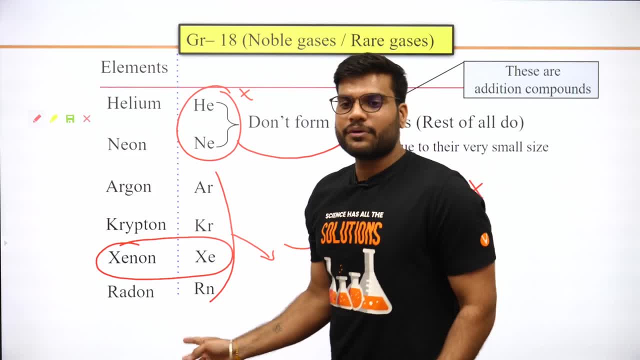 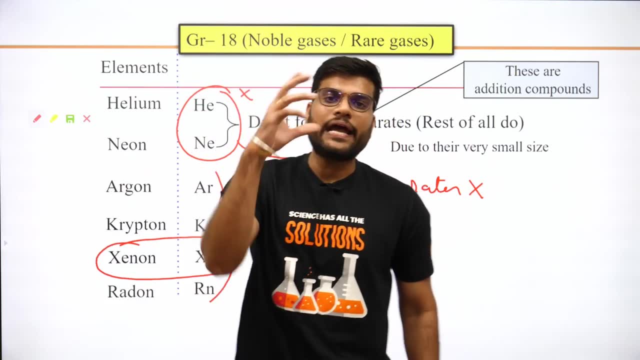 Apart from that, all these clethrates are made, The number of xenon is the highest among them. Now the question is: what is clethrate? What is clethrate? So what is clethrate? Look, let me tell you in a simple way. 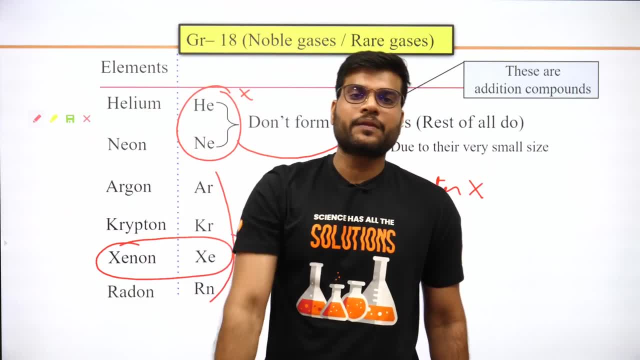 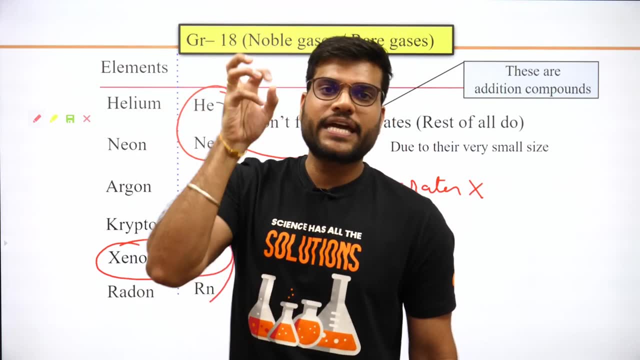 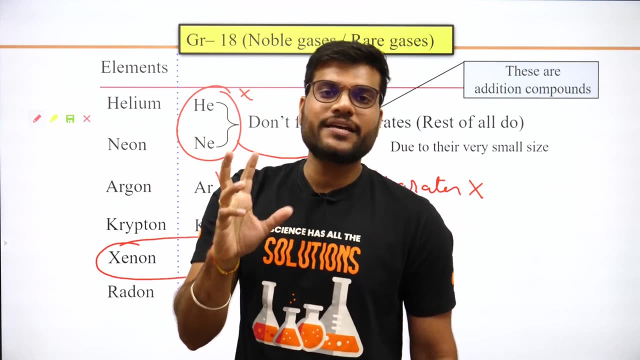 Have you ever seen a bird in a cage? Have you seen or not? Have you seen a bird in a cage? Have you seen a bird in a cage? So, actually, there is space inside the cage in which the bird is. Similarly, there is space in a crystal and these Helium gases enter it. 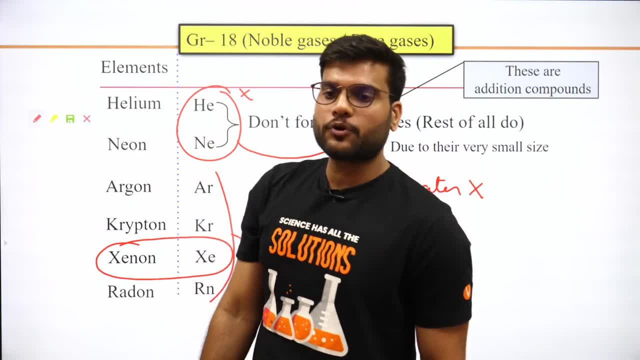 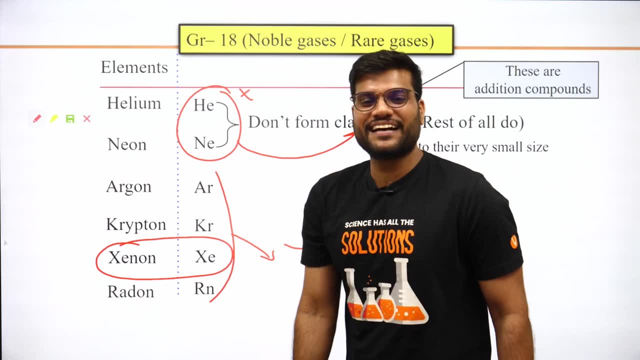 We call it clethrate. So I am telling you the definition of clethrate. Check it carefully. So it is very important. Somebody is saying, hey, Google, what is clethrate? So what does clethrate actually mean? 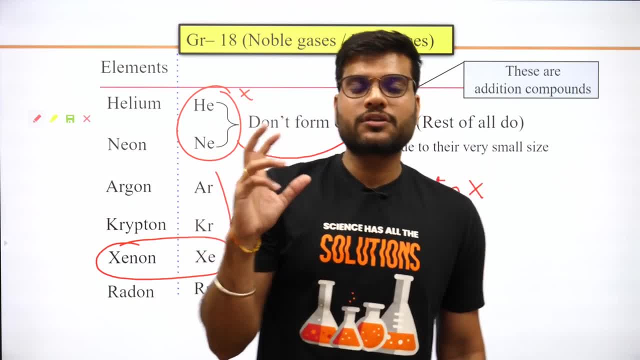 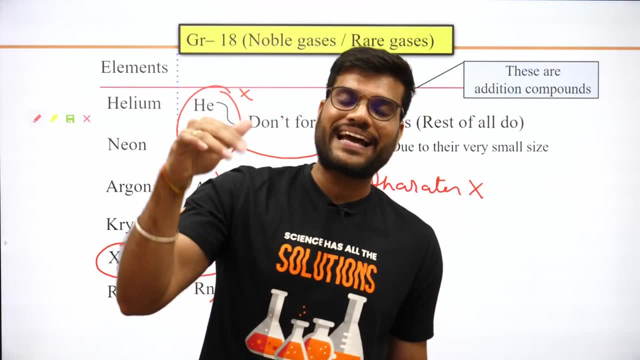 You must have seen a bird in a cage. So there is a space And in that cage actually there is a bird. if there is space, Similarly in a crystal, the noble gases enter the space. We call it clethrate. 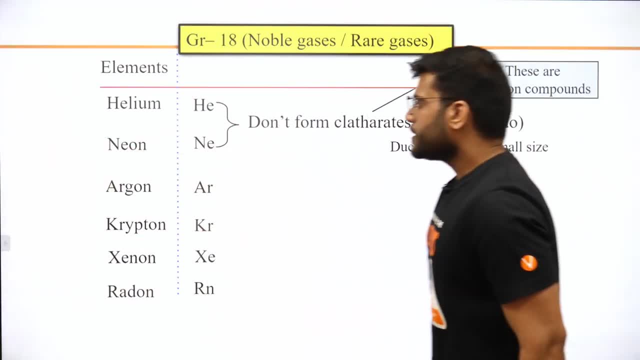 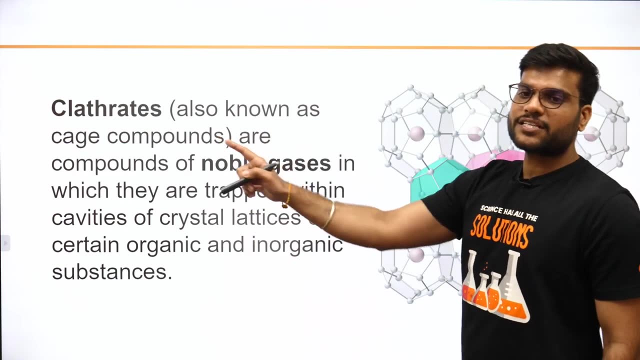 Now let me explain you a little better pictorially. Here you check it. This statement is very important. Now, what is clethrate? This is written in front of you, Just check it. Clethrates means cage compounds. 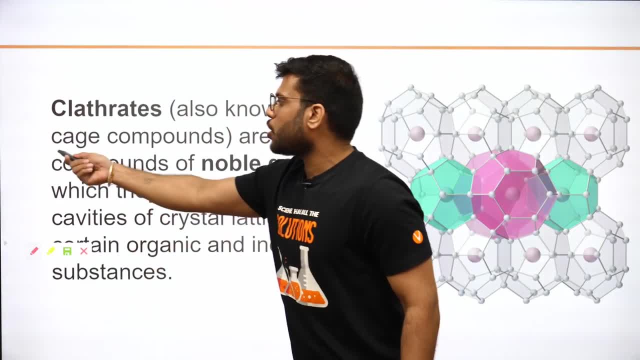 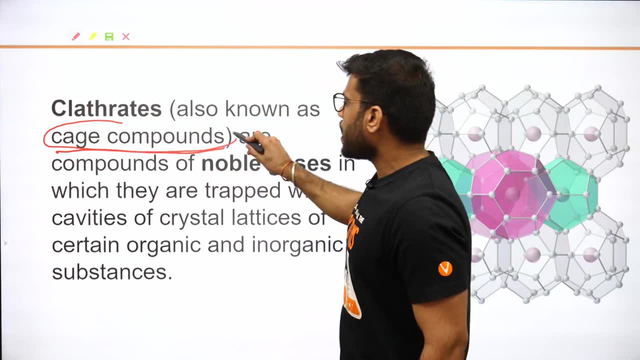 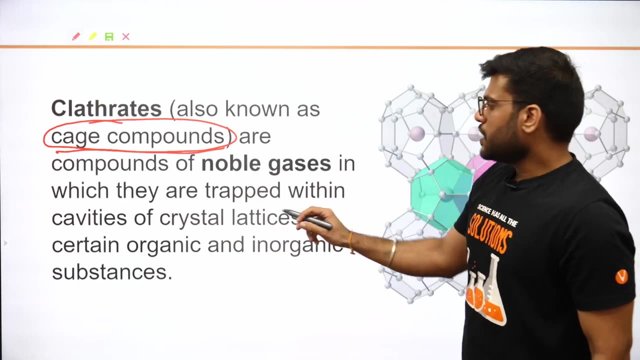 Means compounds like a cage. See this: Clethrates means cage compounds, Means compounds like a cage. Just check it, Is it clear? Compounds like a cage, Compounds of noble gases. These are compounds of noble gases, So the word clethrate. 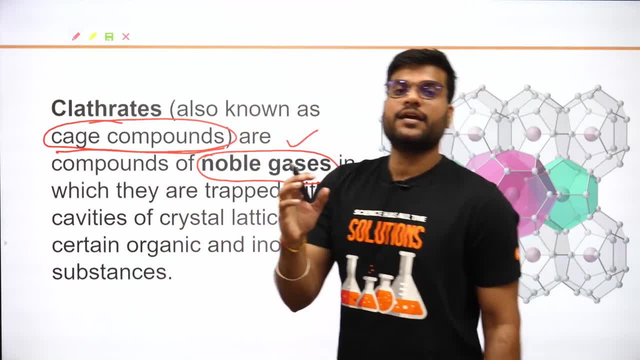 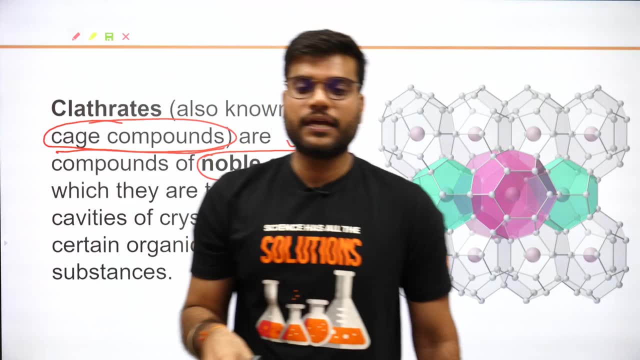 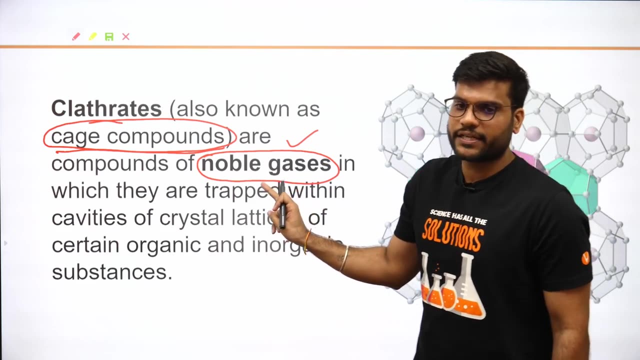 This word is specially associated with whom? With noble gases. So first of all write clethrate In the chat section. clethrate means cage compound. This word is directly associated with noble gases. It is associated with noble gases. 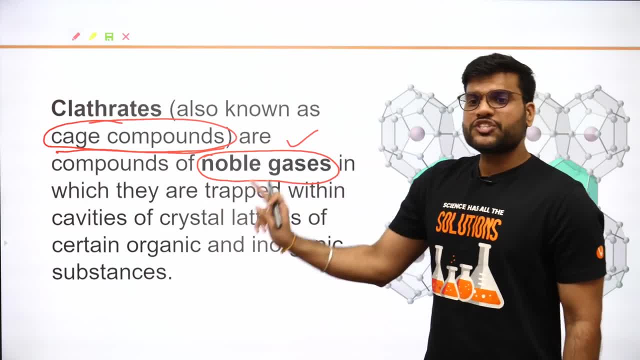 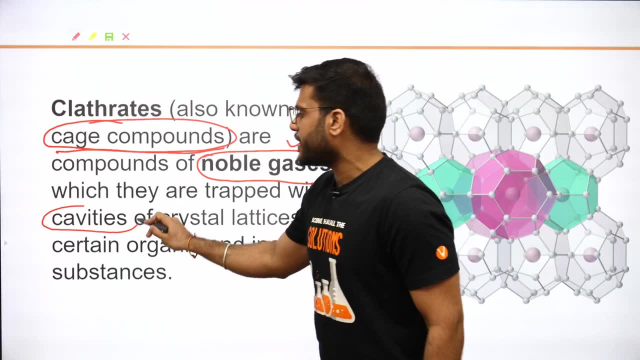 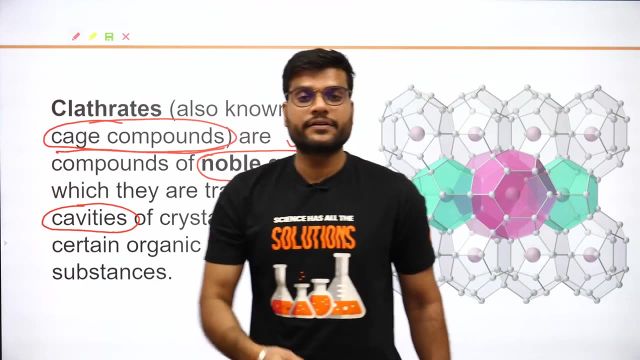 Write it Okay- In which they are trapped within cavities of crystal lattices. Now, what are cavities? Food gets stuck in your teeth. No, There is space in your teeth, Okay, And food gets stuck in it. 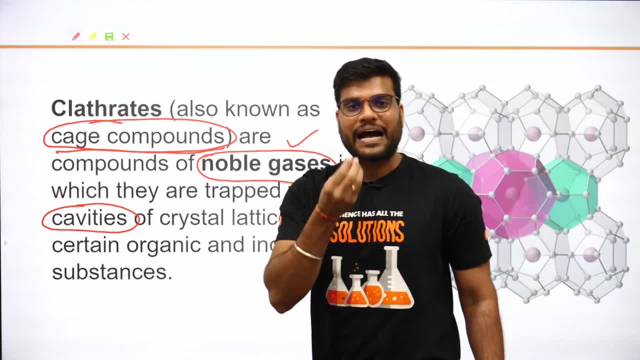 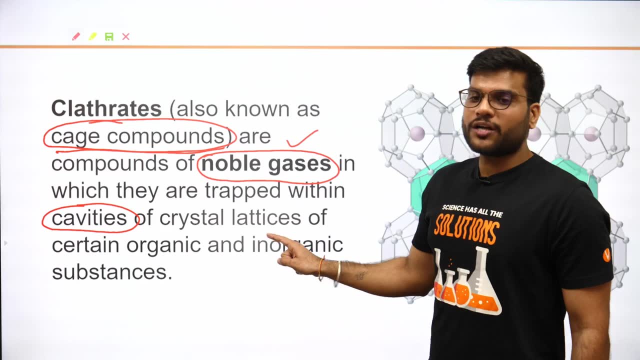 Yes, So it is the same condition. It is the same thing here. When you eat food, food gets stuck in your teeth. That is what we call it In the cavities of crystal lattice. There are many certain lattices in organic and inorganic. 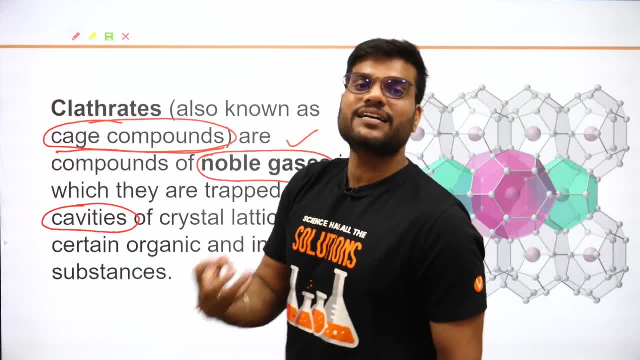 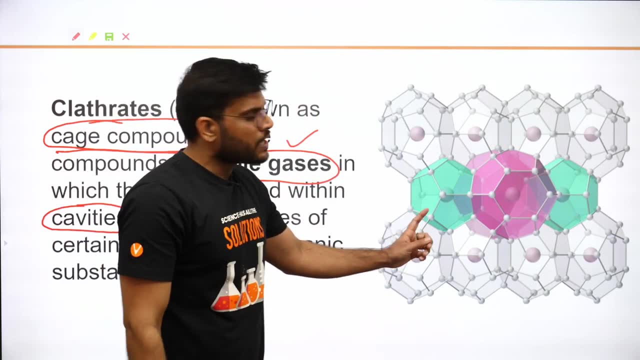 There noble gases get trapped. They get stuck, Like your food gets stuck in your teeth, Like here. you see, This is crystal And in crystal noble gases are trapped, They are stuck. What do we call them? They are called clathrates. 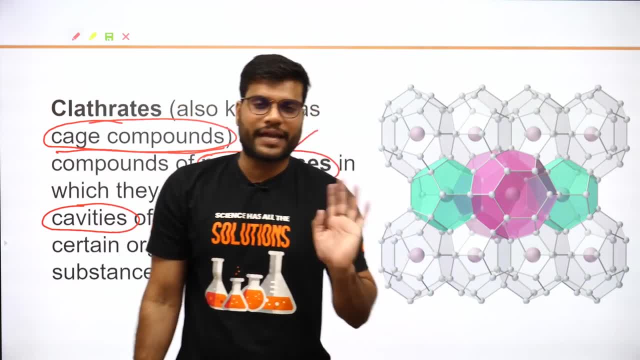 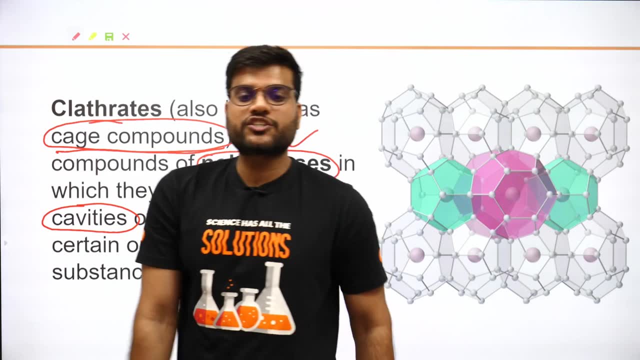 So today, two minutes ago, we didn't know, But now we know what clathrate is. After today, you won't be scared. What is clathrate? It is not Katrina Kaif. Katrina Kaif, Don't change the name. 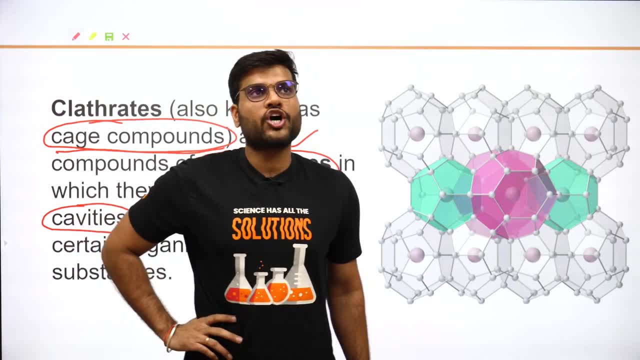 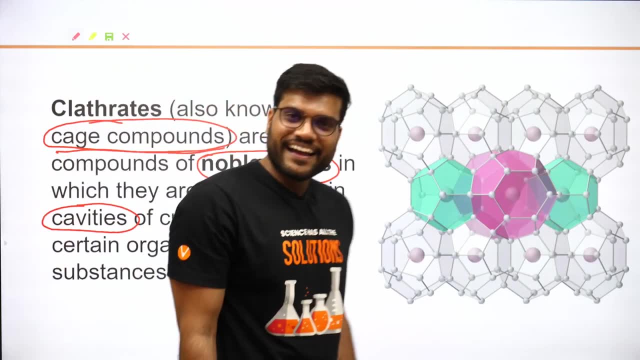 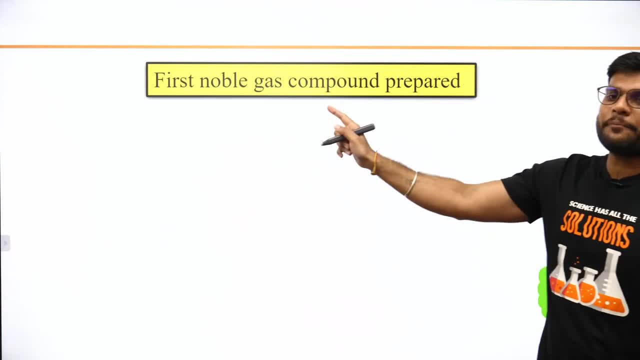 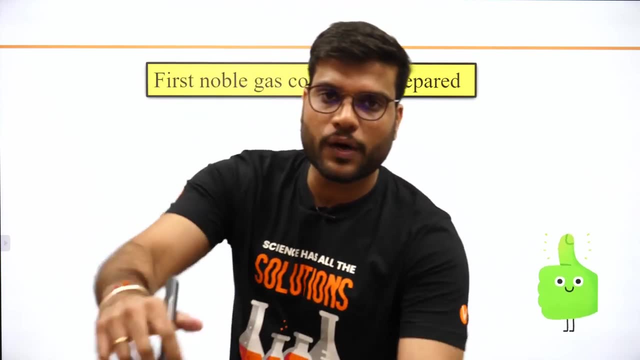 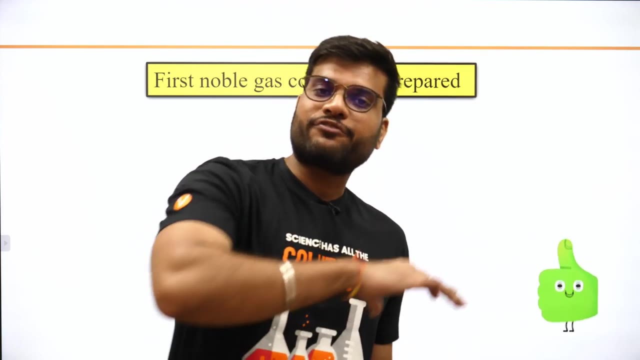 Katrina, Katrina. Now we will check here that how the first noble gas compound was prepared. How was the first noble gas compound prepared? You will know its history, you will enjoy it And then after that we will move towards xenon. And today, chapter 1st is not phantom. 1st is finished. 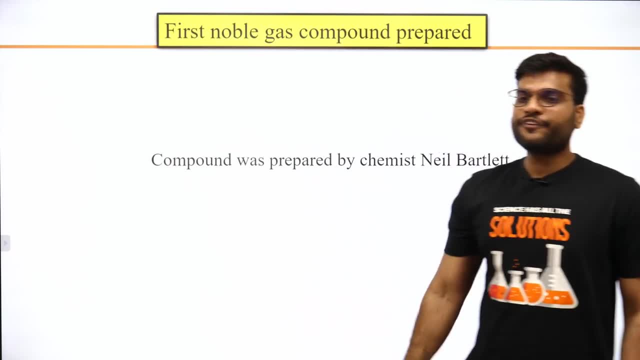 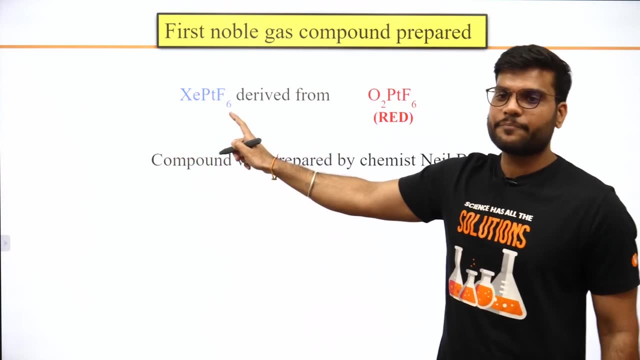 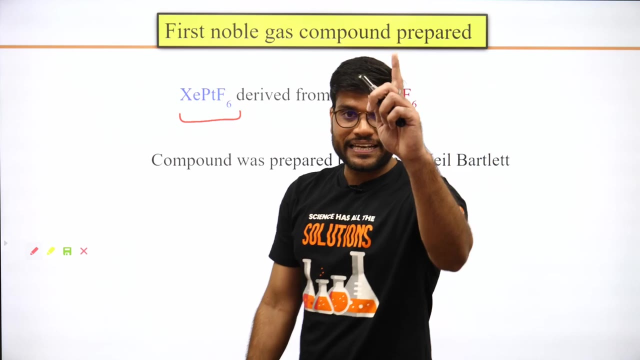 So let's see the first noble gas. Now check how the first noble gas compound was prepared. Actually, the first noble gas compound was prepared. Just check: the first noble gas compound was this one: XZPTF6. This was the first compound of noble gas. 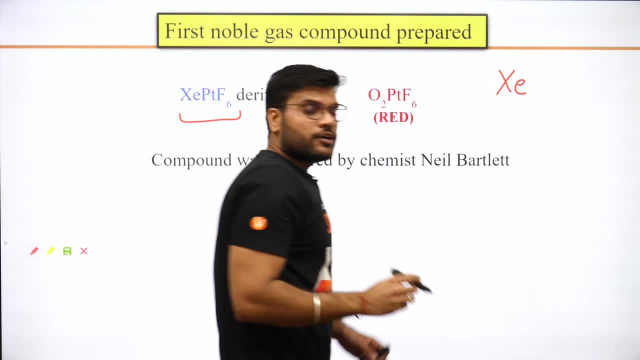 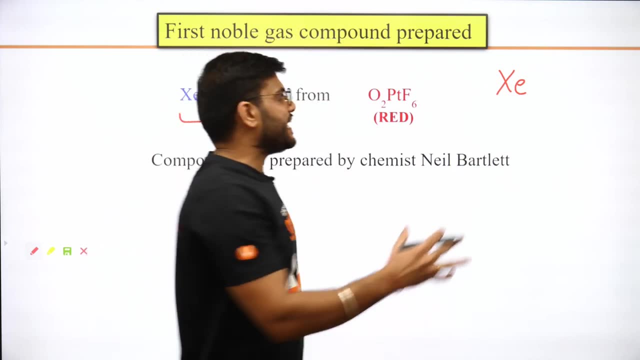 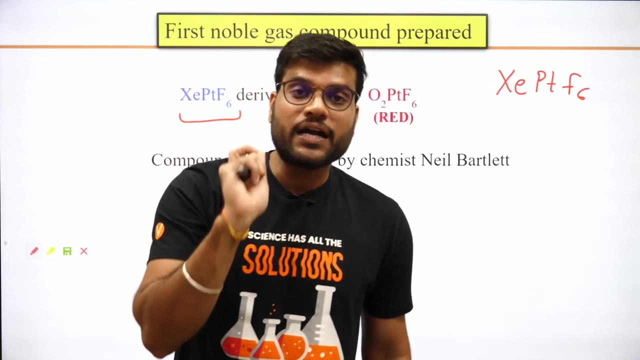 Many times there is a problem that. does noble gas make compound? Yes, it does. Which was the first compound found? XZPTF6. You remember, XZPTF6 was the first compound which was found. What was the first compound of noble gas? 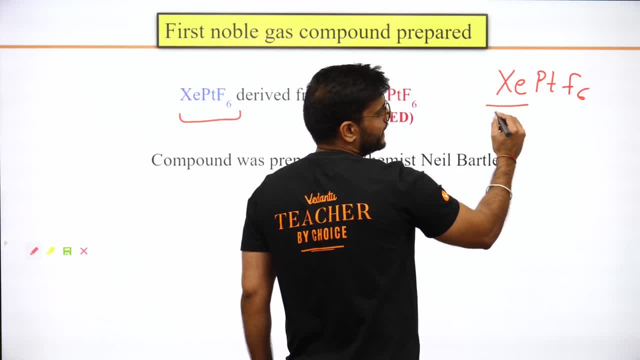 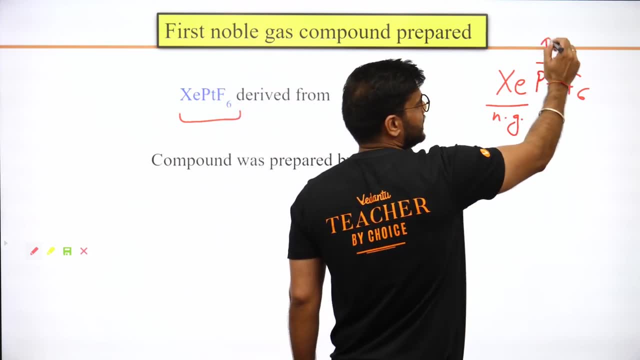 Who are they? Just check, Here is xenon. this is inert gas. NG means inert gas, noble gas. What is PT Platinum? that's a metal, Fluorine. just check Fluorine, look at it. 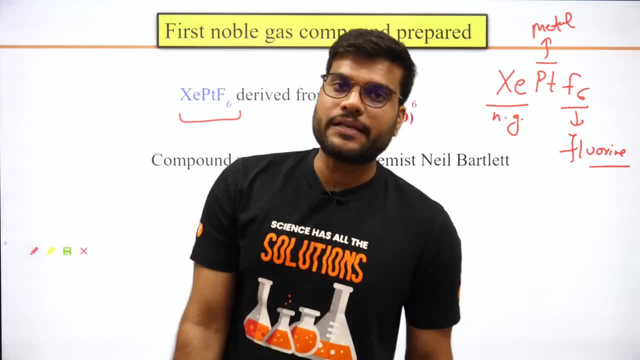 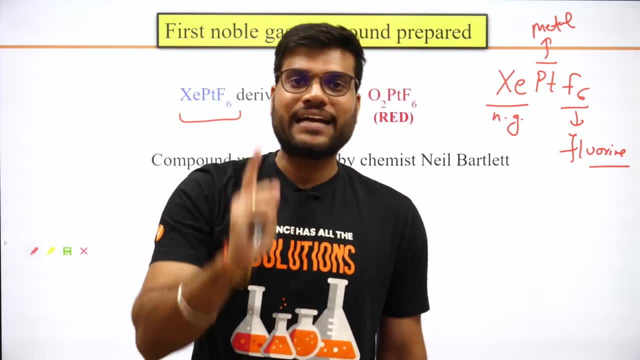 We have this XZPTF6, simple. This is the first compound which was made by whom. I will tell you this. This question has been asked. note down First: noble gas compound. What is this compound? This question has come with 4 numbers. 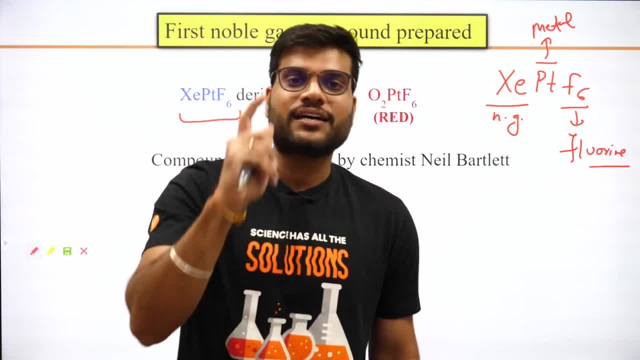 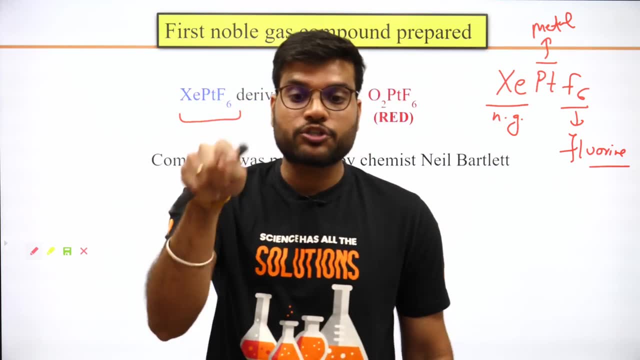 Now it is your choice whether to remember this or not. Now tell me. you guys See how few kids are interested. Swapnil has written this compound in the chat section. Har Simran has written it. Neha Tiwari has written it. 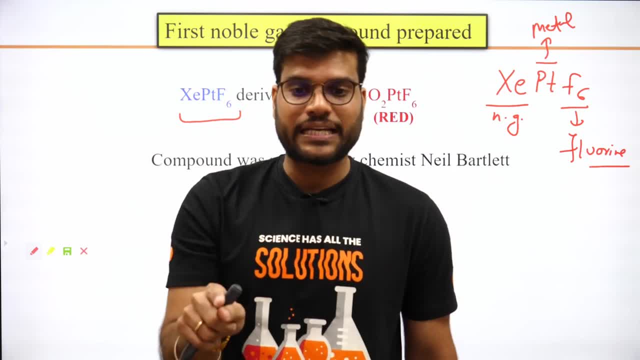 Son, until you guys don't write it, it won't be fun. Abhishek has written it. See, very good, You write it. Dr Rajesh Roshan has written it. Rithik Roshan's movie is coming. 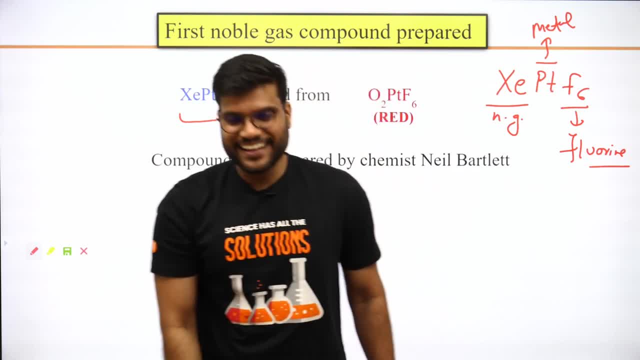 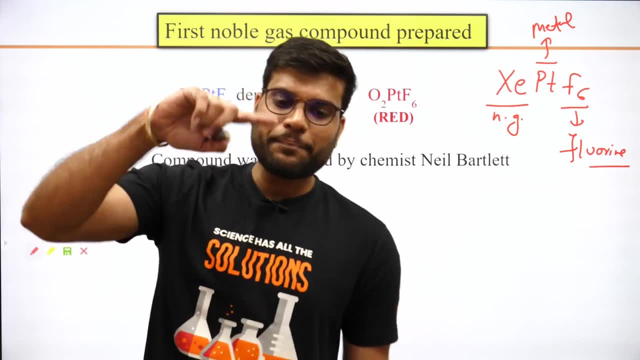 Wow, His father is educated here. Write it. Until you don't write it, it won't be fun. Write it down right now. Which was the first compound? XZPTF6.. This was the first compound And this is a very important question. 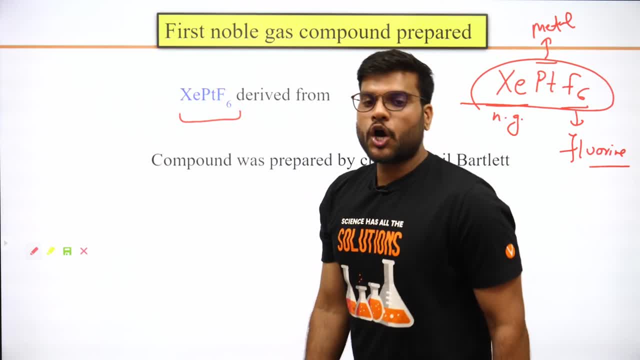 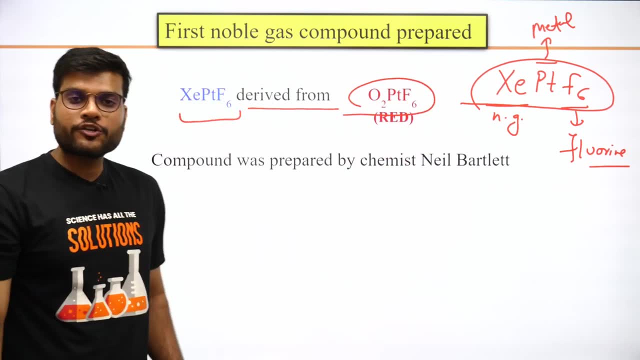 This is the first compound. Now the question is: from whom was it made? And actually this compound was made. Please check: XZPTF6 was derived from O2PTF6.. It was derived from O2PTF6.. 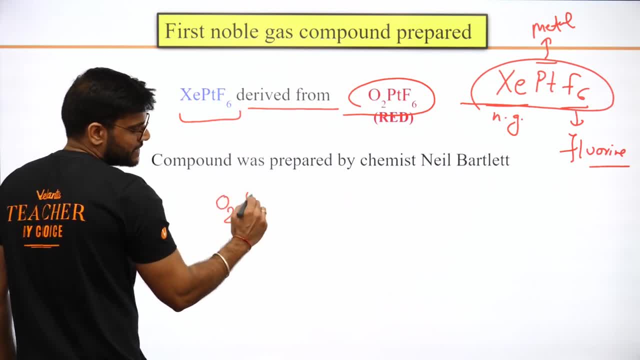 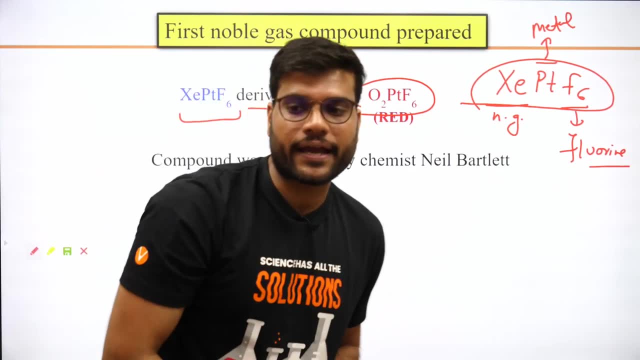 Meaning O2 means there was oxygen in it Along with Pt, And along with it was 6 molecules of fluorine, O2PTF6.. It was derived from this Meaning O2PTF6, and XZ gives you XZPTF6. 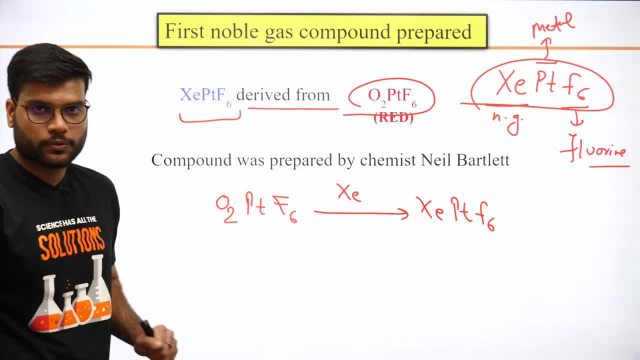 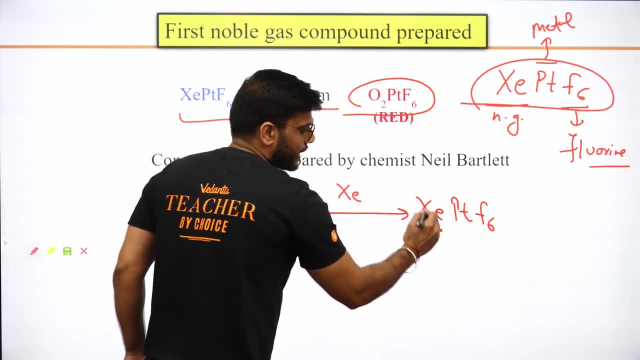 Okay, XZPTF6 gives you Now. look carefully, Actually. how did this happen? You check, Only O2 has been removed from here And XZ has been applied. Is it clear? O2 means oxygen has been removed. 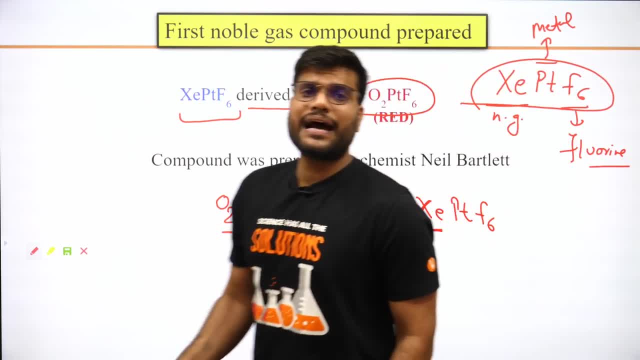 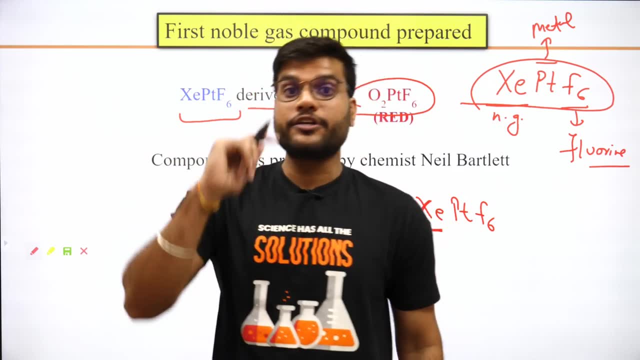 And here Nobel gas has been applied. Why did this happen, That here O2 gas has been removed And Nobel Xenon gas has been applied? What was the reason? This question has been asked many times Earlier. you know, there were interviews. 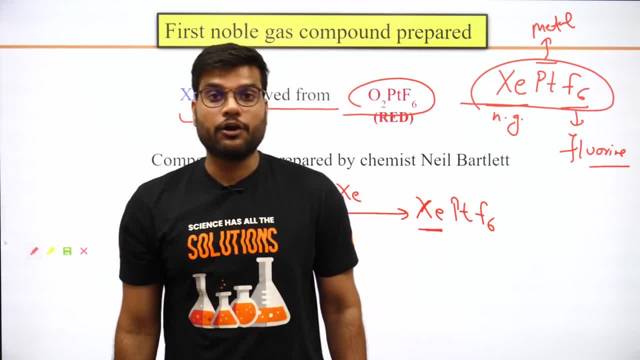 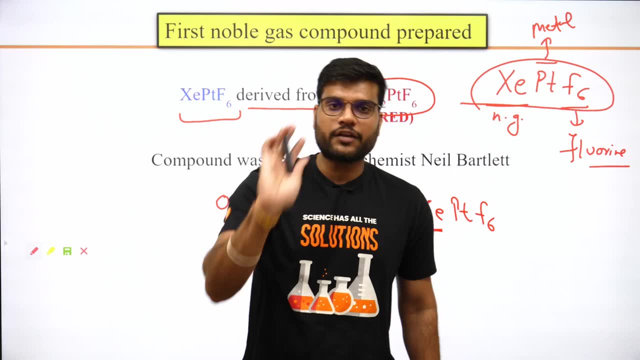 15 years ago to go to IIT. This question has been asked many times in those interviews And maybe it is possible that you have interviews in the good colleges for admission, But nowadays it has stopped Because the children do not have the courage to give the exam. 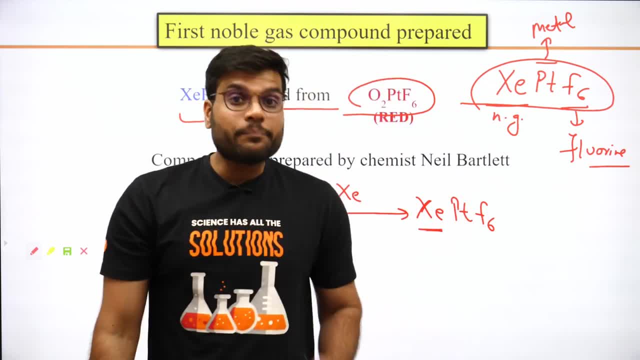 Interview is far away. There is no patience, But earlier there were interviews And a question was asked in them. Now the question is that here O2PTF6 has been reacted by XZ. XZPTF6 has been found. 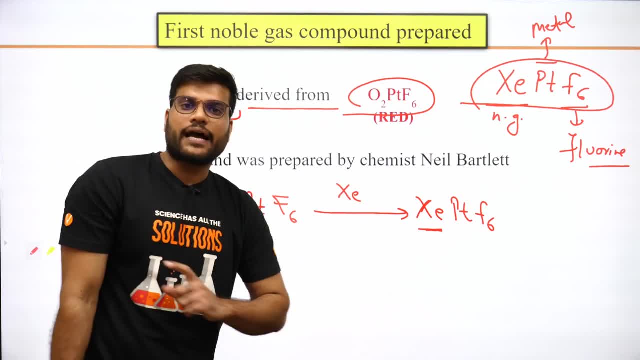 O2 has been removed. The question is: why did this happen? So I am going to give you its answer. So come on, check carefully. Look here: Compound was prepared by this chemist, Neil Barlet. Neil Barlet. 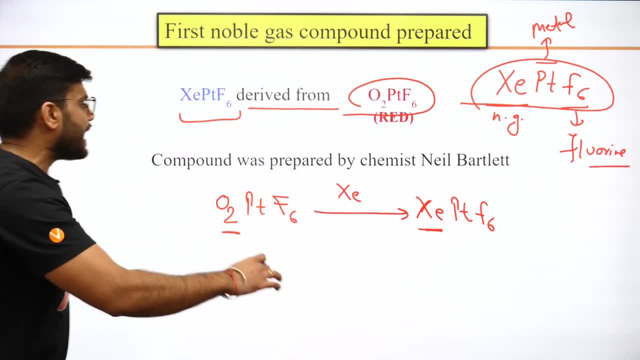 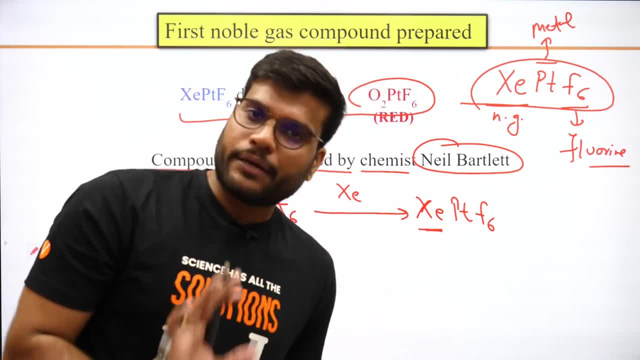 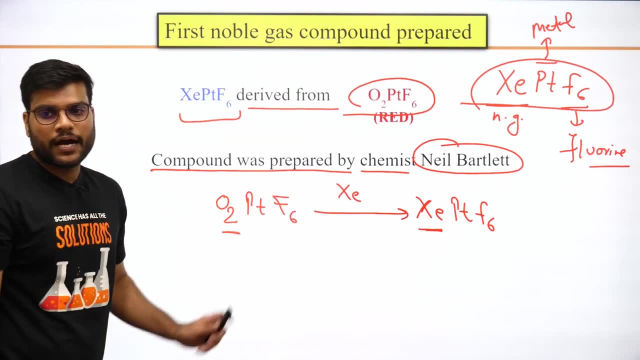 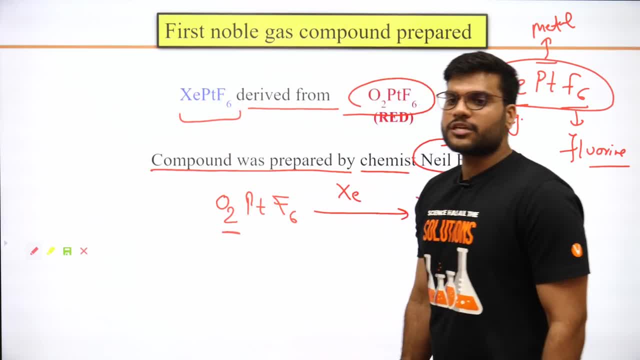 So, Neil Barlet, It was this chemist who had made this compound. Did everybody understand? So now let's go ahead. Now look here: the question is that, from here, O2 was replaced by XZ. But why is this? 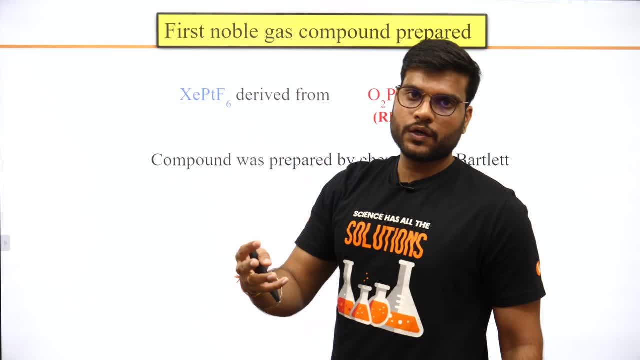 What is this difference in both? So it is asked, so you can check. Actually, check here: O2PTF6, it was decomposed. So after decomposing, O2PTF6 is decomposed. Again, it was decomposed. 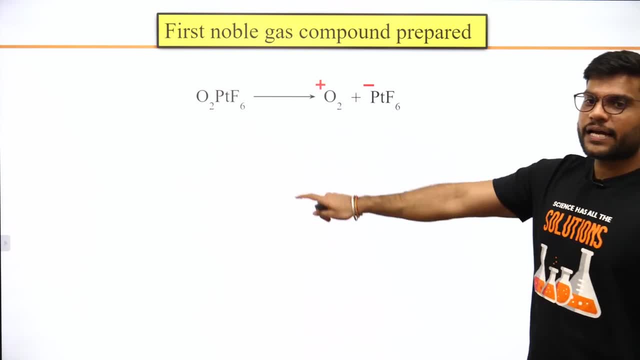 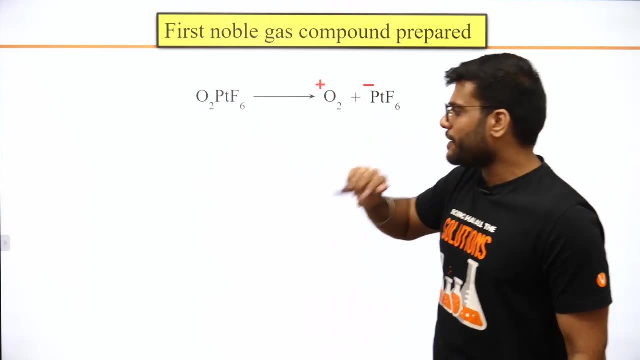 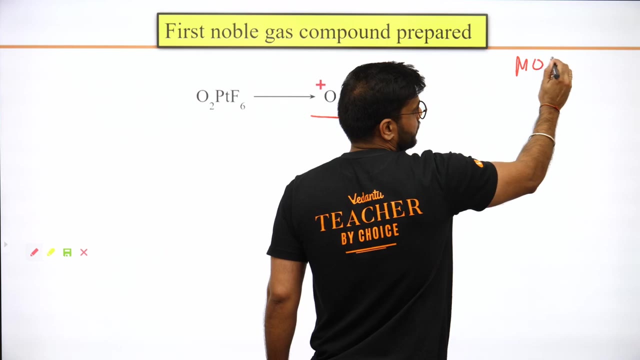 Why was this? Actually? I am checking here: O2PtF6 decomposes and gives O2 plus and PtF6 minus. First of all, you need to note down this thing. You guys check it. You have read O2 plus Where In MOT. In MOT, O2 plus is a compound. 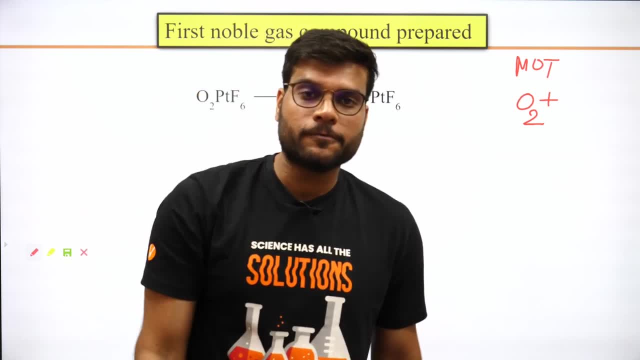 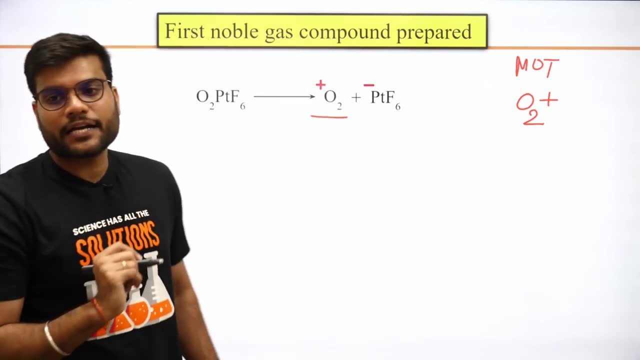 There is a species of which you take out the bond order. You check the magnetic, diamagnetic and paramagnetic properties. Do you remember O2 plus? Now, what are you doing? Just check it: O2PtF6 decomposes and gives O2 plus and PtF6 minus. 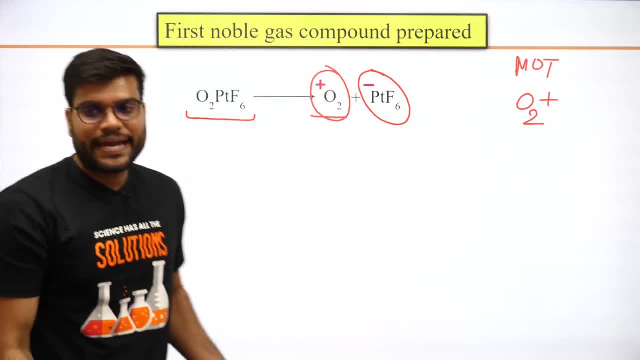 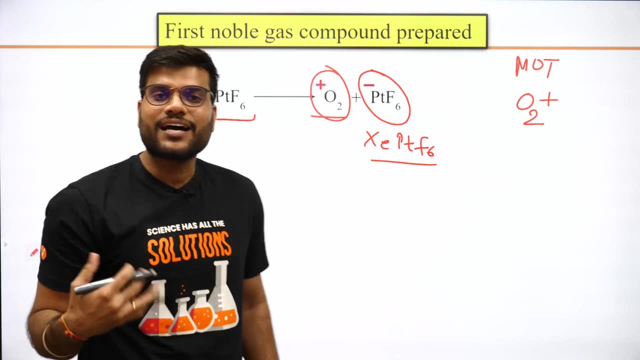 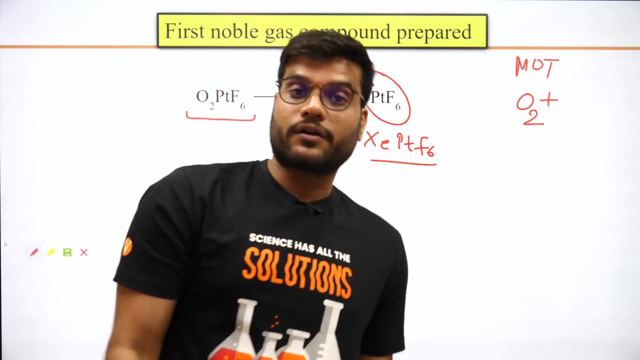 This makes anion. Now this anion actually reacts with Xe and Xe makes PtF6.. Now the question is: why did Xe do this? Xe was an inert gas. Where did this quality come from? It replaced the oxygen and took its place. 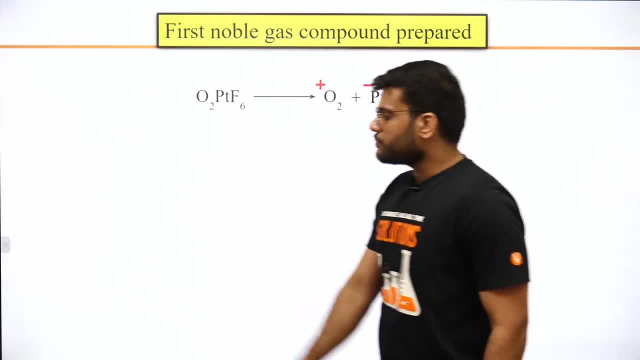 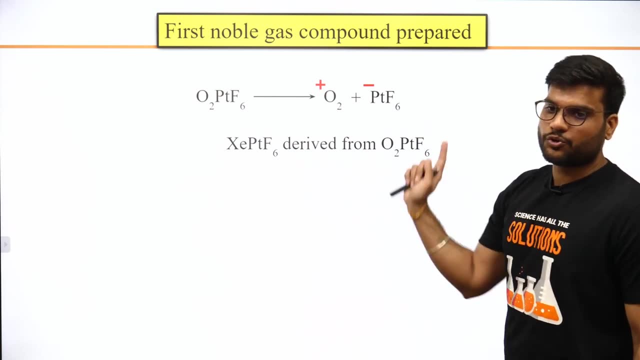 So I will tell you Now understand the reason for this. It is very important And the question has been asked on this. Just check it. We have derived O2PtF6 from Xe PtF6, which has happened in this way, which I have told you. 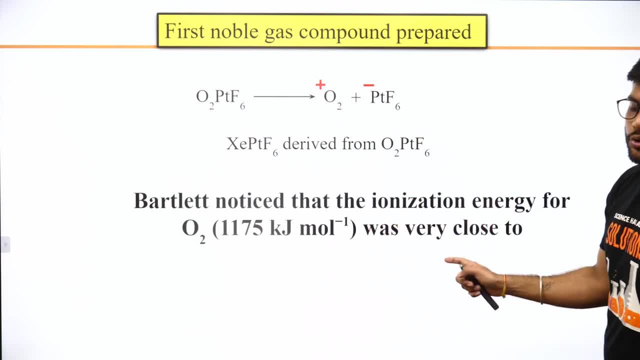 Now, what is the reason? Now look at it. This is the reason which you have to keep in mind Here. Barlet noticed that. just check it: The ionization energy for O2, how much is it? 1175,, don't remember this. 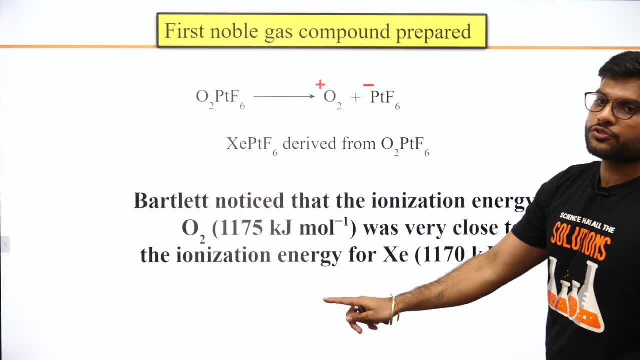 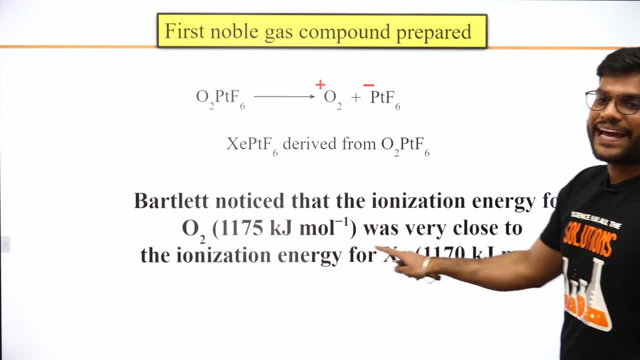 Was very close to. was very close to the ionization energy. Was very close to the ionization energy for O2.. Very close to the ionization energy of Xe. This happened because O2's ionization energy and Xe's ionization energy were almost similar. 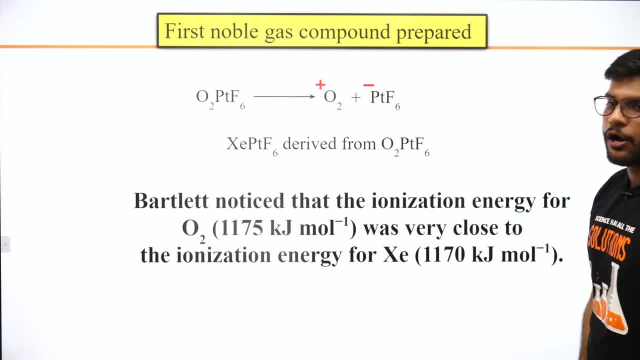 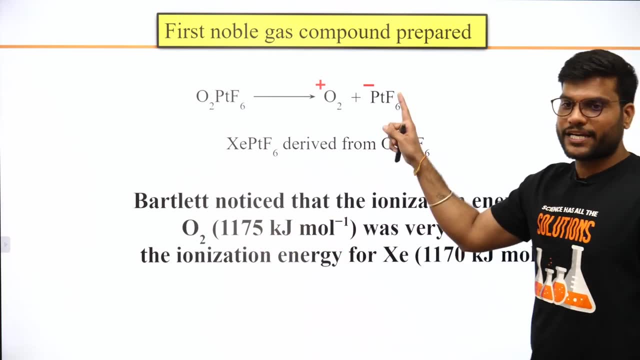 This is one of the reasons due to which the first compound was formed. I will tell you. Take a screenshot of this O2's ionization energy, due to which it got ionized. Just check it: It is getting ionized and making O2+. 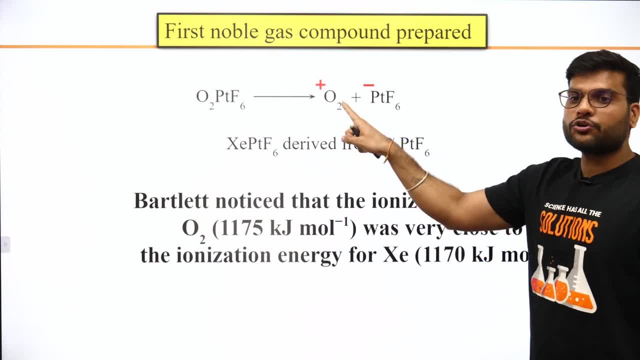 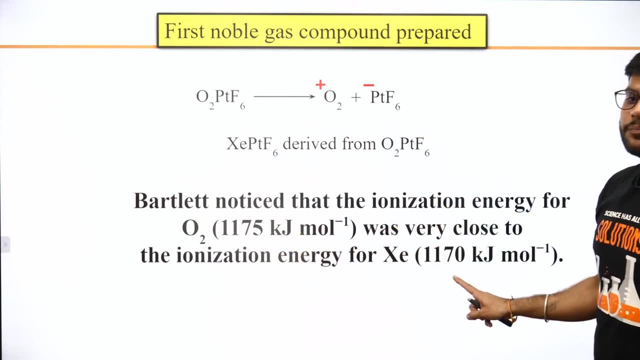 What is the meaning of ionization enthalpy To extract electrons? So from here you have extracted an electron from O2.. Its ionization enthalpy is 1175.. The same ionization enthalpy of Xe is also there. 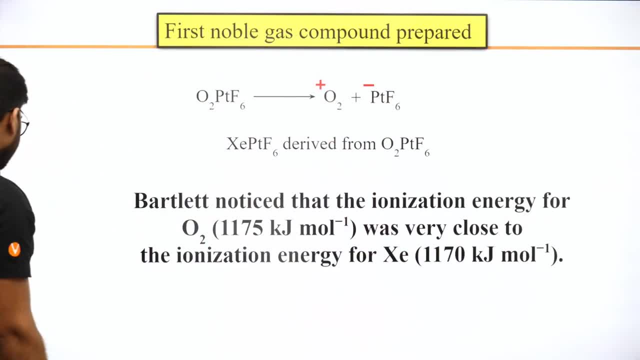 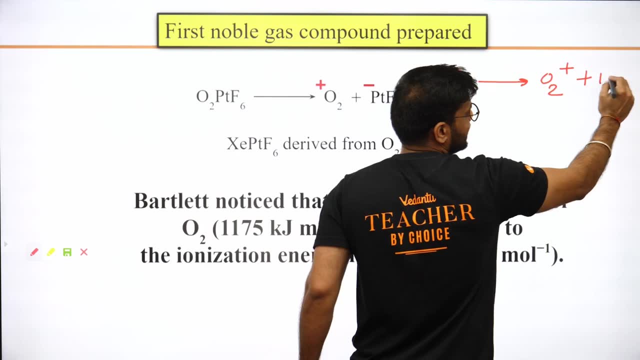 Now understand it a little better. To understand it better, just understand Here: if you have to extract an electron from O2, then it will be converted into O2+ And one electron will be extracted out. This is what we are talking about. 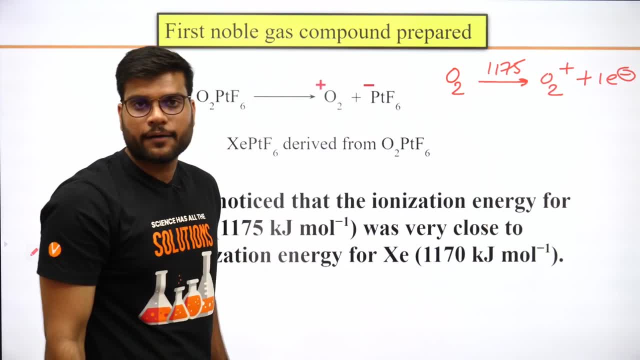 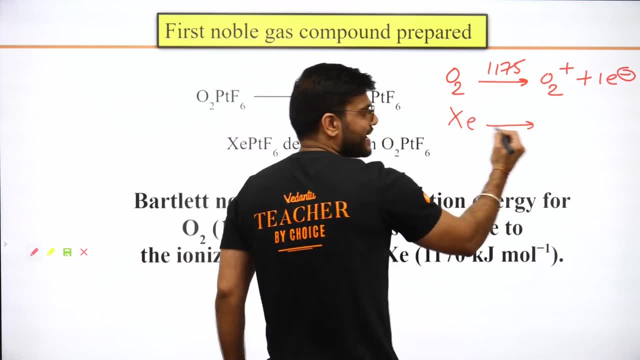 And it will take 1175 kilojoules per mole energy. When so much amount of energy is being used to make that compound, then the same, a little less than that. Xe can also do this work, Xe plus and one electron is extracted. 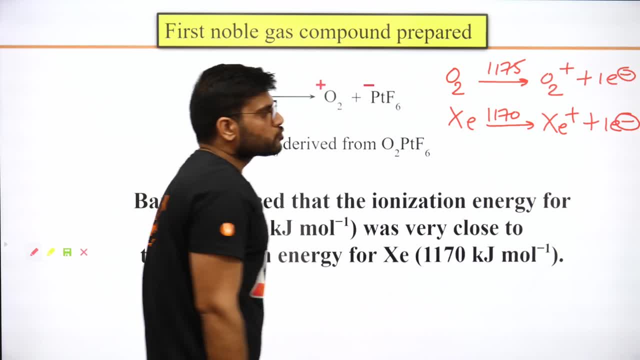 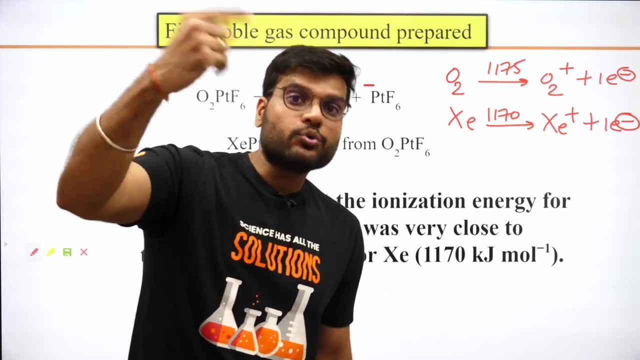 From here also, 1175 kilojoules per mole energy is being invested. So the work done by Xe, the work done by O2, that work can also be done by Xe For a little less amount of energy than that. 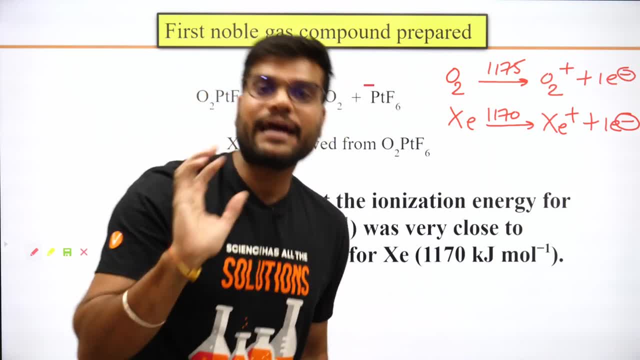 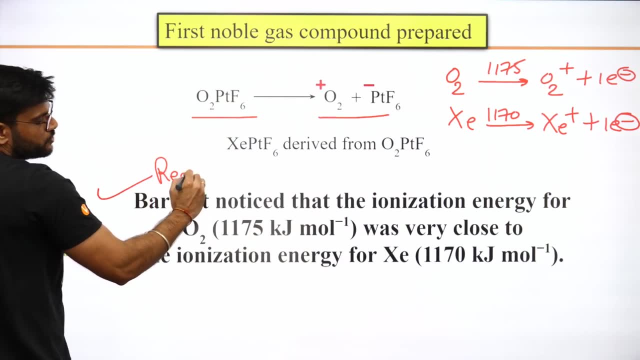 So this means that the compound could have been made by Xe. This is the overall meaning of this. So here, just check. This is the reason for that, And this reason has actually been asked in the exam. Now, this is really very important. 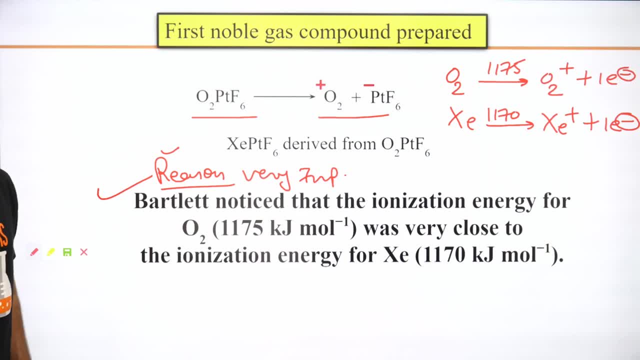 And I am telling all of you that please take a screenshot of this. Take a screenshot, my dear children. Take a screenshot. Take a screenshot One, two, one, two, three, four. Take a screenshot, my dear children. 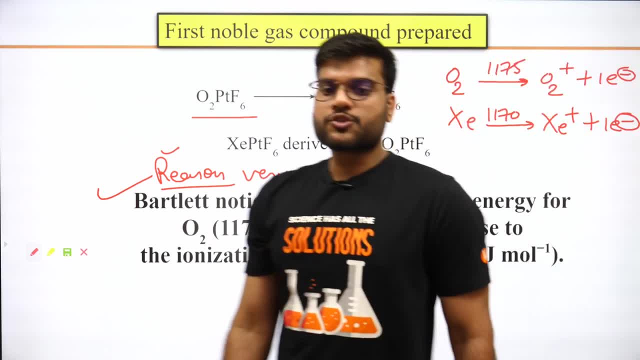 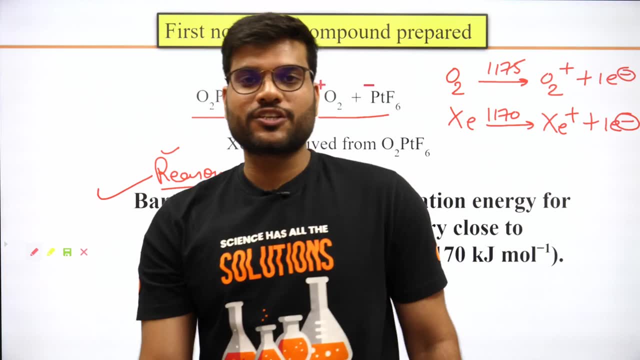 Take a screenshot. Take a screenshot quickly, Very good. So here I think you have understood. I think you have understood M M Keshal, Mr Keshal, Okay, Kailash, What is Kailash? 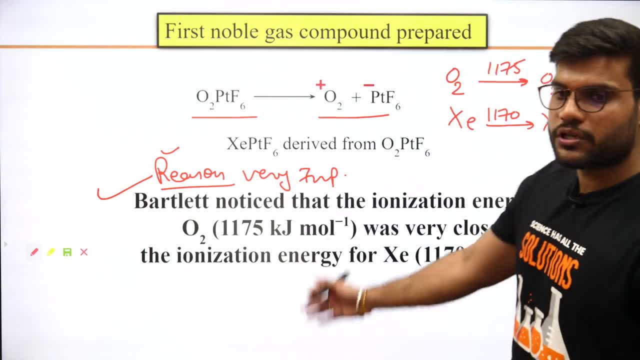 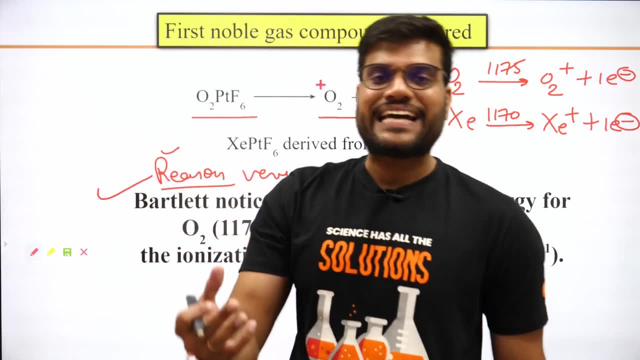 Thank you so much for coming Today. we have to finish it, And I think you have noted it down. Did you take it? Very good? Come on Very good. Now let's move ahead, Because here Xe is such that it makes compounds. 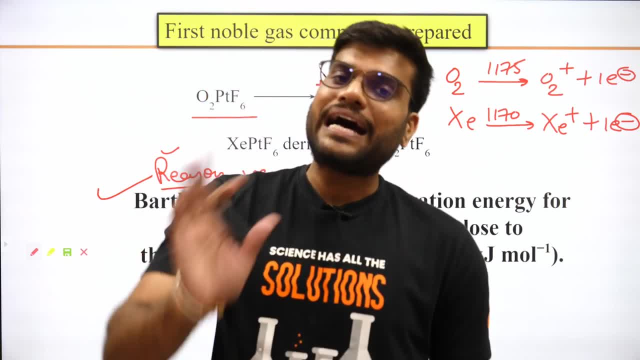 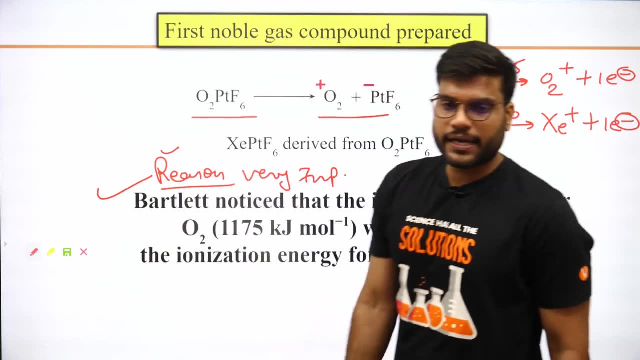 And Xe is such that it can also show chemical reactions. So today we have to study Xe, And the most questions are asked on it. So here, now we start the real game. Okay, So you note it down. 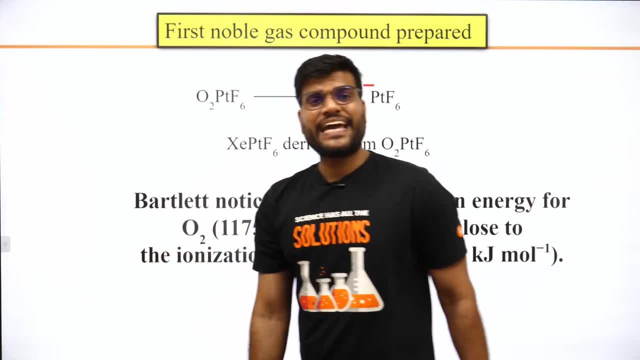 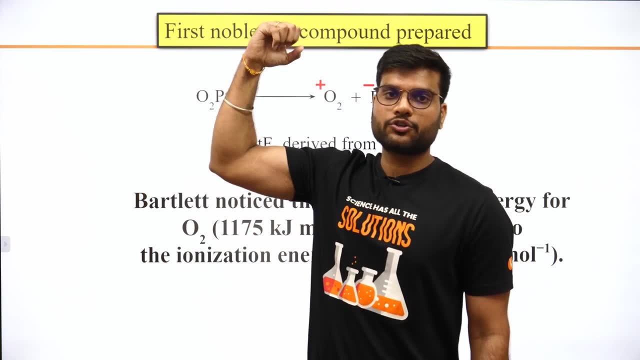 Very good, That's really brilliant. Today is the day of the game, Today is Mr Dhyanchand's birthday, Okay, And today is Fit India. So I will tell you all that if you become fit, then India will also be fit. 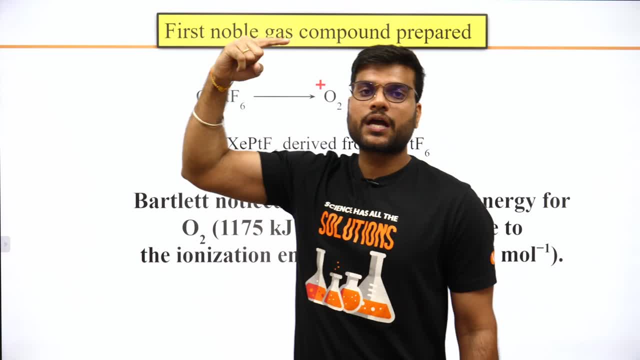 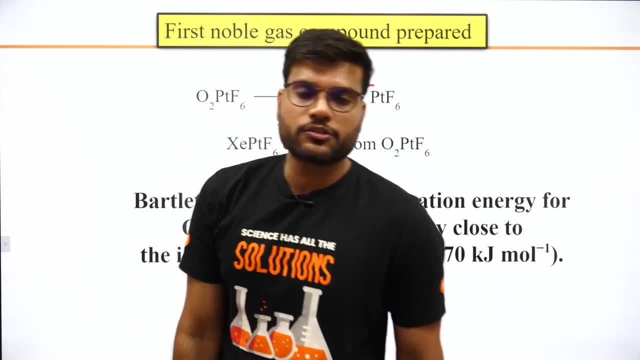 So I am telling you all to check it out. Yesterday I made a diet video here How to become from zero to hero. I am telling you all to go and check it out. It's not about making Dole Shole, Pak Shack. 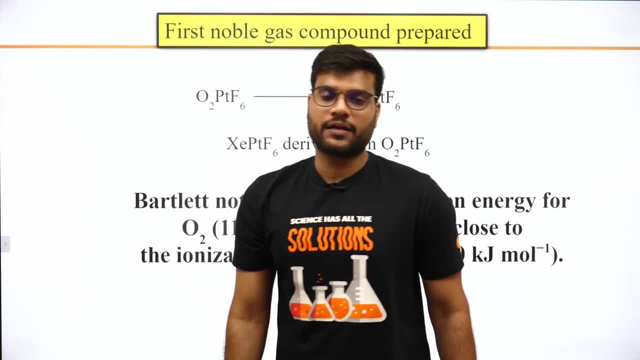 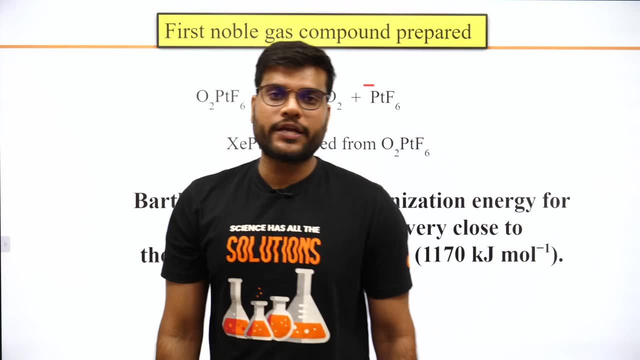 No, I am telling you to be super active, To run. If you get a chance to run, then you can run. Do you understand Means? you should be healthy. So if you want to make such a body, then you have to take care of your diet. 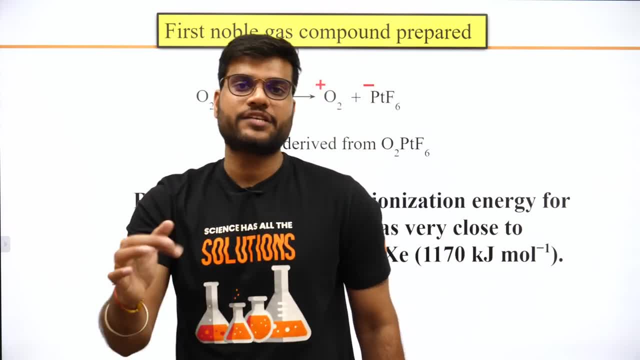 And for that I have made a very good video. I took a live session yesterday itself. Now just check it out. Come on, kids, Let's start Now from here. Xe's chemical reaction. Just check it out. 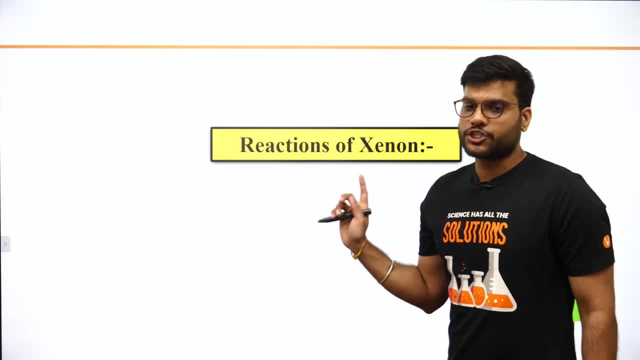 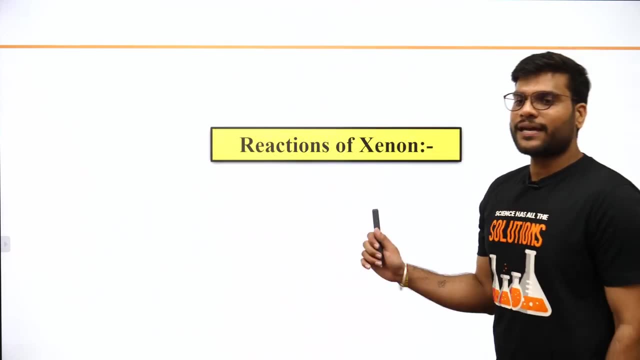 Our next topic is this: Reactions of Xenon. Check out of this, Kids. write it down quickly. Xenon's chemical reactions: Write it down right now. Xenon's chemical reactions. Xenon's chemical reactions: Write it down. 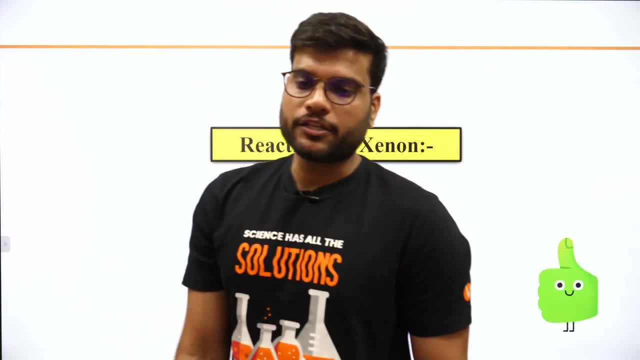 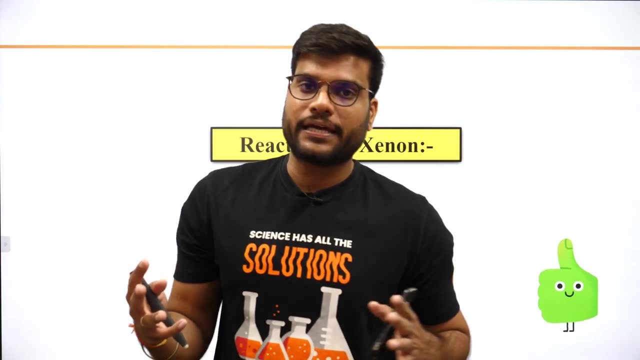 Write it down. It's very important. Everyone has written it down, It's very good. So come on. now We will see Xenon's chemical reactions And when Xenon's chemical reactions will make compounds. How is their chemical reaction hydrolysis. 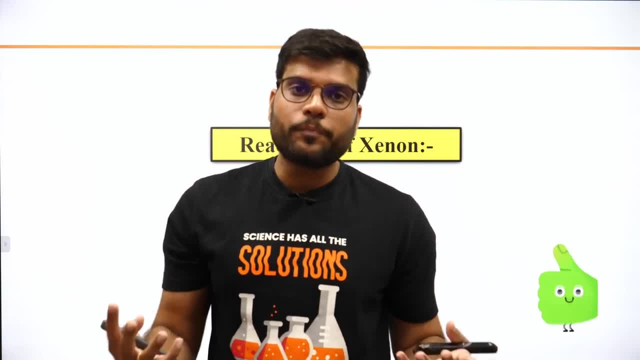 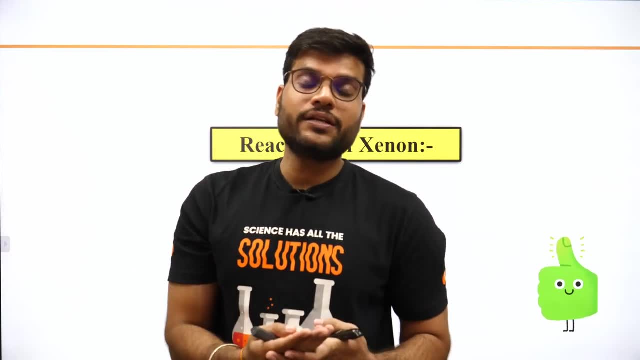 And actually questions come a lot above the hydrolysis of Xenon's compounds And that is the most important: Whose questions are asked? Okay, So from here, the question comes from 18 number group: The production of Xenon's compound hydrolysis. 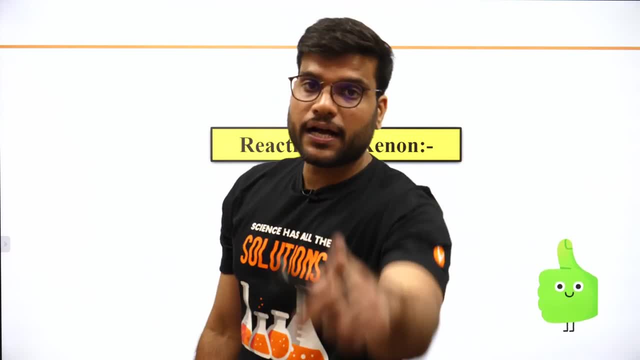 This question is asked, So please stay tuned, Because now the half hour is very important. So let's start. First of all, check the chemical reactions of Xenon. This is very easy. Suppose I have done the chemical reaction of Xenon. 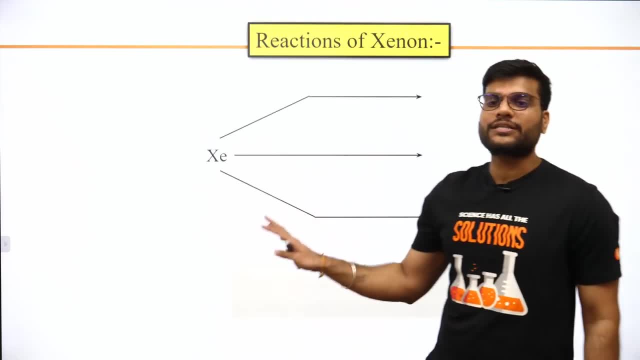 With whom? Check it out With fluorine. So what will it make? XZF2.. Now, here fluorine is not in large quantity, Do you understand? If you have done Xenon's reaction with F2, it will make XZF2.. 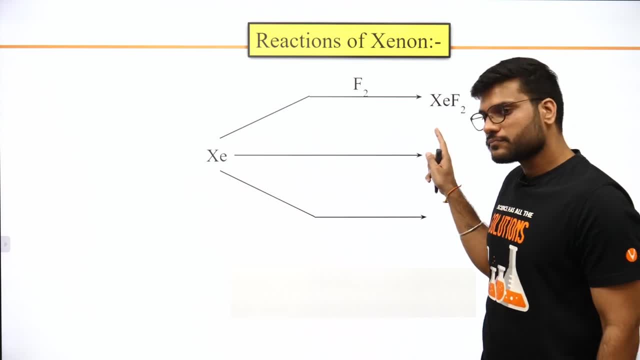 This is a very simple compound. If you have done Xenon's reaction with F2, it will make XZF2.. This is a very simple compound If you have done Xenon's reaction with XZF2.. If you have done Xenon's reaction with XZF2.. 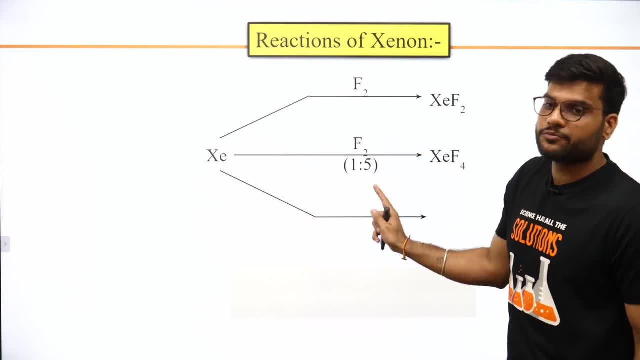 If you have done Xenon's reaction with XZF2.. But you have done it with 1 ratio 5.. Now understand the meaning of this. 1 Ratio 5 means if you have taken it with 1 mol, then you will have to take it with 5 mol. 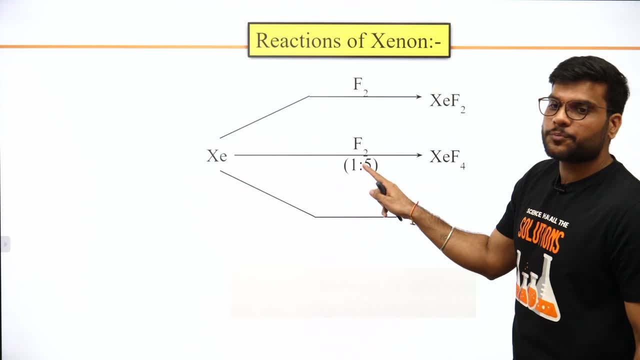 When you have taken it with 1 ratio 5, then it will increase to F4. The amount of fluorine will increase. It is very easy, Isn't it? So you just keep checking. This is very important, And if you have increased the amount further here. 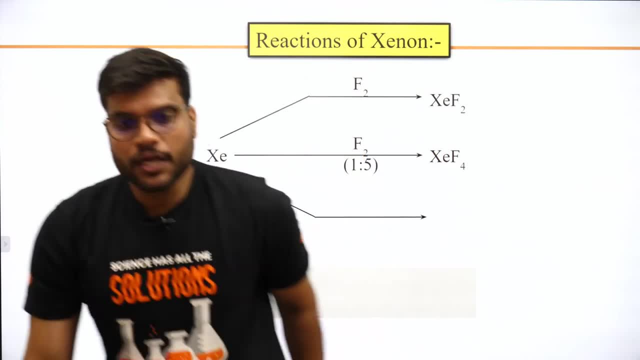 Meaning If you take fluorine with 1 ratio 20.. Meaning you take it with 1 and 20, then you will make XZF6. And this is very important. You just check this out. I will tell you the most. 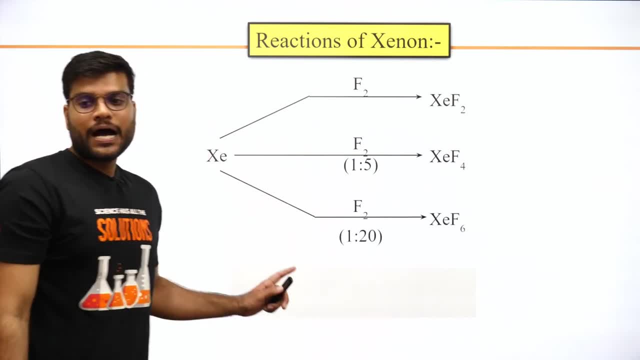 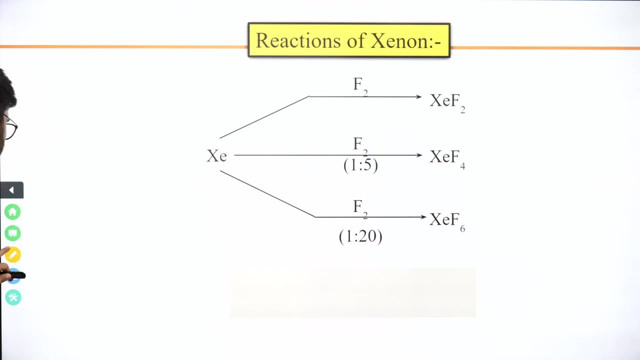 The way I have done. it is very simple. Just see Means. if you take fluorine in 1 ratio, 20 Means. if you take this 1 and that 20, Then you will make XZF6, And this is very important. you just check. 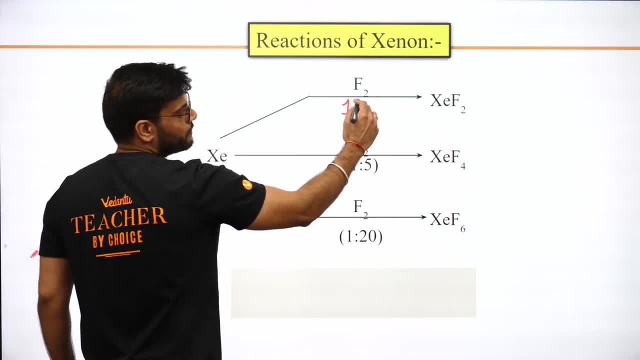 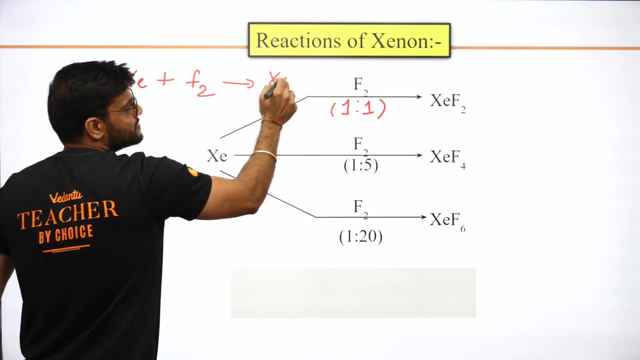 I tell you all Here 1 ratio 1 has been taken. If someone asks what has been taken in 1 ratio 1, Then XZ has also taken 1, F2 has also taken 1 And here XZF2 will be made. Are you getting it? 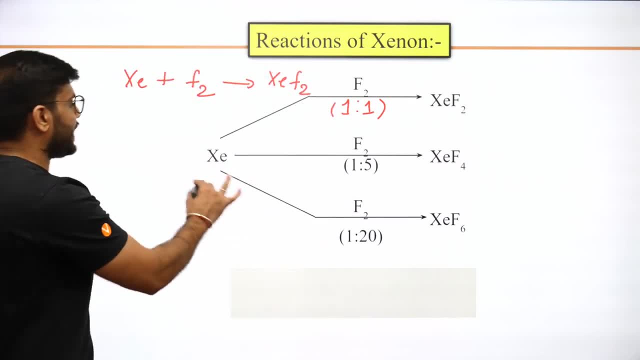 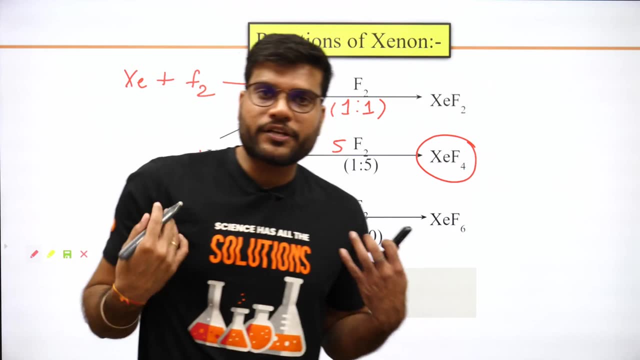 This is easy: XZF2 will be made. But if you take XZ1 here and this 5, Then you will just make XZF4. This much excess amount is required. Do you understand Experimentally? Where did it come from? No, Newton was given. 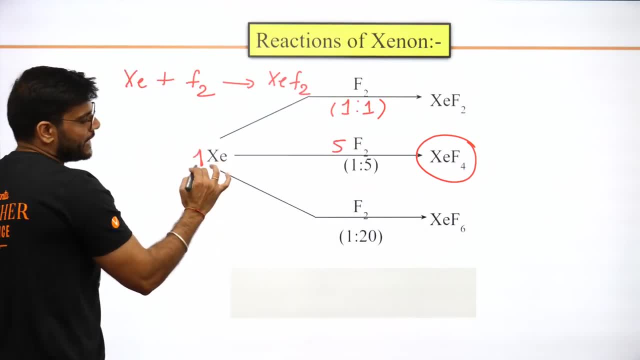 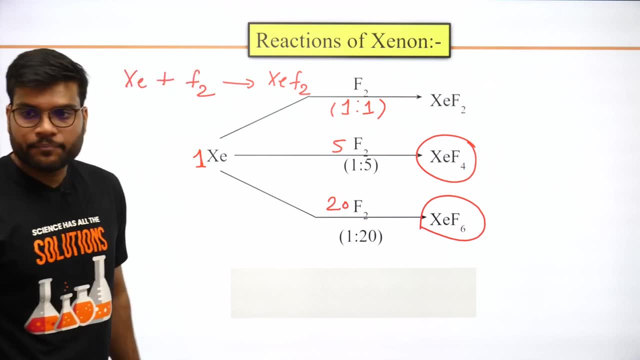 It came from experiment. Now see, If you take this 1 and this 20, 1 and 20, Then what will you get? You will get XZF6, which is very important. So now the whole game has come here. Now, here you have 3 fluoride of xenon. 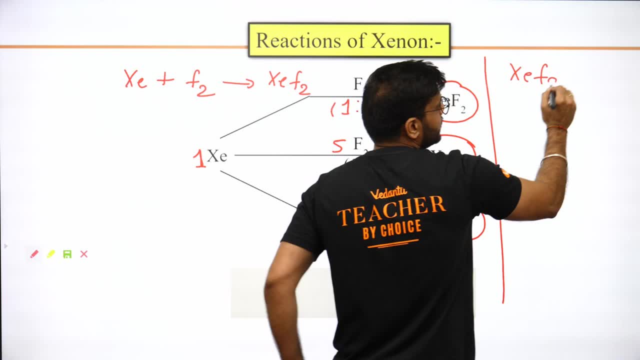 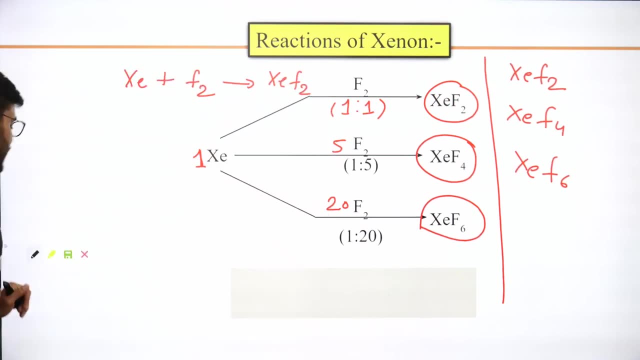 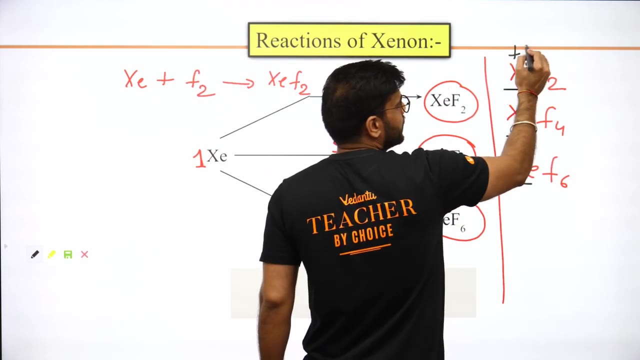 Which are they? XZF2, Remember, XZF4, XZF6, And the best way is What you do here Here. mention the oxidation state of xenon Here. how much is it Plus 2 Here? how much is it Plus 4 Here? how much is it? 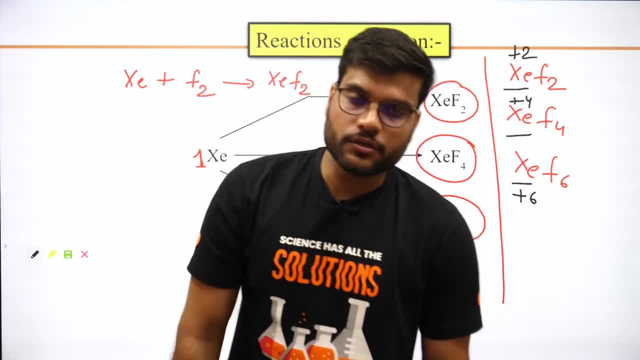 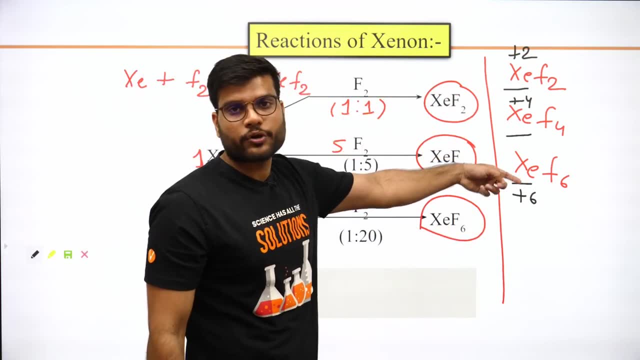 Plus 6, This will make 3 fluoride of xenon. They are called xenon fluoride. Is it clear? 3 compounds have been made, So here, xenon difluoride, tetrafluoride and hexafluoride have been made. 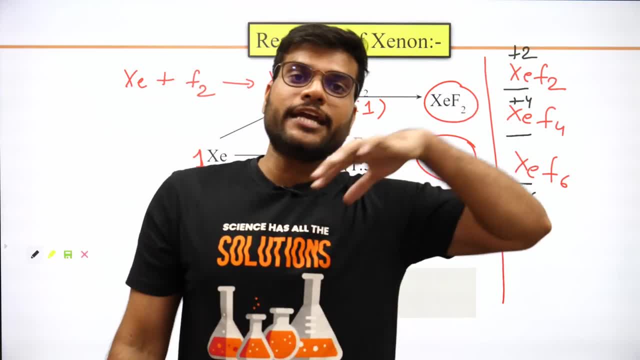 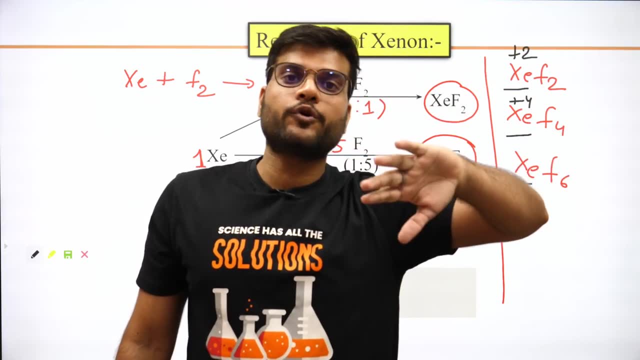 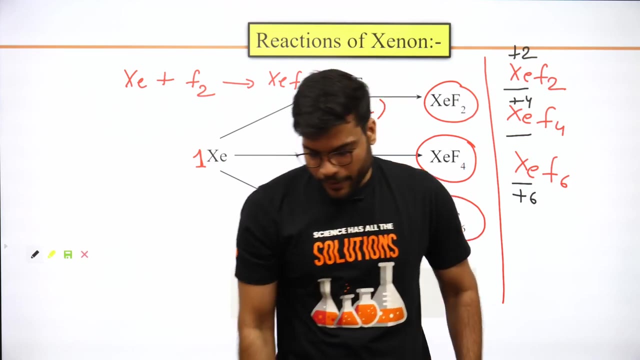 Now, from here, Your real game starts, Because if you do hydrolysis of these compounds, If you do hydrolysis of these compounds, Then definitely you will get compounds here, Which is very important. So let's start quickly Here. Come on, brother. Very amazing: Here chemical reaction is going to come in front of you. 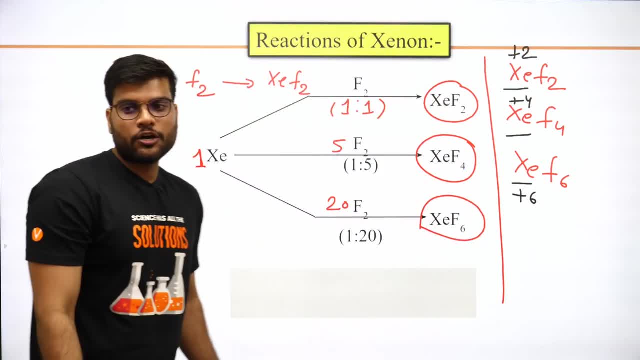 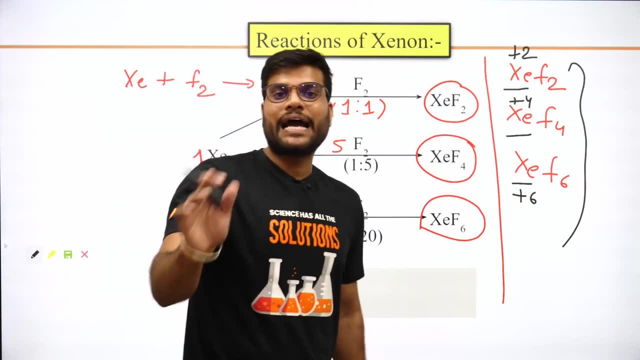 Which you have to take care of. Now. the game starts from here. So come on, If you do hydrolysis of these compounds, Then what compounds will be made? Just check that, Which is very important. I will tell you an interesting thing here, Here what you have to understand carefully. 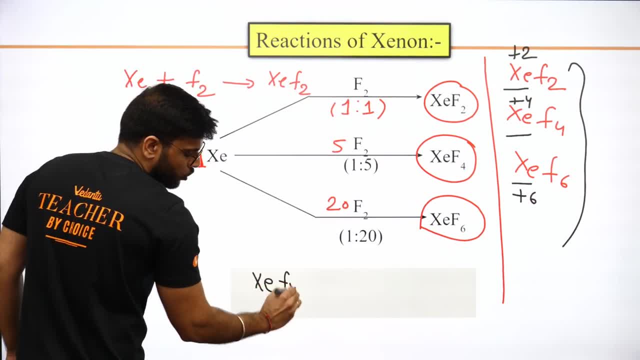 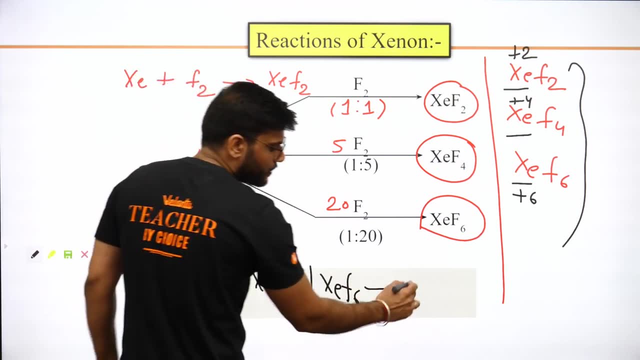 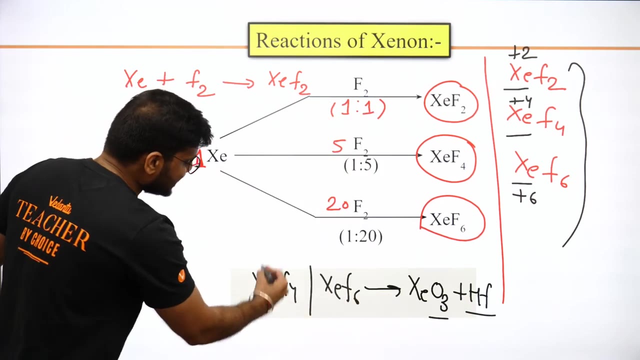 Check what I am going to write: XEF4 and XEF6. After both these hydrolysis, Two compounds will be made. One of them is XEO3 And the other is HF. This is sure. You can take XEF4 or XEF6, This XEO3 compound of them. Xenon trioxide. Xenon trioxide- Xenon oxide is sure. Note down this question. This question has been asked many times. I request you, Don't go anywhere And note down this Whenever you do. hydrolysis of XEF4 and XEF6. This question has been asked many times. 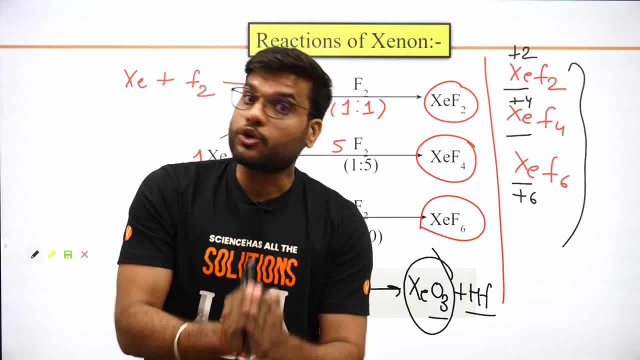 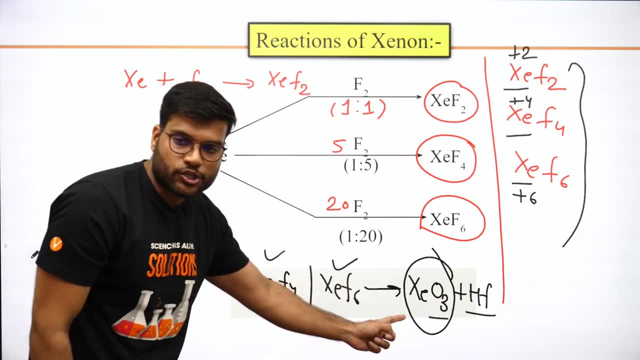 Note down this. There is a question about this in NEET, So don't go anywhere. Stay here, Don't go anywhere. Note down this: When you do hydrolysis of XEF4 and XEF6, Then XEO3 and HF will definitely be found. What will be found? 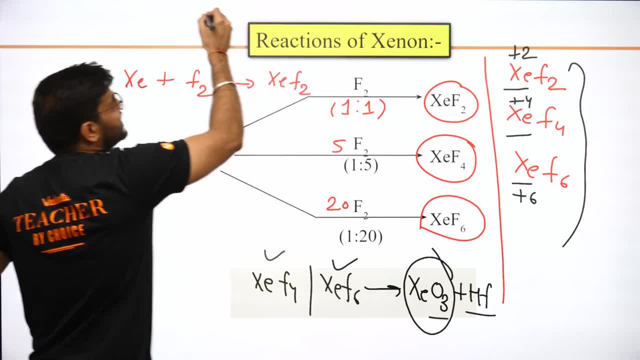 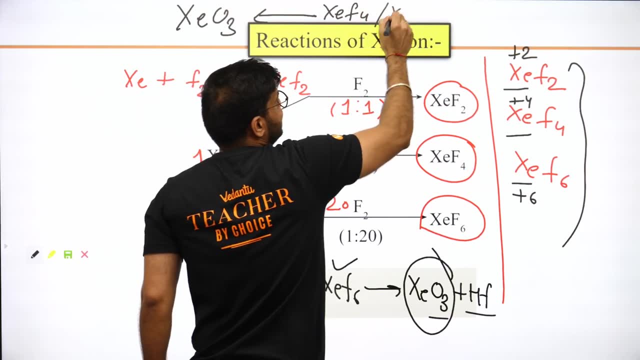 We will see. I have given you the answer. Please check. Everyone. write in the chat section. I will go after this. XEO3 will be found. You will be confirmed. Through whom? Through XEF4 and XEF6. My dear children, It is very important. It is very important. 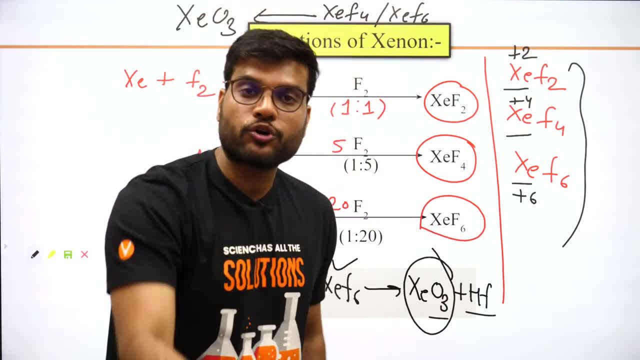 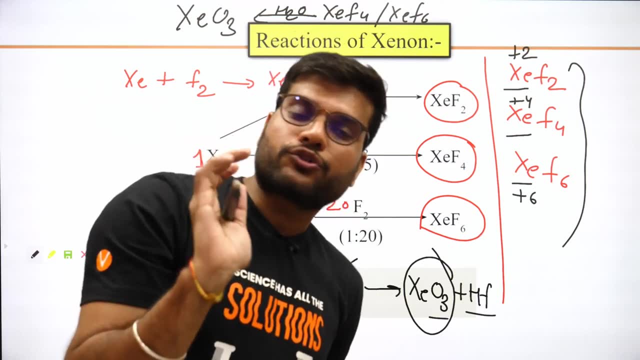 You note down XEF6 and XEF4. Both have hydrolysis. Hydrolysis means You have to get the reaction from water. I will tell you the reaction completely, But you will get it from XEO3. Now. this is very important. Now let's move ahead. 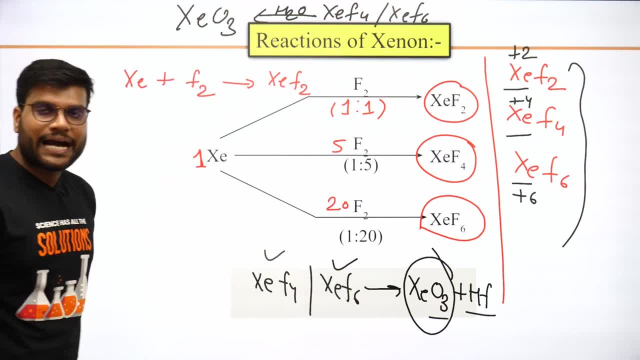 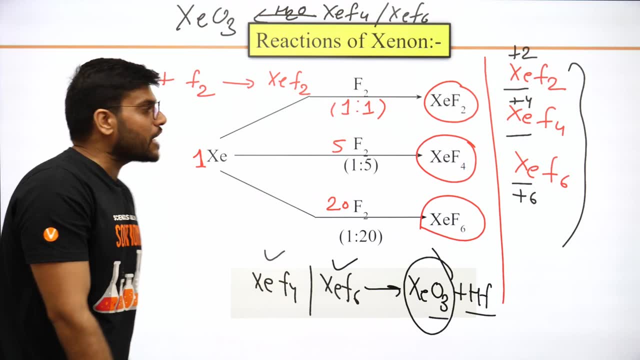 I will show you the reaction, Which is very important, So let's go From here Almost. we will finish in the next 15 minutes, So keep patience for 15 minutes And stay here, Okay, Because now your 4 numbers will be confirmed, If you have seen the next 15 minutes carefully. 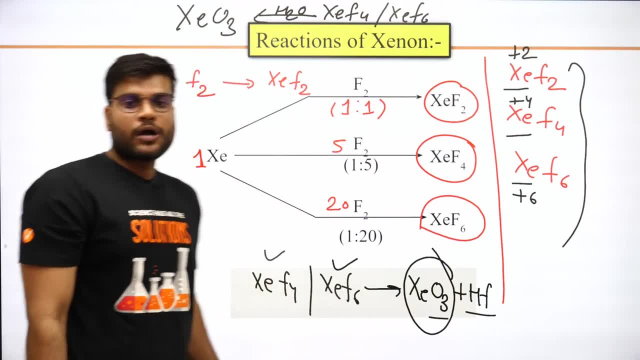 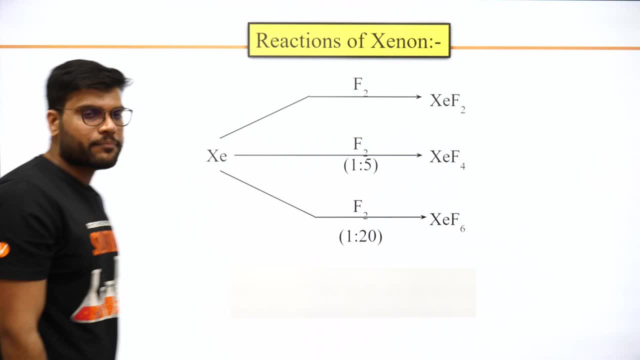 Then I give 4 number guarantee It will be confirmed. So don't go anywhere. Okay, So you note down this. Now let's go ahead. Take a screenshot. 1, 2, 3. Take a screenshot, My dear children. Take a screenshot Now I will tell you the chemical reaction. 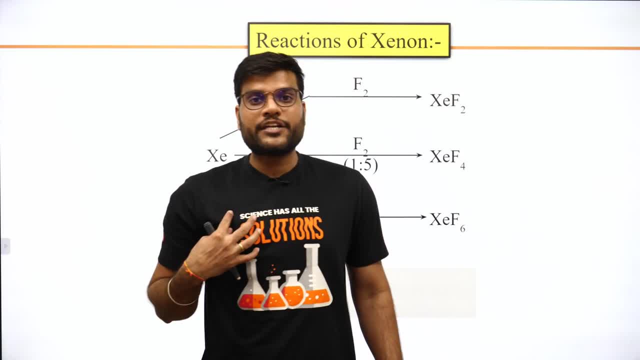 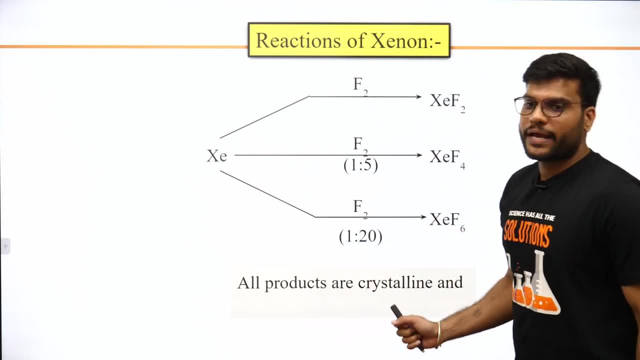 How to remember. I will also tell you that Because I am your tutor. I will also tell you the short trick: How to remember. So let's go for that, man, Come on, let's start quickly. So from here, If you note down one more thing: All products are: 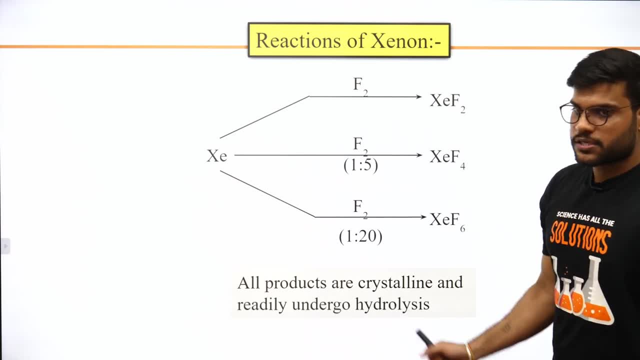 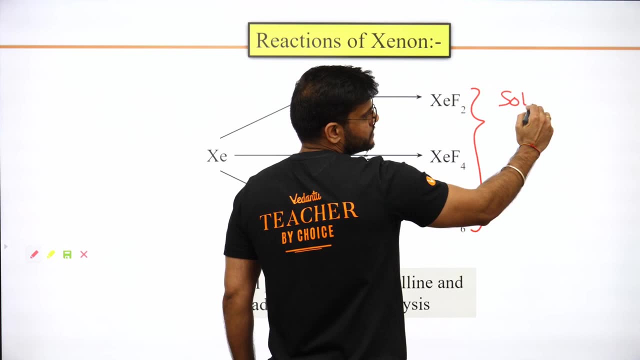 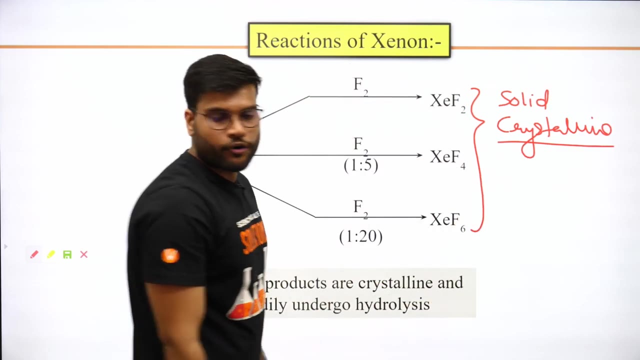 Crystalline and Readily undergo hydrolysis. All these products, You will understand carefully, They are in crystalline form, They are solid, They are in solid crystalline form. They are in solid crystalline form. Okay, They are in solid crystalline form. And second, 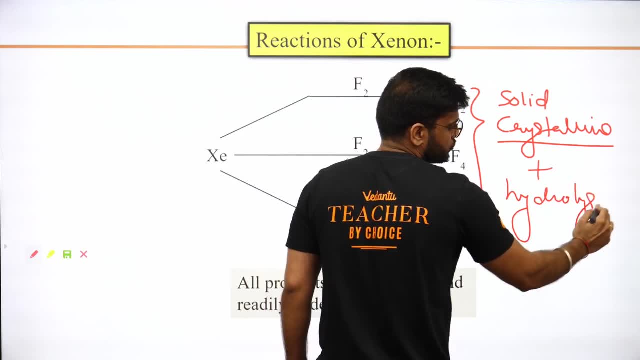 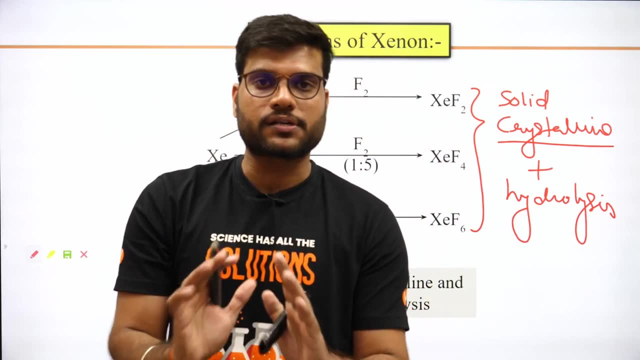 They are easily. Hydrolysis is possible. That's what we are doing. First of all, They are in crystalline form. Second, Their hydrolysis is possible. You can easily Hydrolysis. So come on, Let's start quickly. Let's get their hydrolysis done. 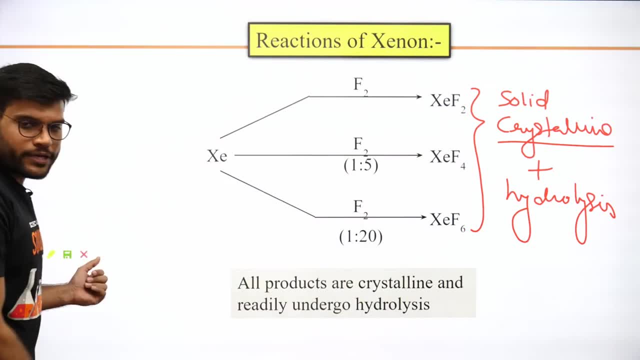 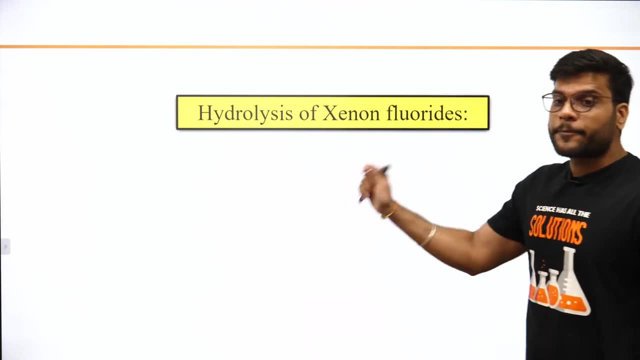 Did you take a screenshot? 1, 2, 3, 4, 5. Come on, Now, let's get their hydrolysis done. So see, Come on, brother, Now our most important topic of our 80 number group Is here. Bigger topic, Important topic: Nothing You note down. 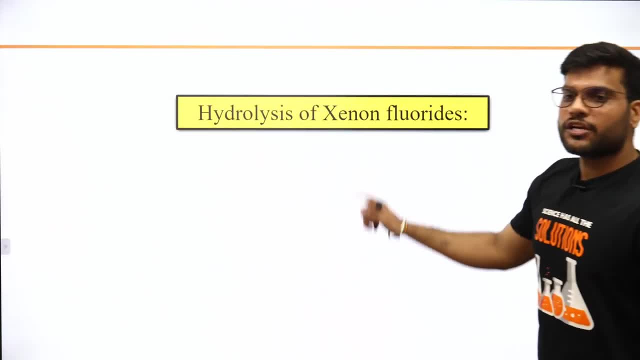 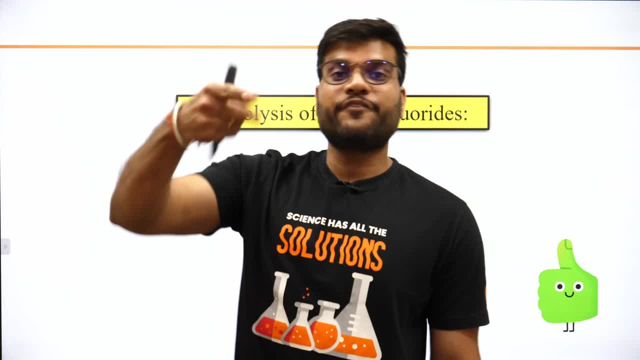 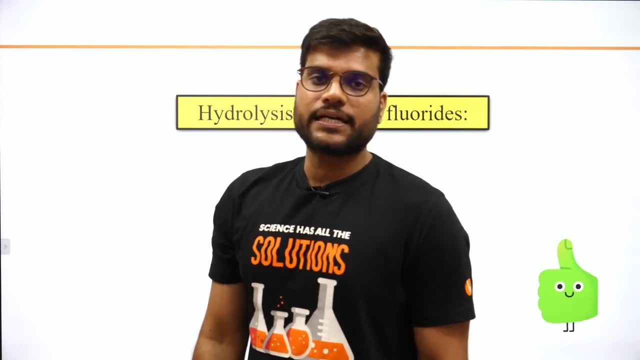 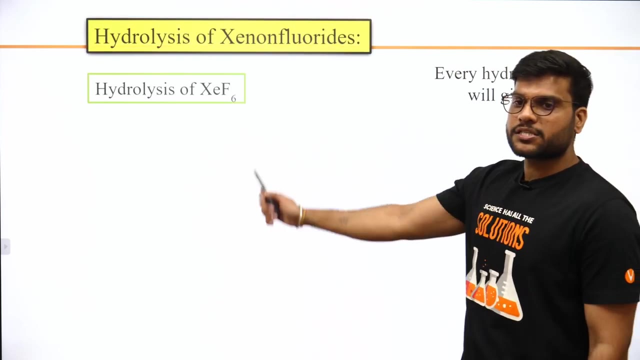 Whom Zeno fluoride Will we make To do XZF6, XZF4, XZF2 Compound? Small introduction: I told before How to remember chemical reaction. Let me teach you. Come on, Okay, Come on. So Hydrolysis. Now you should check First who We are hydrolyzing. 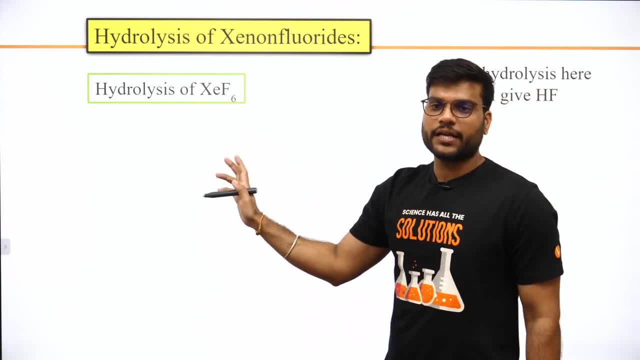 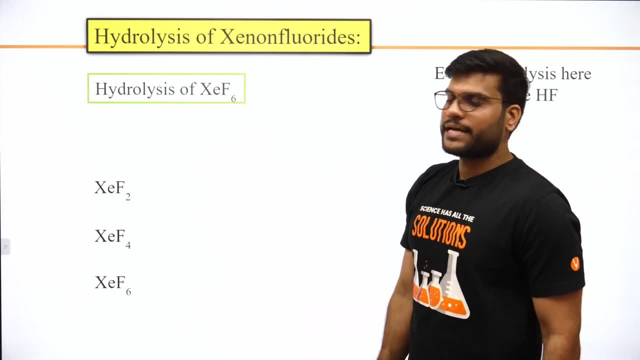 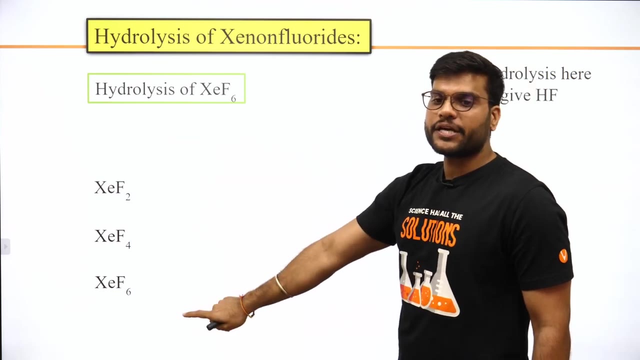 XZF6. Okay, We are making XZF6 idolysis. Check it If you did. Hydrolysis of XZF6. Well, Everyone. So first of all, let's look at F6. Then I will write the chemical reaction for F6. I will explain it to you in short. 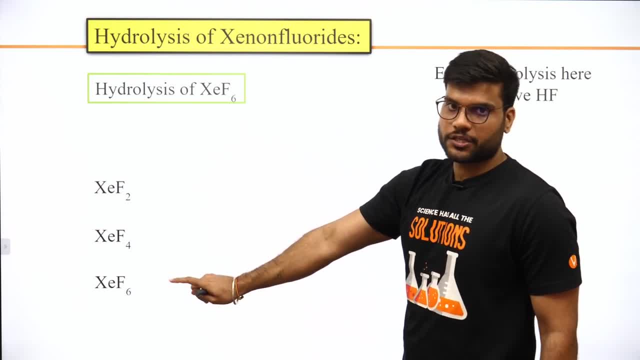 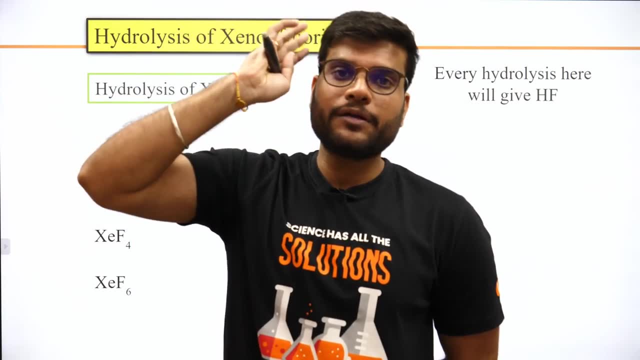 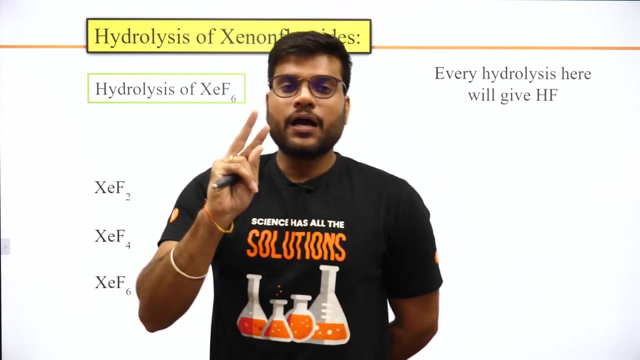 Does everyone understand. I will explain its resultant in short. Now you have to understand it carefully, And if you understand the hydrolysis of Xe F6, then you will not have any problem with F4 and A2.. So what do you have to do? You have to pay attention. What do you use in hydrolysis Water? 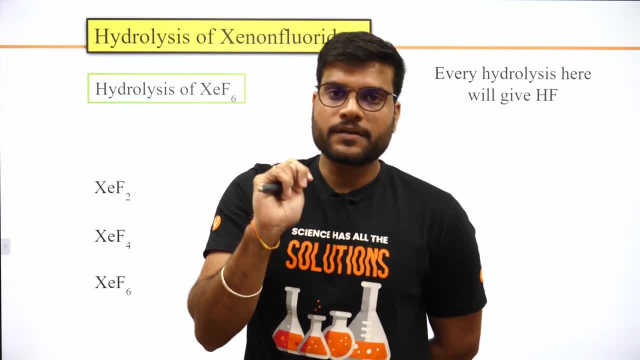 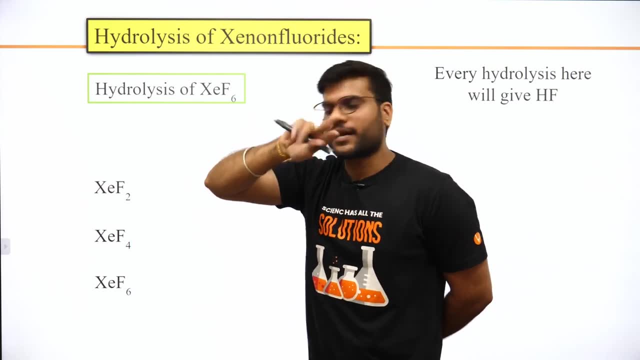 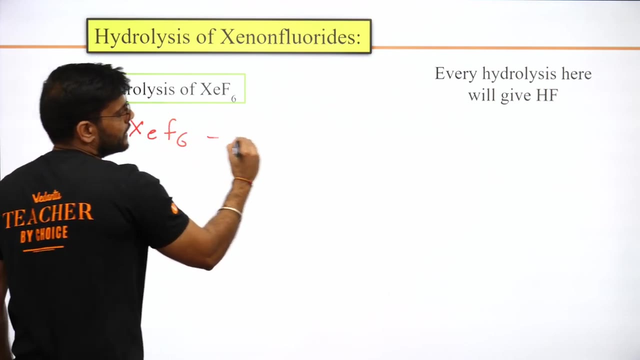 How much hydrogen do you have in water? 2. How much fluorine does this brother have? 6. You take out 2 fluorine from 2 hydrogen. Keep taking it out. I will show you how to do it. Look, assume that I am doing hydrolysis of Xe F6.. First I used H2O, Now you tell me how much hydrogen is there. 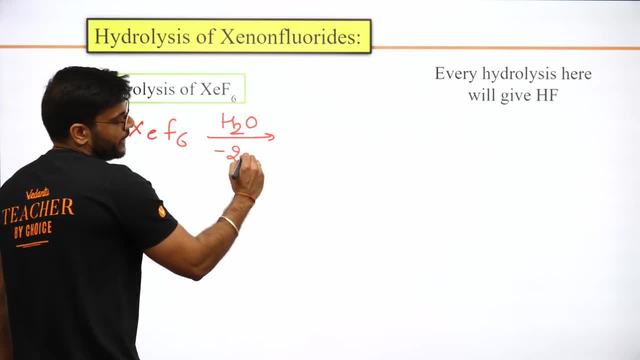 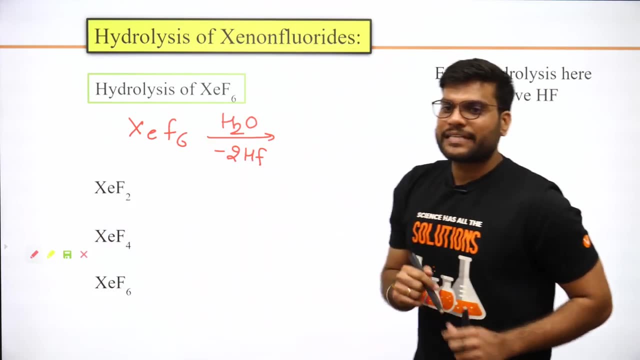 2.. I can take out 2 HF from 2 hydrogen and 2 fluorine. Yes or no? I can take out 2 HF, And we also know this, Just check. If you take out 2 fluorine, then there will be a deficiency of minus 2 here. 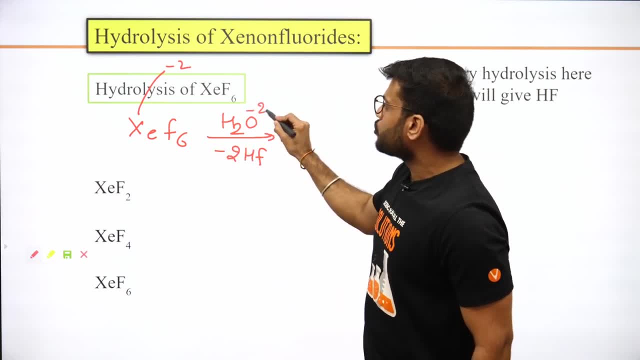 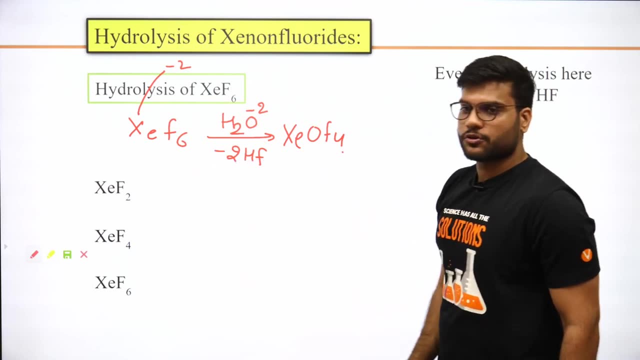 Because 2 fluorine has gone And we know that if there are 2 minus after oxygen, then what will be the compound here? XeOF4.. How easy it is: Take out 2 fluorine and give it oxygen. Is it hard? 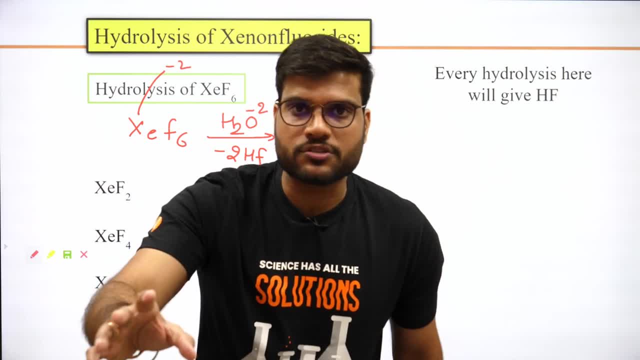 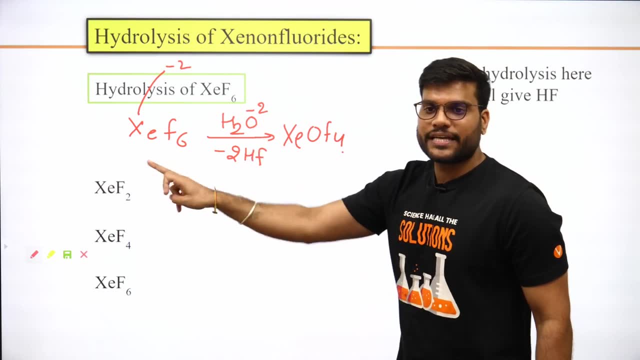 Do you have to do it? for this, You have to order a red color pot from Amazon. Tell me what I did. I took out 2 fluorine and made 2 HF here, Gave it oxygen. I took out 2 fluorine and gave it oxygen. Is it hard? 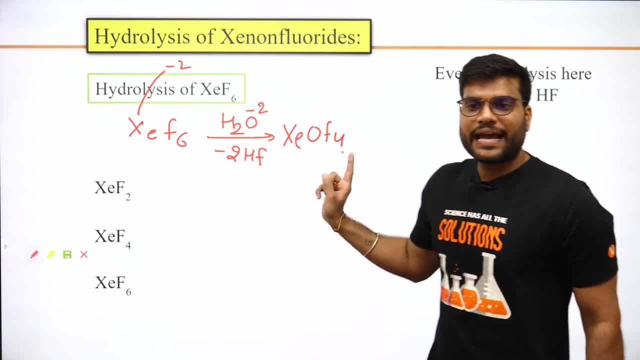 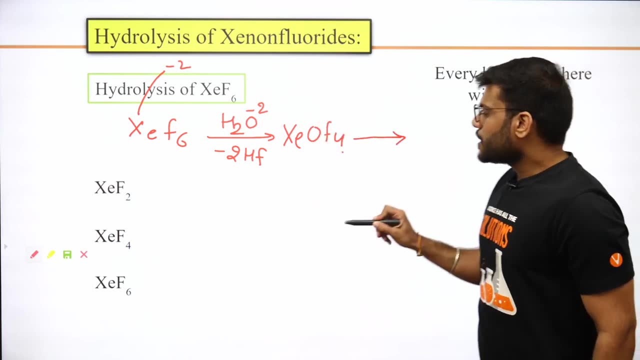 Do you have to take a pot of red color for this? Tell me, Is it hard? I took out 2 fluorine and gave it oxygen. There is nothing in it. Now let's move ahead. Just check From here: again, it has fluorine. 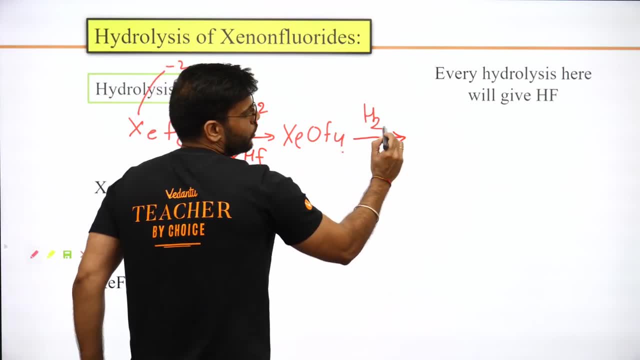 So what I am doing here, Just check: I am doing H2O hydrolysis. Tell me here how much hydrogen is there? 2.. How much is there from here? 4 fluorine. So I take out 2 fluorine. 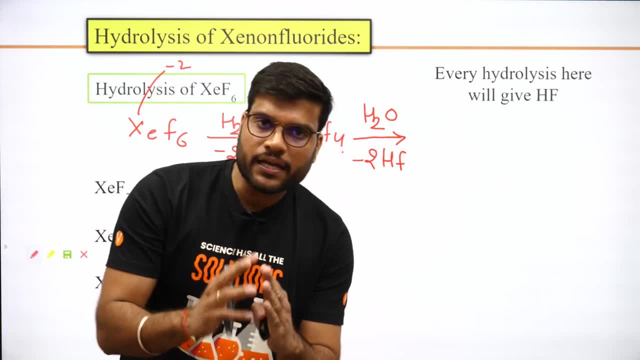 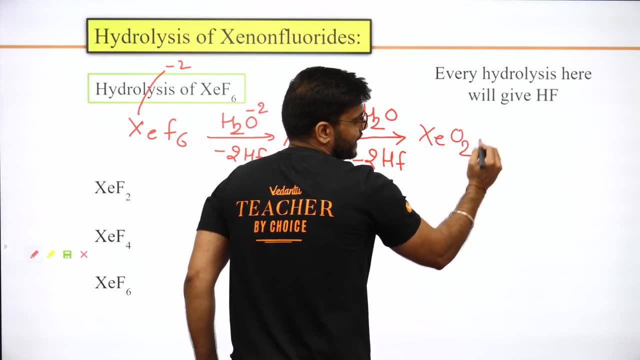 Take this: 2 fluorine makes 2 HF. So 2 hydrogen, 2 fluorine, 2 HF are being made. If you give 1 oxygen to it, what will it become? It will become XeO2F2.. Yes or no? Is it hard? 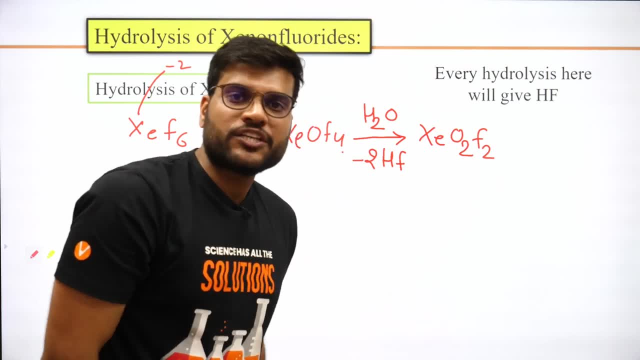 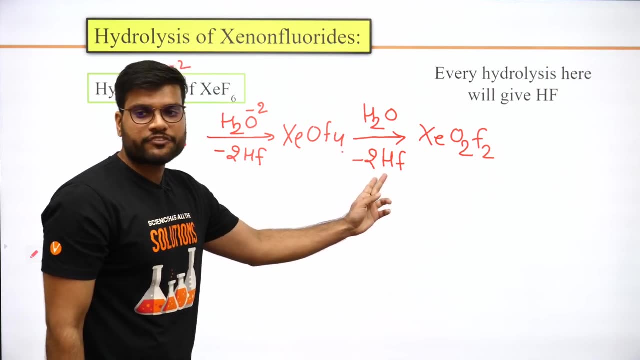 Do you have to wear a red color pot on your jeans for this? No, What did I do? I took out 2 fluorine, 2 hydrogen, 2 HF are being made. Now if I take 1 more oxygen here, then it becomes XeO2F2.. 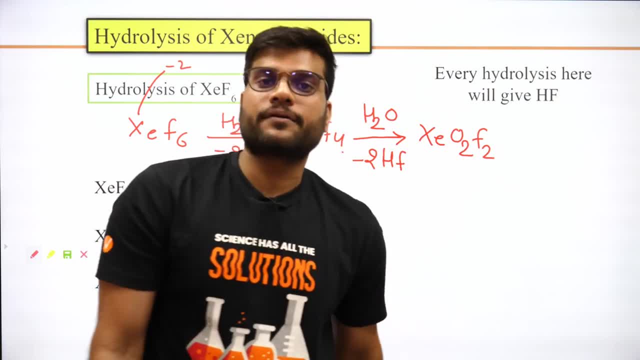 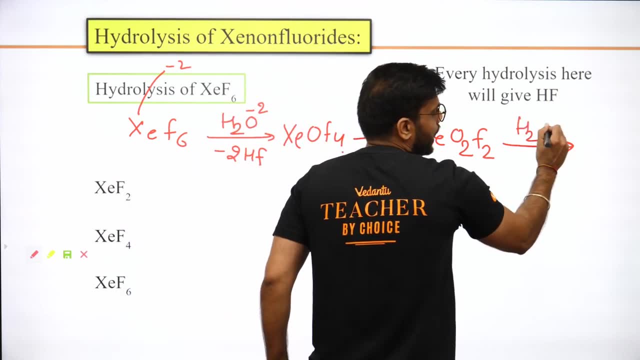 Is it hard? No, But kids don't even remember this. Now let's move ahead. Now we have 2 more fluorine, So take out 1 more water. If I take 1 more water, then 2 hydrogen, 2 fluorine will be taken out. 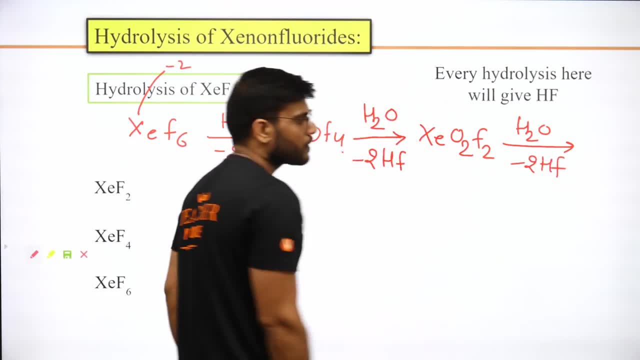 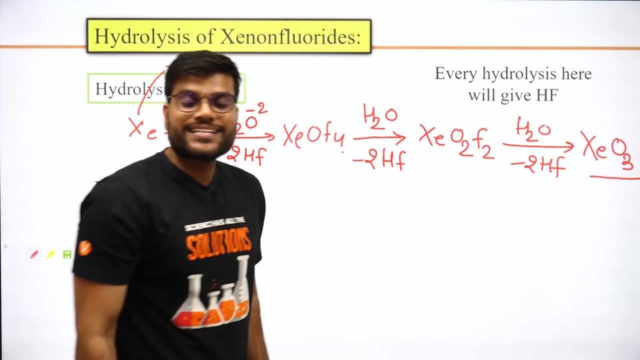 So what will happen here? 2 HF is taken out. Now tell me what will become the compound here. So, finally, compound is XeO3.. I had told you this XeO3, and what are you making together? Tell me. 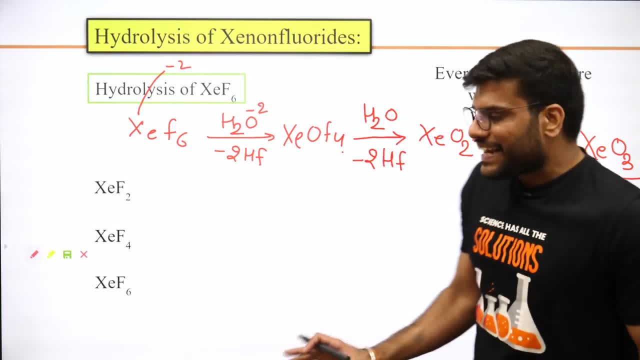 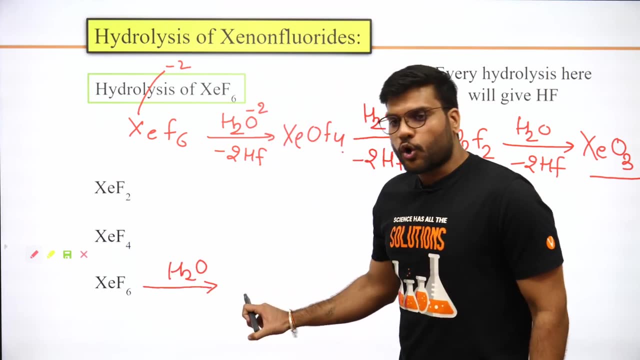 XeO3 and HF are being made together. So if you get hydrolysis done with total XeF6, if you get hydrolysis done here, then you will get 2 compounds which I told you in the beginning. What will you get? XeO3.. 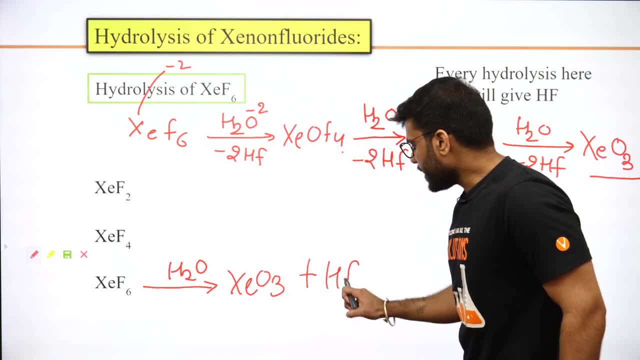 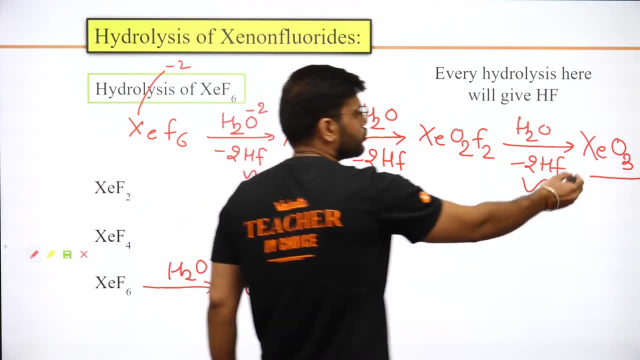 And what are you getting? second HF? See, you got this HF, this HF, this HF, And what did you get in the end? XeO3.. You got XeO3.. Yes or no? Tell me, Is it hard? 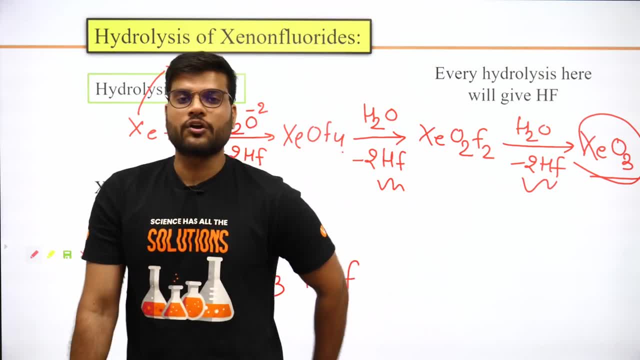 Will you have to buy a red colored cloth for this? Order it from Amazon. If you don't understand, then ask mom for a red scarf. Listen to the song. I can't remember the song. Red scarf, Take it and fly. 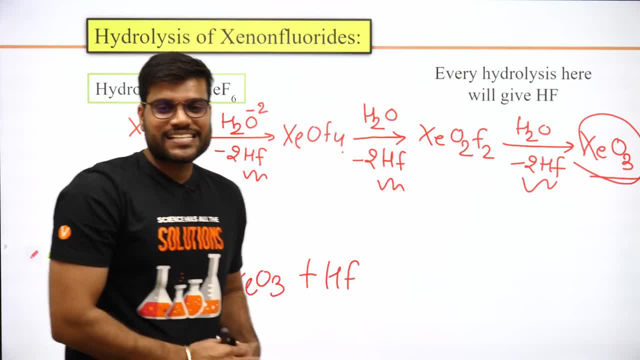 See, It is very easy. I think you must have understood How easy it is. if you don't understand this- And I wrote here the resultant of the last- What is going to happen finally? Finally, XeF6, H2O, XeO3 and HF will be made. 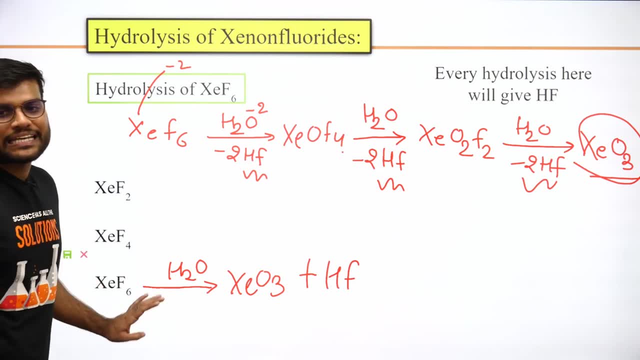 The matter is over. I have written here the resultant of the last. What is going to happen finally, Finally, what is going to happen finally? Finally, XeF6, H2O, XeO3 and HF will be made. 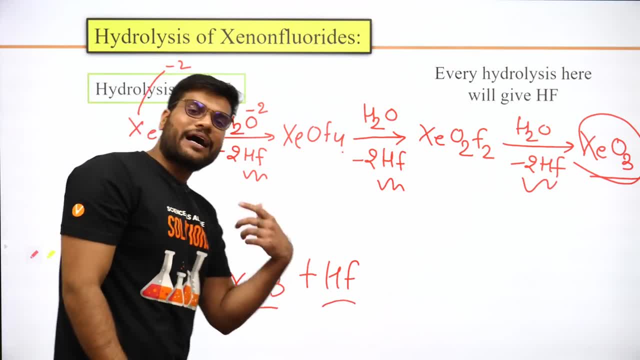 The matter is over. The matter is over. Money will be consumed. Did you understand? This is such an easy way. That's it. You have to do the same with everyone else. So now I will explain to you. This will be its sequence. 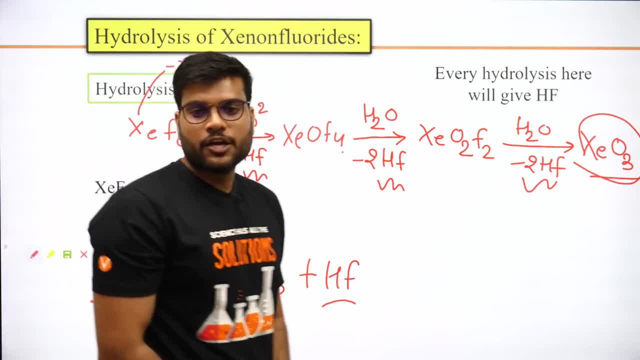 Now you just check How many fluorines are there here- Two. So can this be made? This cannot be made. XeO3 cannot be made under any circumstances. Are you getting it? This cannot be made. This cannot be made. 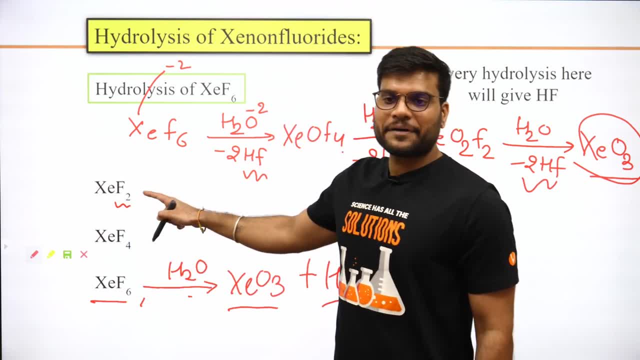 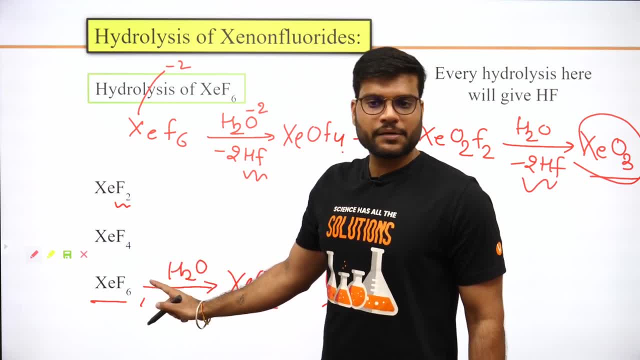 So come on, I will explain to you through the sequence You check once quickly. First of all, what you have to do is just check: If XeF2 goes with H2O, then there is nothing in it. If it goes, then it will make hydrogen 2, fluorine 2, what will you do? 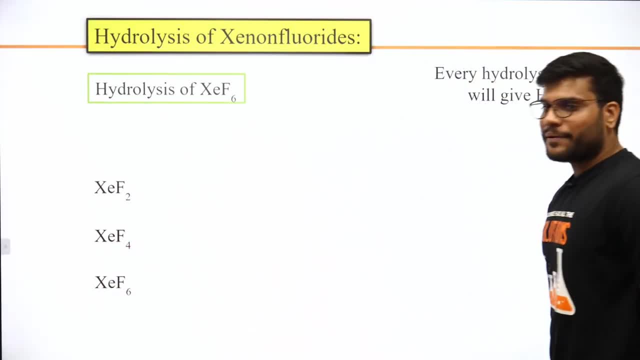 HF will be made Right Along with that. Xenon is separated from here. This is the first thing that we have to do. This is the second thing that we have to do. This is the third thing that we have to do. 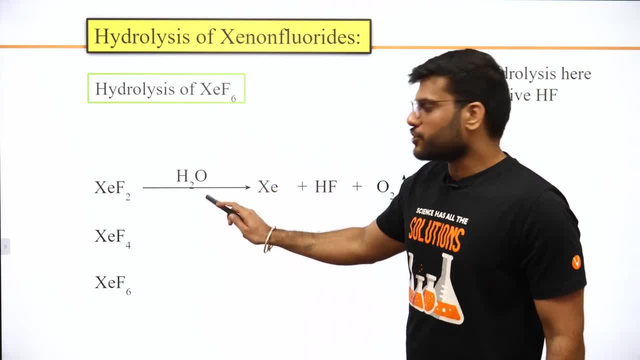 This is the fourth thing that we have to do. This is the fifth thing that we have to do. This is the fifth thing that we have to do. If you have done hydrolysis of XeF2, then you will get Xe. 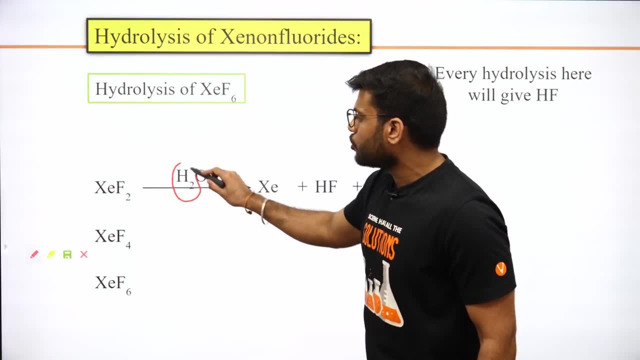 It is clear: This is the first compound. Xe is found And there is nothing left. H2F2 will make HF Two. half oxygen will come out of here and Xe will come out. This is very important. This is very important. 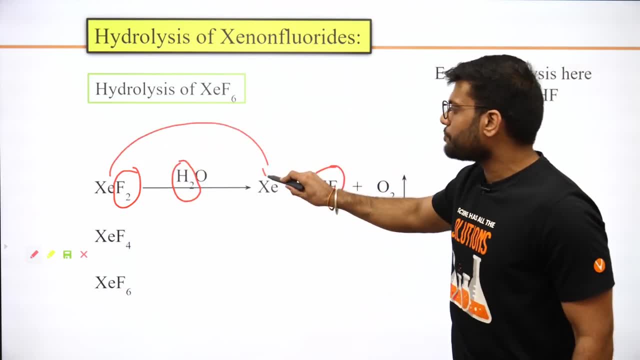 It is very important, So you have to do this. So this is the first thing that we have to do. You check once quickly. First of all, what you have to do is just check. If XeF2 goes with H2O, then there is nothing in it. 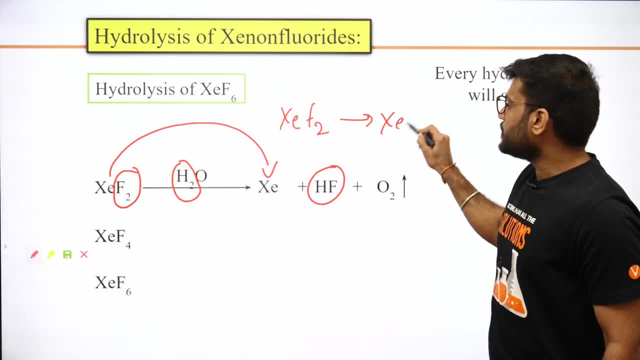 If it goes, then there is nothing in it. If it goes, then it is hydrogen 2, fluorine 2, what will you do? HF will be made Right. If it goes, then there is nothing in it. It is clear. 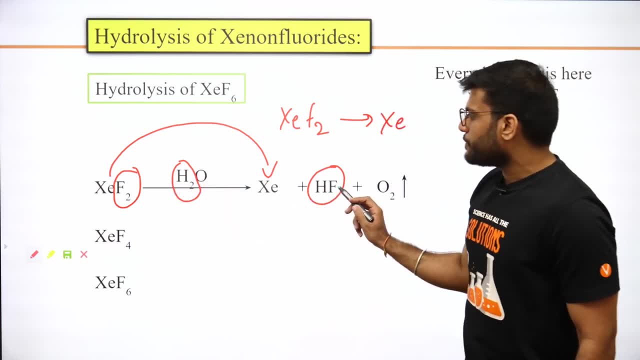 This is the first compound. Xe is found And there is nothing left. H2F2 will make HF Two. half oxygen will come out of here and Xe will come out. This is very important. Just note it down. This can be remembered very easily. 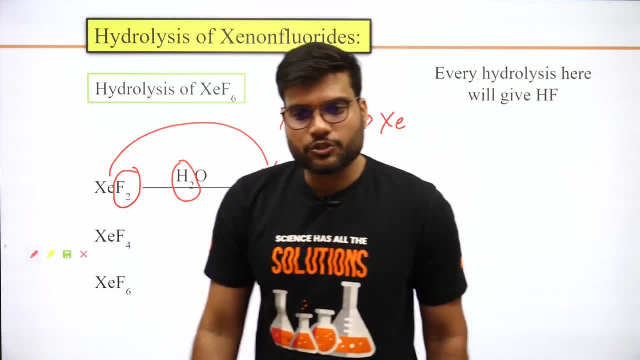 I will explain it again. Just check, Look again From XeF2H2O. I will take a question in a while. First of all, let's finish this. Someone is asking a question of clathrate in the middle. 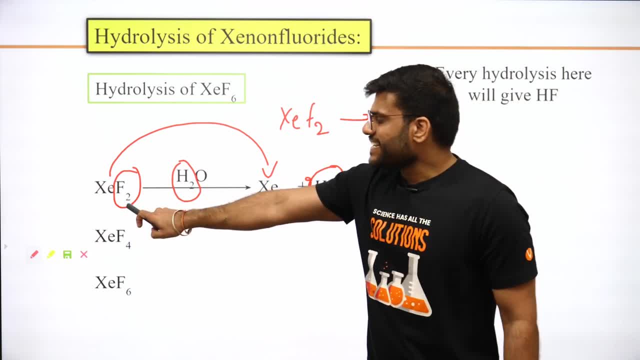 Do you know what happens When we are studying in school? we have to do this. We have to do this. When we are studying in school, we have to do this. When we are studying in school, we have to do this. 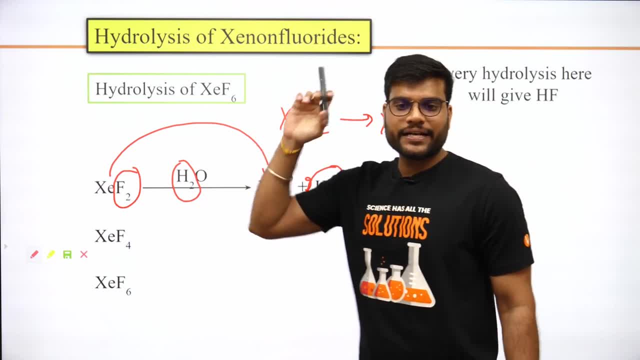 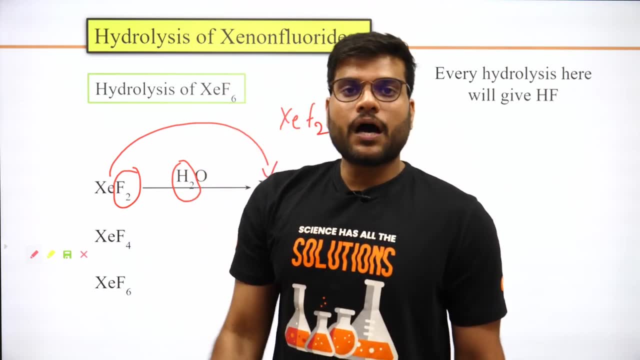 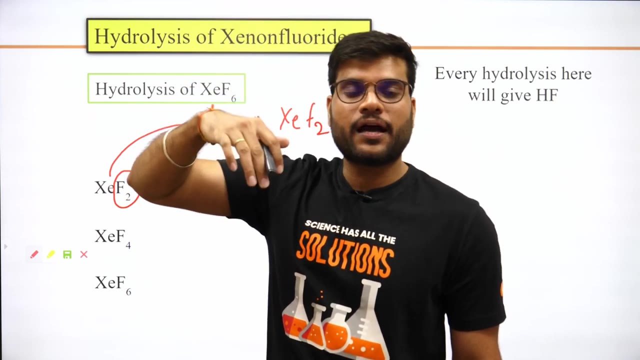 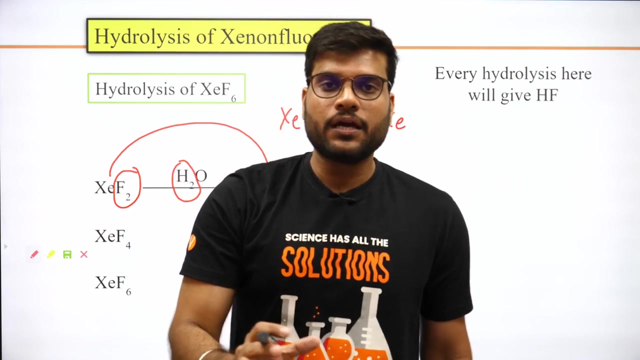 We do this At that time. the topic was made 5, half an hour ago. Then a baby will suddenly fall and ask a question of a topic half an hour ago. Now, first of all, ask yourself the question honestly: Is it the right time to ask a question yesterday or half an hour ago in the class? 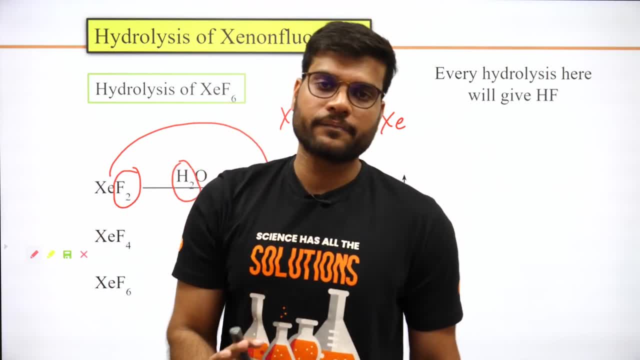 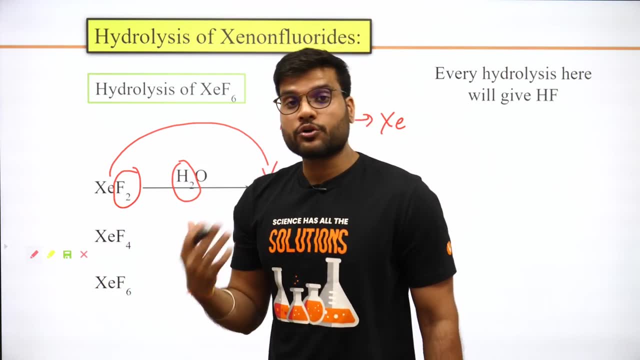 What does it mean? Understand? This is諾 sta Ji, Jied Ji. It's not there. You keep asking the same question. Stop. And the funny thing is, you are disturbing others. you are disturbing the teacher too. You think to yourself: are you paying attention here? 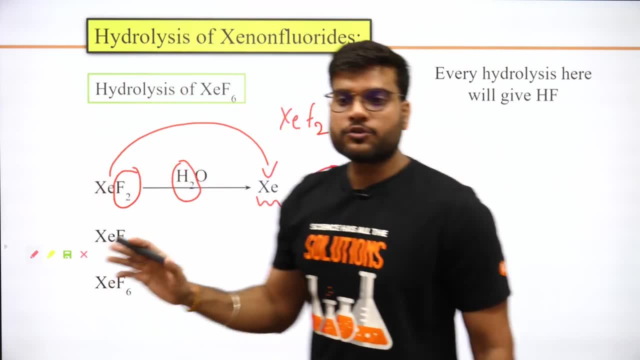 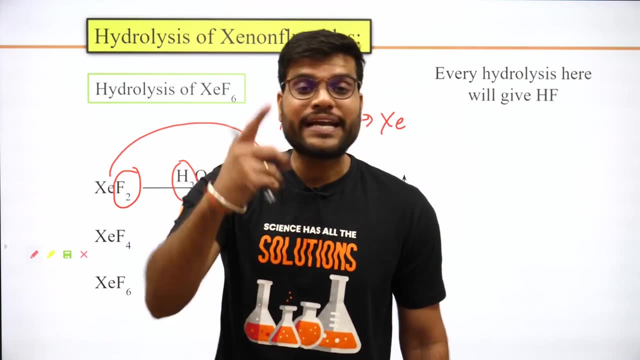 Because of the clathrate, the question that you are having. because of that, you have left the important chemical reaction, which is really of number 4.. That's why you don't get the rank. Why don't the kids get the rank? Because the kids are not in the live, the moment. 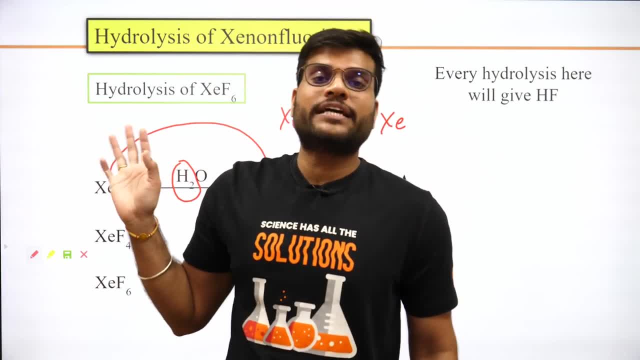 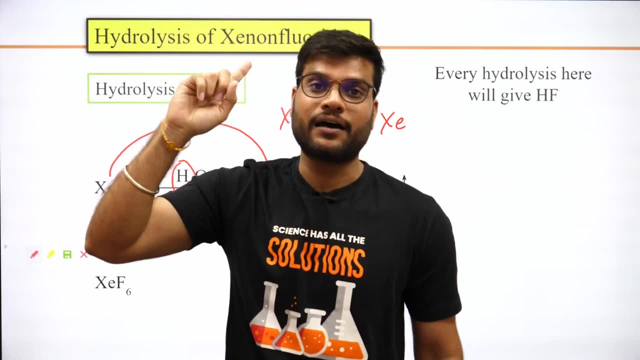 Means. you don't have to pay attention to what is going on right now. What do we have to pay attention to? What happened yesterday? What did you study half an hour ago? What question is going on in my mind? This is not the reason for selection. 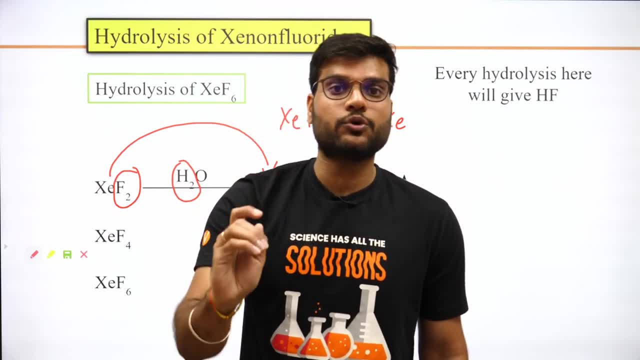 And this is true, the selection of the topper. Why is the selection of the topper? Because it is live. the moment Means it is focusing on what is going on within the moment. This is the biggest thing about the topper. 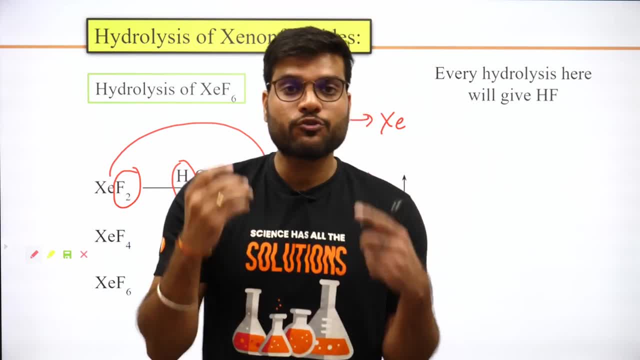 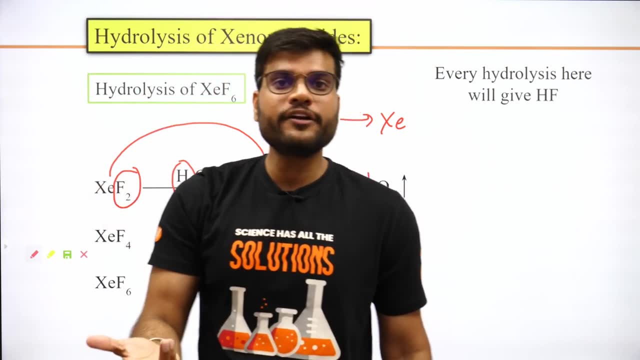 which you should learn. Pay attention to what is going on. right now, You are asking the question of the clathrate When the clathrate is over. it's been half an hour, So think of it. How will you do it? 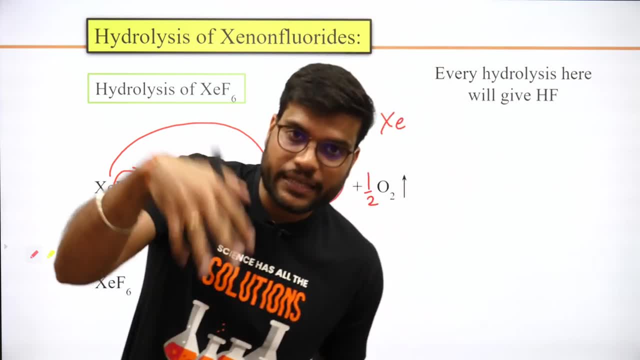 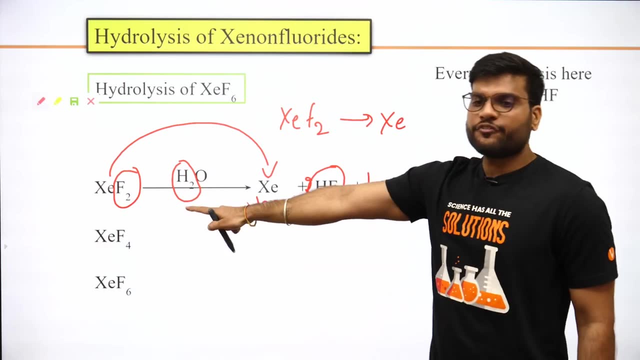 So change your habits. In this moment. what is going on? you have to focus on that. Okay, So check here. What is happening here? If XEF2 reacts with water, then it is visible that two hydrogen and two fluorine HF will be formed. 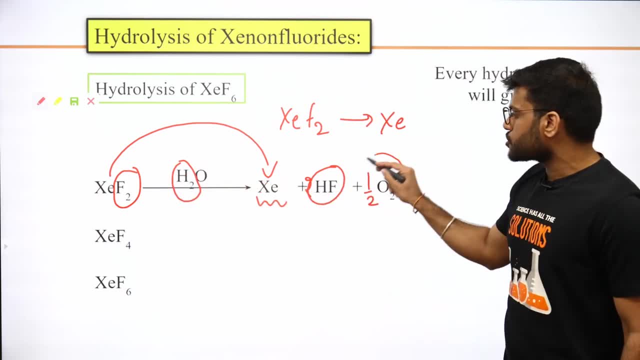 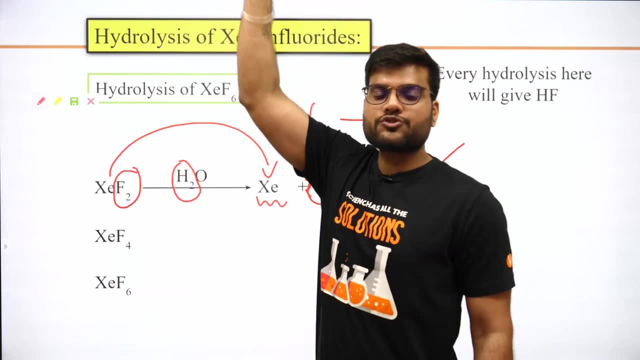 XE will come out separately And the O that is visible here will come out in the form of oxygen. Balance can also be done easily. This first chemical reaction is over. Did everyone understand, Yes or no? Hey, I am cold. 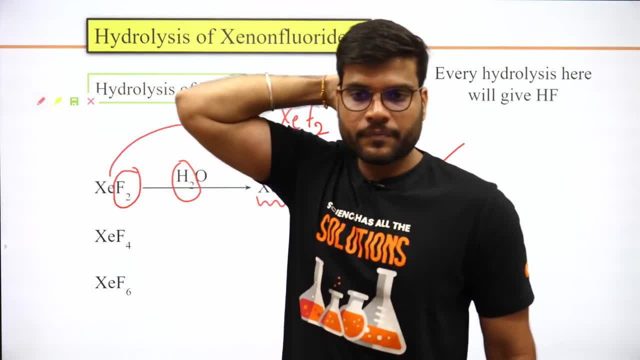 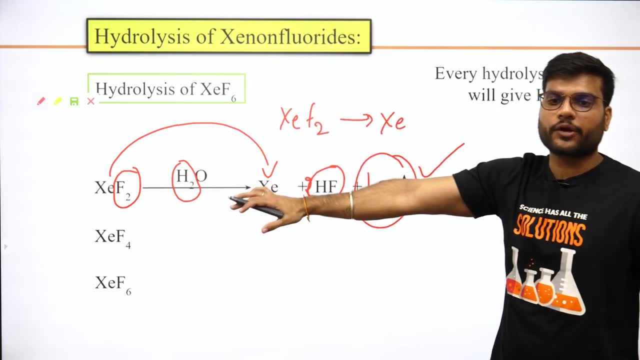 I stay like this: Yes or no? Did everyone understand? Yes or no? Did everyone understand? Let's move on to the first chemical reaction. So the XEF2 one is over. Now let's move on to what will happen in XEF4.. 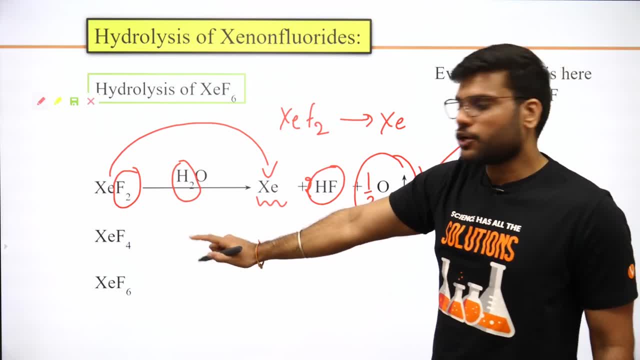 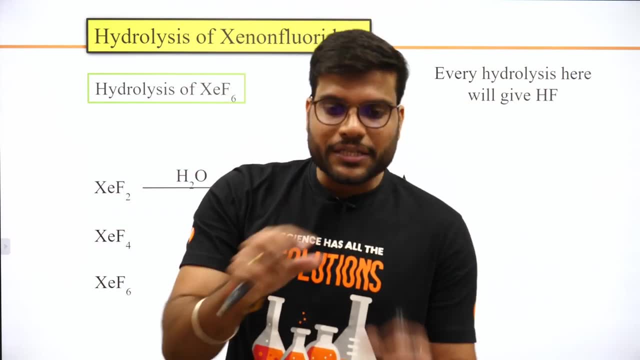 We will check that. Okay, Come on Now. next Somebody is saying: sir, you said so much, You should have given the answer, So I have written such a big statement of yours. I could not even read what was written in the chat. 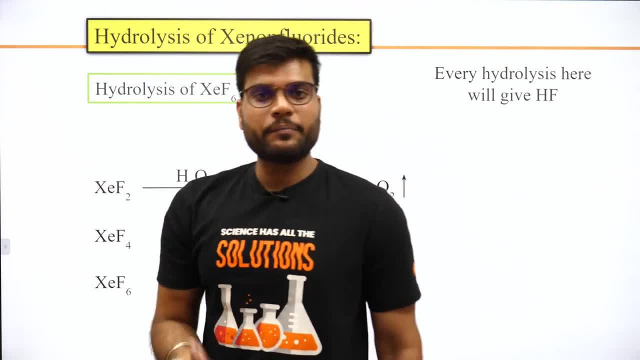 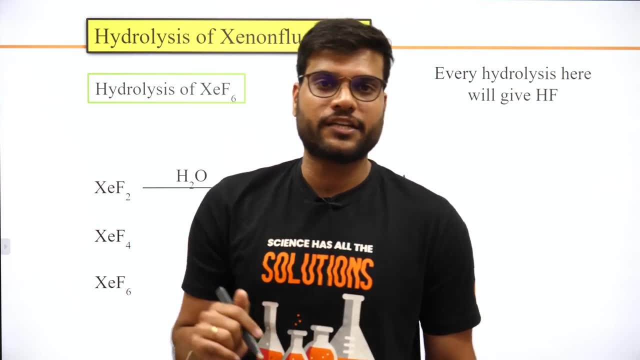 I just saw this much I had written clathrate, So you also understand my helplessness. children, It is very easy to speak. It is not so easy to stand and read in a live session. You have to see everything here. 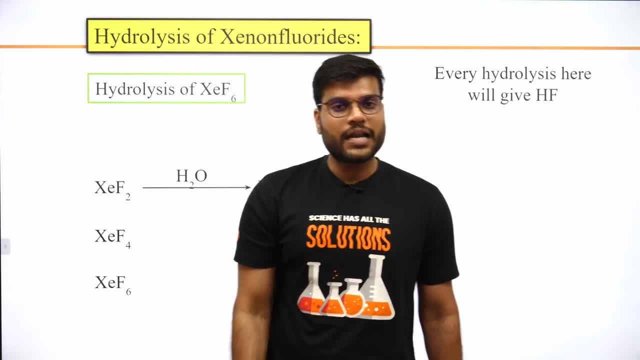 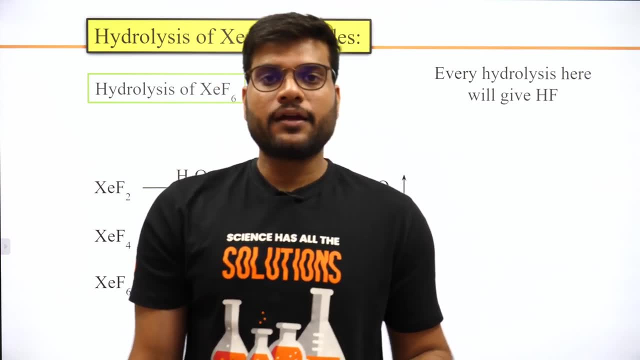 But I am not saying this. I will not answer your question. Assume that, even if I go, you have mail, You can message me. Some people also have my number. Let's call directly, Okay, And you don't have me? 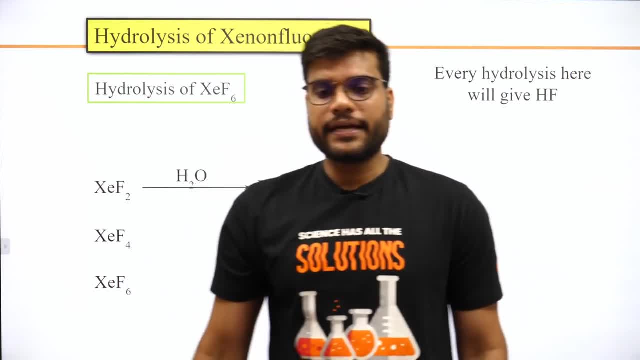 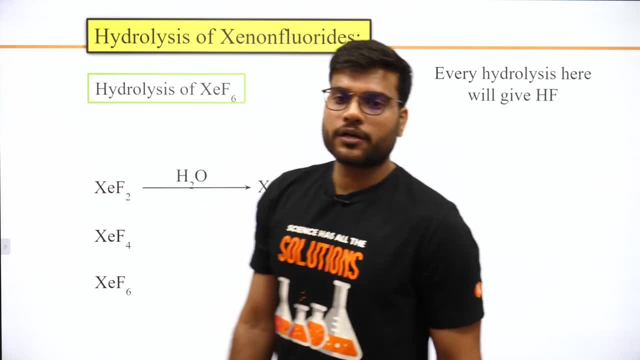 Nobody is there. Google will give the answer. Why are you scared? Okay, Come on, Come on, brother, brother, brother, Come on, let's move on. Come on. What do we have next? XZF4.. So let's go to XZF4.. 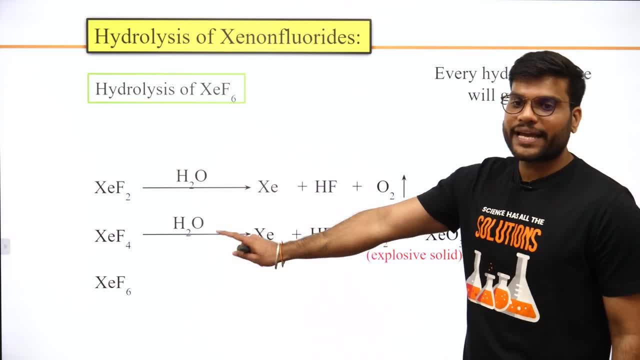 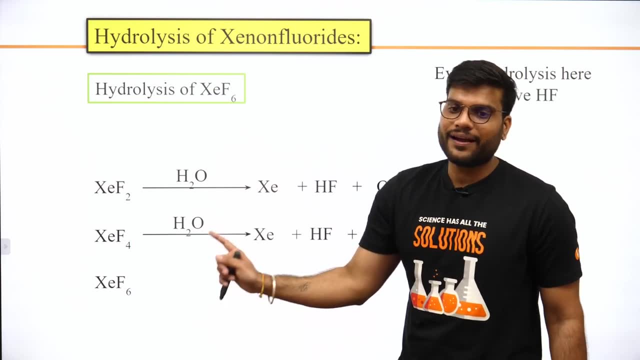 If you have done hydrolysis of XZF4, then again see what is happening here. Here I had told you XZF4 will make XZO3 extra thing. What will it make XZO3 extra What I had told you? 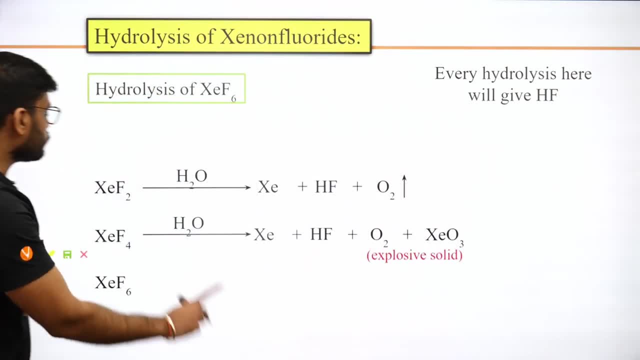 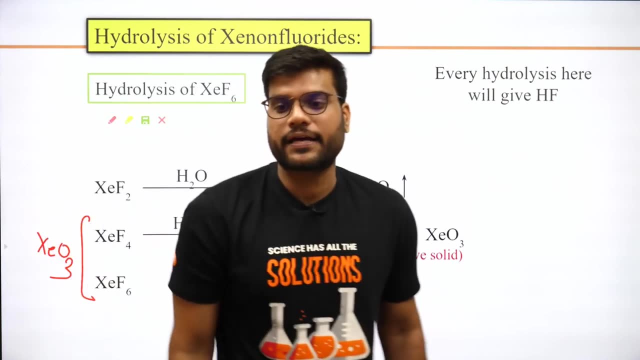 It will make. Just check. This is very important. XZF2 is the only one that does not make XZO3.. Apart from this, you will see both of them making XZO3.. Note down I had already done this. 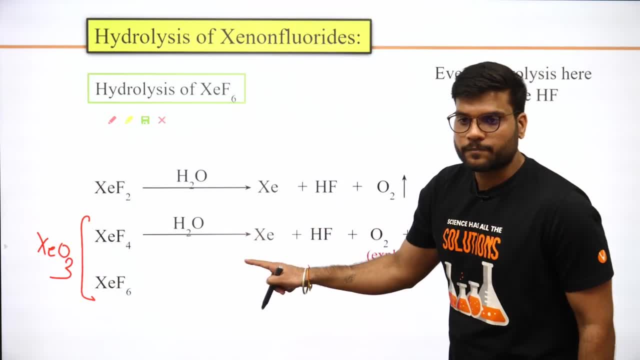 So here, If you do the reaction of XZF4 with H2O, So in that case- see The upper compound- is common. It is also making all the compounds. Just check, See The method of remembering. The upper compound is also making this. 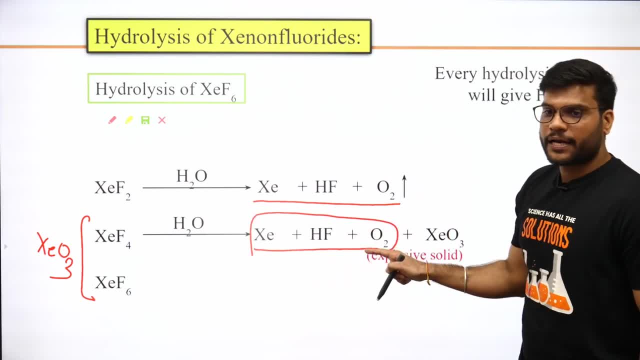 But it will make one extra. Why? Because it has a responsibility. Why Because it has 2 extra fluorine. So what is it doing here? Just check, It is also making XZO3.. And what is this? It is explosive solid. 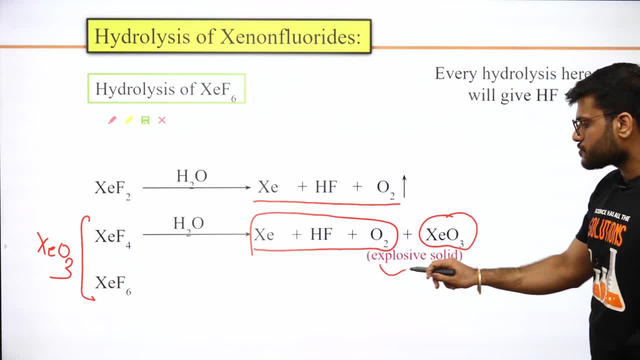 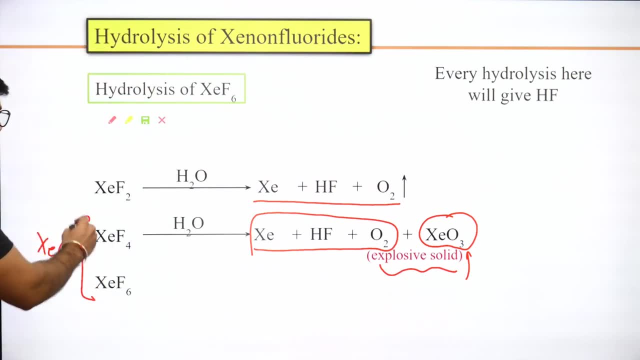 Just check, XZO3 is explosive solid. You note down it right now That brother, the upper one, is making all the compounds together. And what is this? It is explosive solid. Just check, XZO3 is explosive solid. So the upper one is making all the compounds. 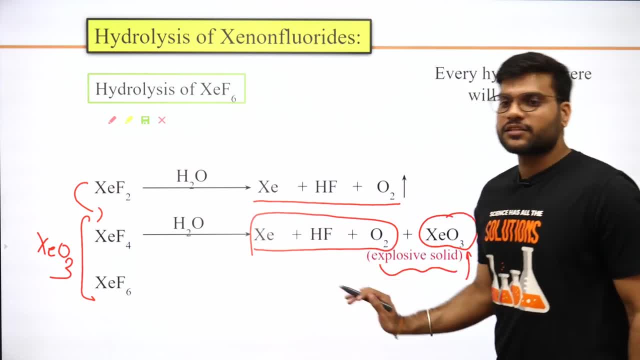 It is a big brother, So it is doing all the duties of the younger brother, Means it is making all the compounds, But it is also giving one extra, Do you understand? So this is very important. Write it in your chat section right now. 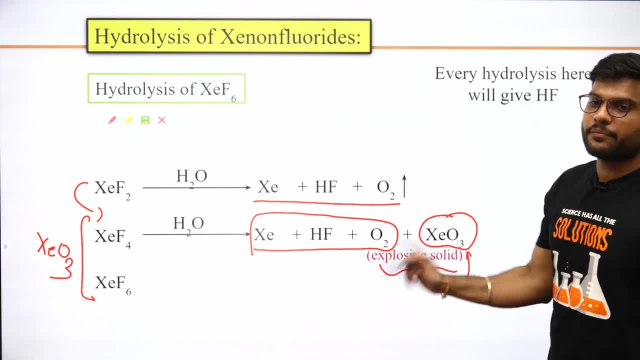 Brother, it is very important. Write it, It will be useful. So XZF4: by doing the reaction with H2O, It makes XZ, HF, O2.. Which makes XZF2 also, But it actually gives XZO3.. 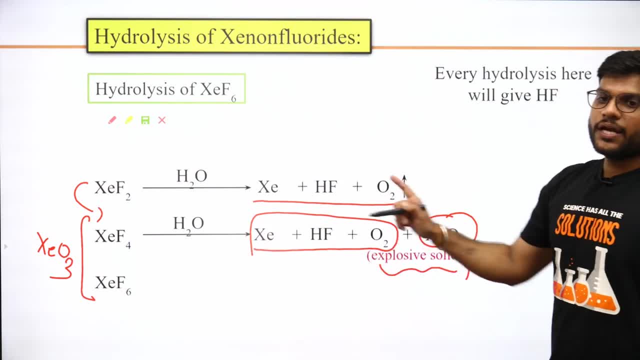 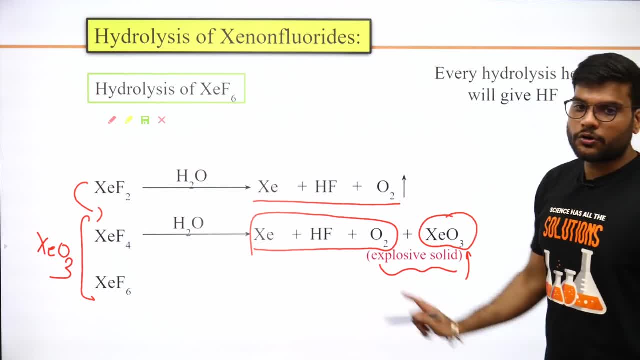 Who else has written dear children? Who else has written Biomolecules will start uploading now, Don't worry. Neha has written it And Keshav Pathak has written it. No write, there is no use. This is a question of four numbers. 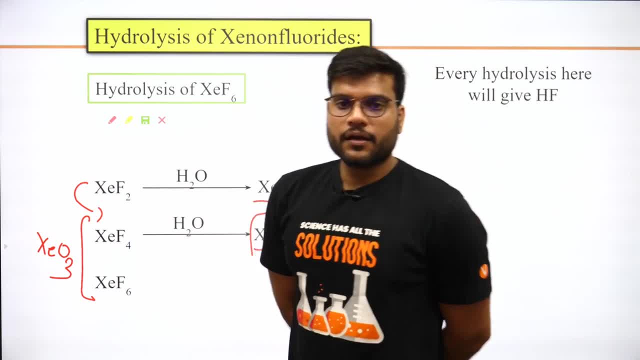 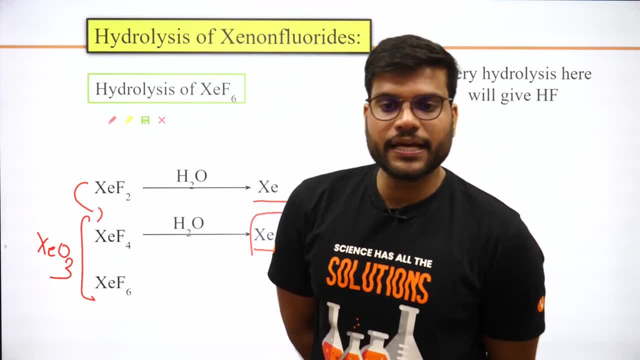 Write, Write it now. The question of four numbers is coming. Sonam Katiar has written it. Explosive, Ex-pulsive. This, This, This question is also of number 4.. It is explosive, solid, So this. 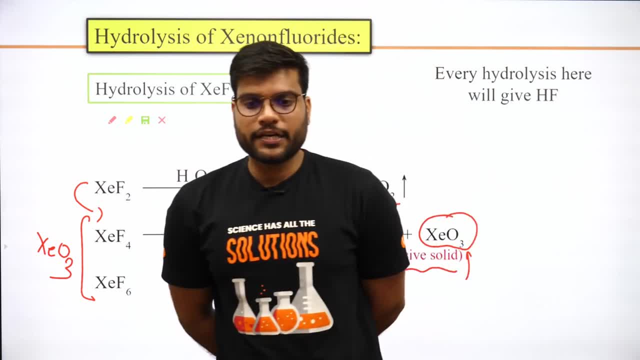 It is explosive solid. This. So what? This is explosive solid. It is explosive. take a look, This is explosive solid. take a look, These are explosive solid. It is explosive solid. It is not expulsive, it is explosive. 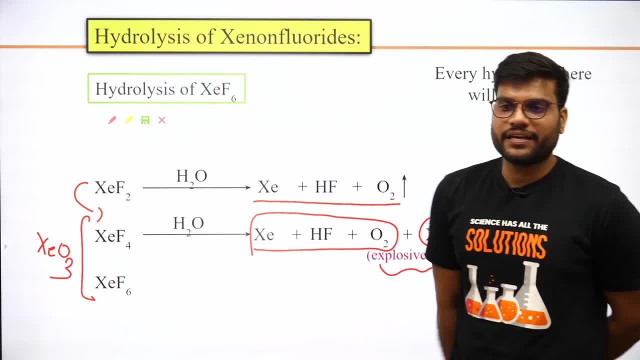 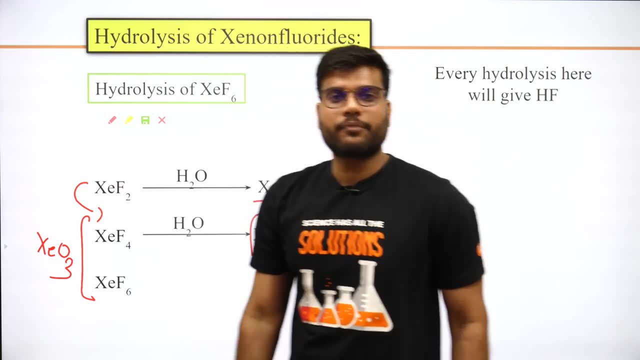 Now we will move towards the last chemical reaction. What does XZF6 do? We have to check that. Rest of the things are with us. In fact, I have already shown you the chemical reaction of XZF6.. It will make only two compounds. 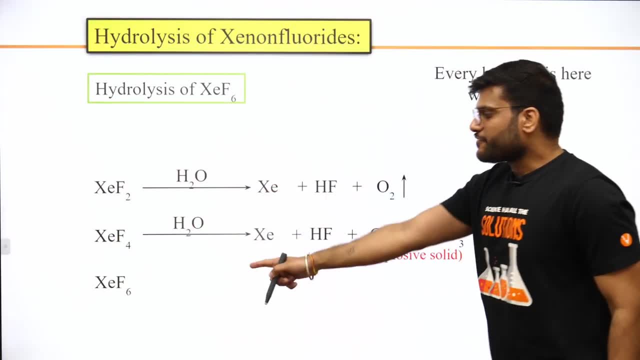 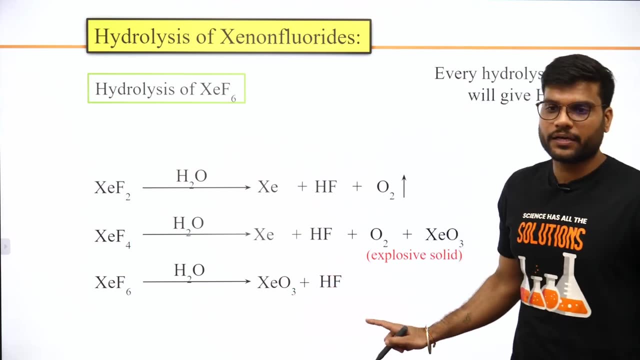 Check XZO3 and HF. XZF6, this is Birla. I have already shown you its chemical reaction. If you have reacted with H2O of XZF6, then it will make only two compounds: One is XZO3 and one is HF. 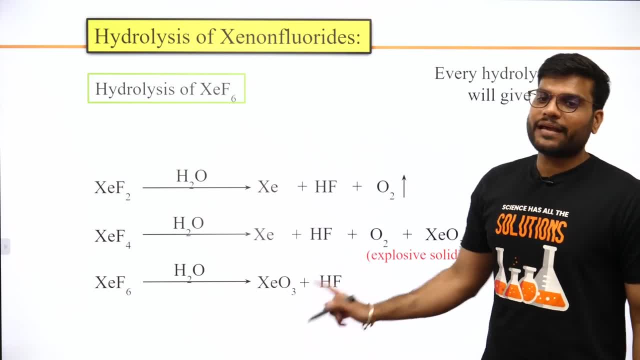 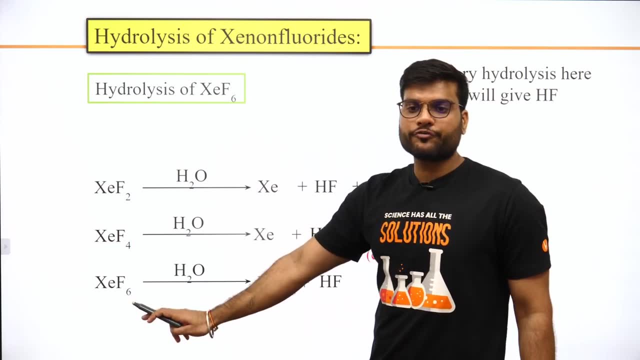 This does not give oxygen And this is a very important chemical reaction. I have already shown you the chemical reaction of XZF6.. This is the easiest way to remember. Two hydrogens and two fluorines. Keep removing them. HF and XZO3 will be formed. 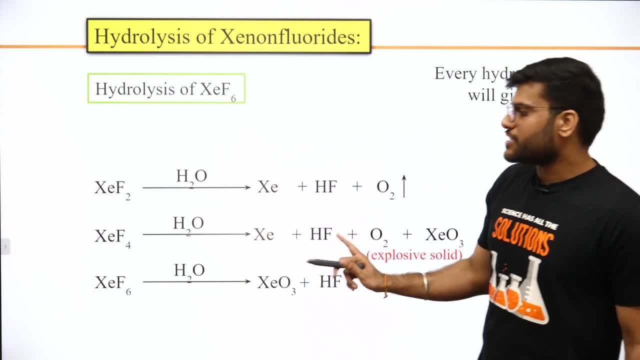 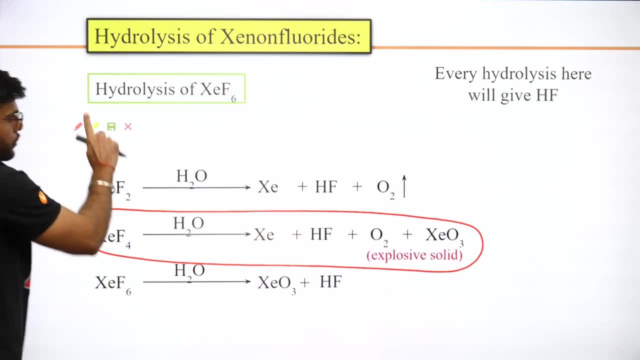 Nothing else will be formed In the upper reaction. if you ask me which is the most important reaction, then it is the middle one. This one is very special Because it is giving four compounds by beating the upper and the lower one. And this question is asked many times. 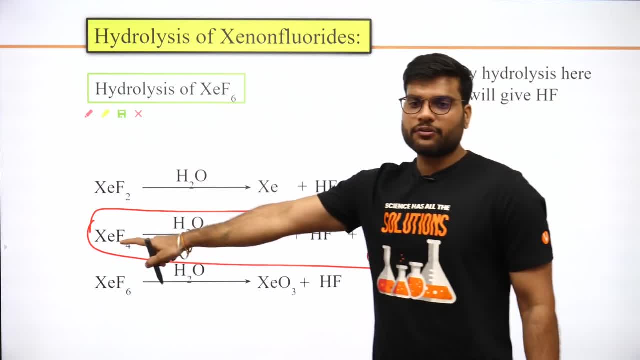 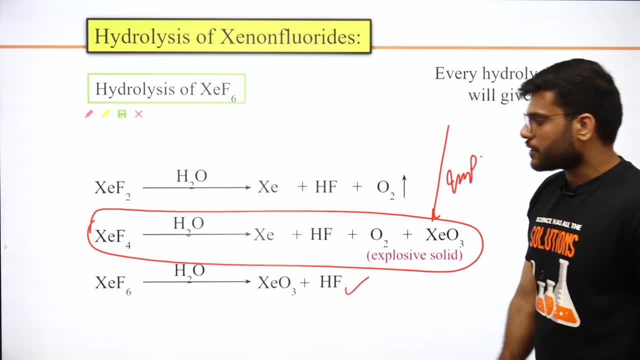 Now, this is really very important. The question of hydrolysis of XZF4 is asked every time And I tell you that please note it down. And all these are chemical reactions. I have already shown you this. I will also show you. 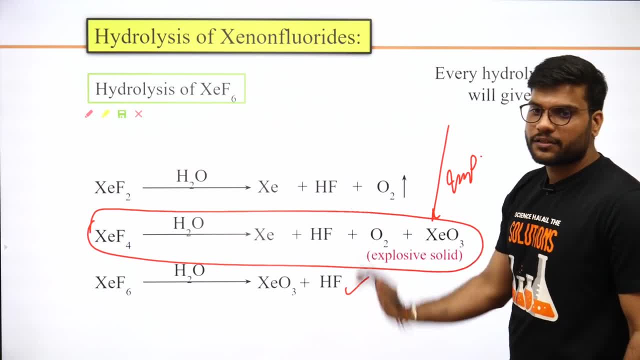 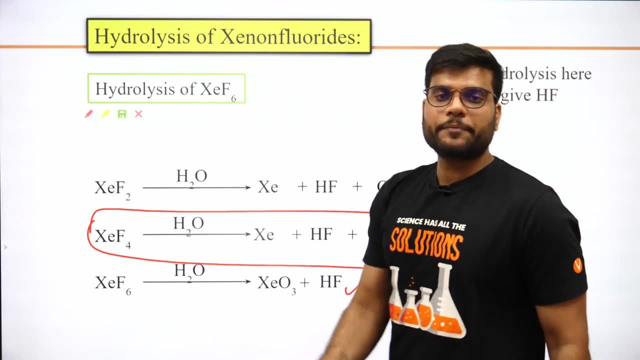 I have already shown you this. It will make only two compounds. This will give four and this will give three. It is very important. Okay, Did everyone understand? Very good, Very good, We are at the landing point, After that, group number 18.. 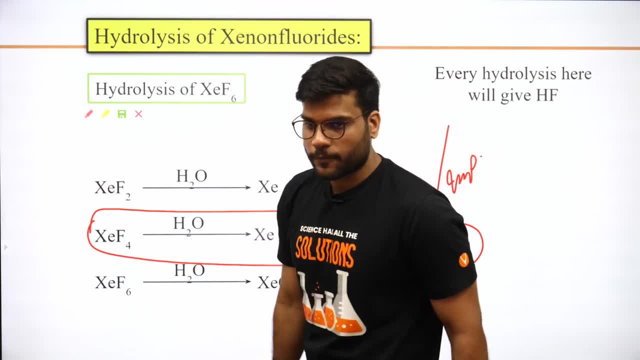 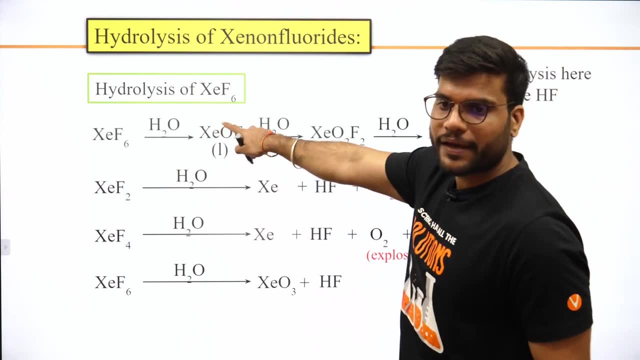 First A Finish. Come on, Now let's move ahead. Come on, So how to make a compound in XZF6? I will check you again in its sequence, Because I have already shown you. Please check. XZF6 will make XZOF4 with water. 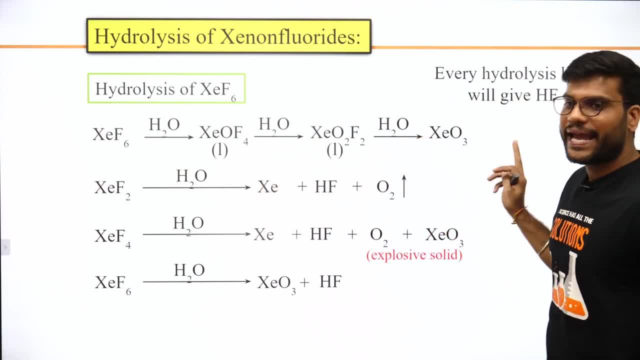 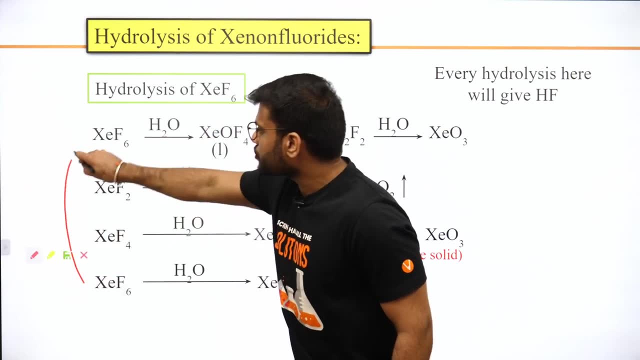 Then it will make XZO2F2 with water, Then it will make XZO3 with water. Every time it will take out HF. This is the chemical reaction Which you can compare. Actually, they are complementing each other. This is the chemical reaction. 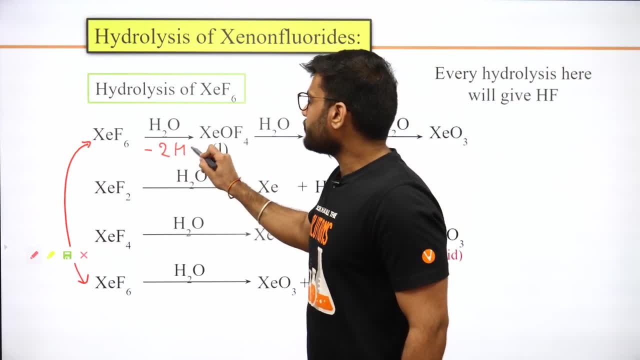 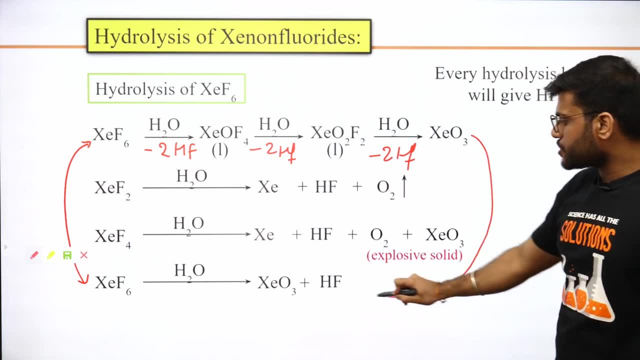 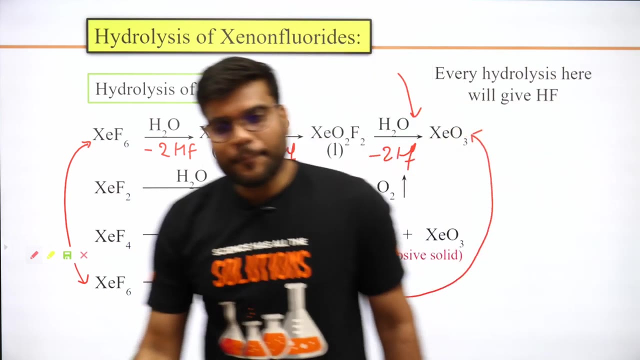 And here always, two molecules HF will come out, Two molecules HF comes out, Two molecules HF comes out, And this and this chemical reaction are same. Alright, This is told. This is overall, Everyone understood. And here our 4 number, if you remember. 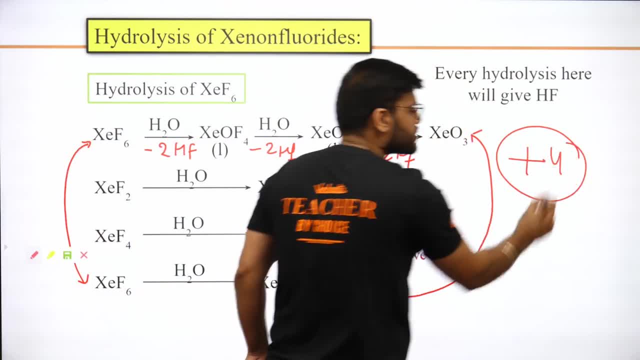 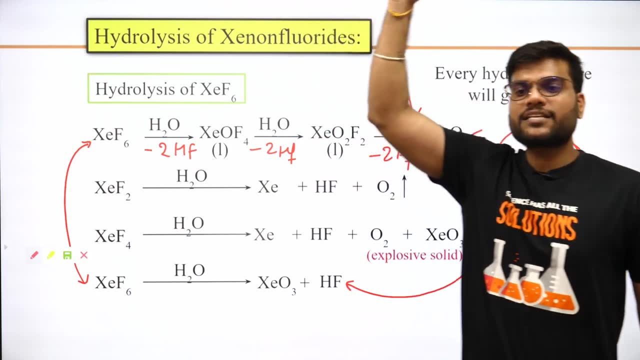 4 number has been confirmed, Plus 4 number has been confirmed. if you remember the chemical reaction, Who all have remembered, To whom all the 4 numbers are confirmed, Tell me Write. Yes, Yes, We remember, our 4 numbers are confirmed. 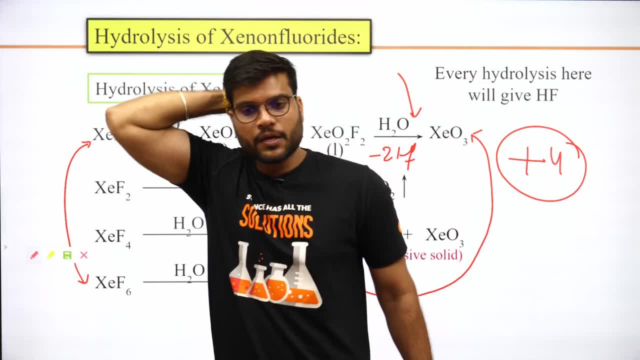 Who all have their 4 numbers are confirmed, Write me. Who all have the 4 numbers made here. Who all have the 4 numbers made here, have made here, Who all have remembered here. We will do the last slide and after that we. 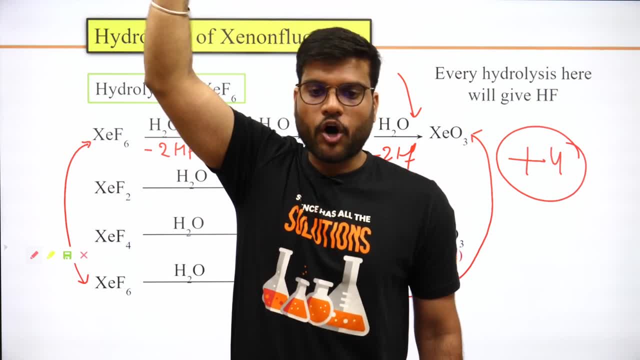 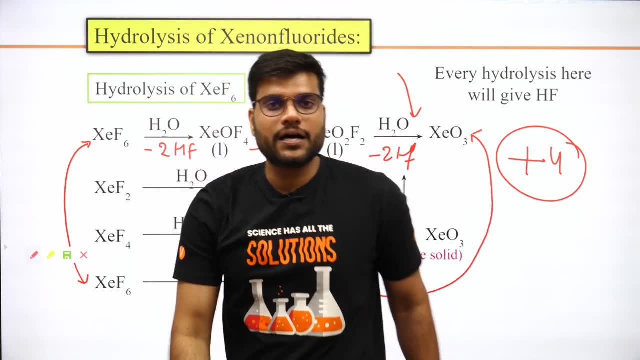 will finish, Are you sure? Number 4.. Very good, my dear children, Those who are watching right now, you can write in the comment section that, yes, I remembered Those who really understood that, yes, everything was going well, Very good. So I will move towards the last slide. 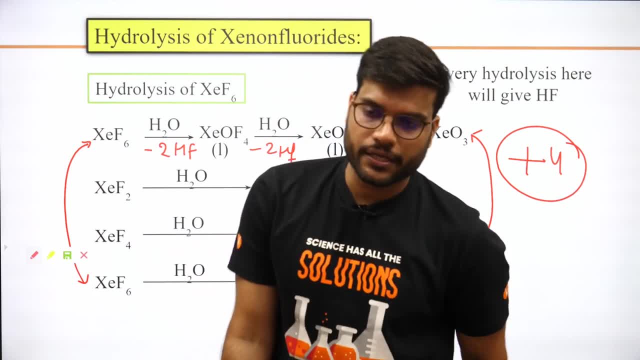 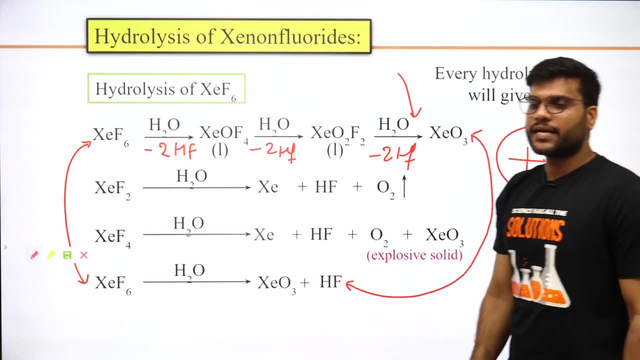 I will tell you the last three chemical reactions, which are excellent and easy. Just check it and after that we will finish our group number 18 first. So here we will move forward. Take a screenshot. Take a screenshot 1,, 2,, 3,, 4,. 5 is very important. Take a screenshot 1,. 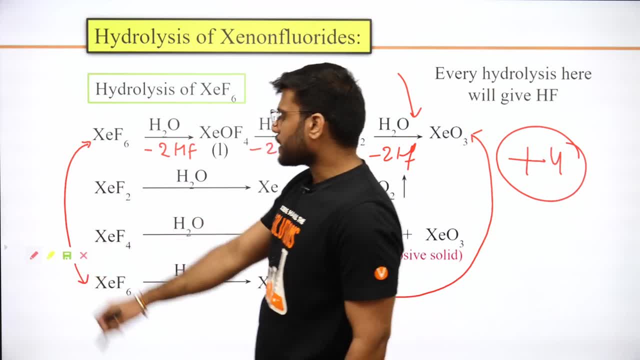 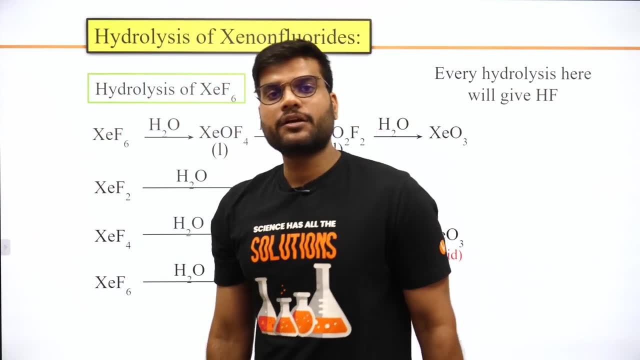 2,, 3,, 4, 5.. Take a screenshot. Let's move forward. I am removing it. Last sort of chemical reaction. After that, it is over. It is enough. 18 number group is over. It means people are. 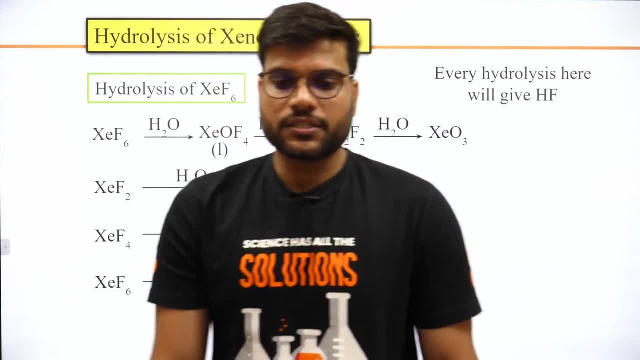 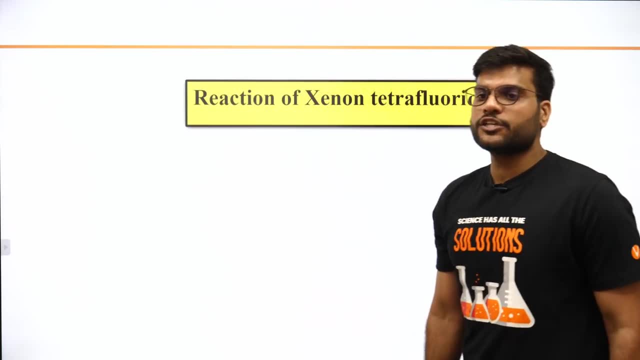 over. After that we will start the new chapter. Last, Are you ready to see the last chemical reaction? Let me show you the last chemical reaction. Look, brother, Reaction number 18 of Xenon tetrafluoride. Last, because I had told you that tetrafluoride is very important. 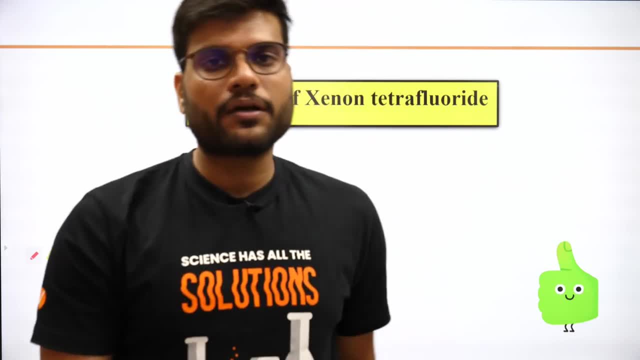 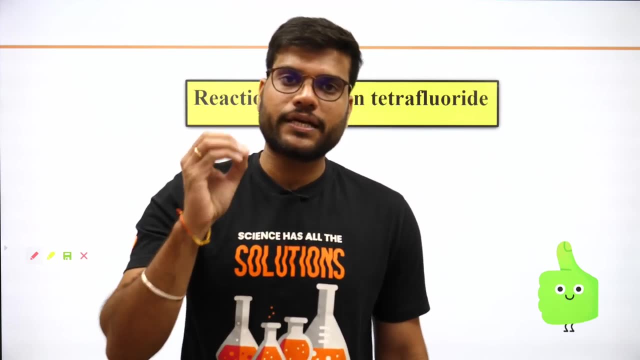 here. So I will show you the chemical reaction of Xenon tetrafluoride. Actually it makes complex compounds here. It is very interesting How to remember that is also very simple. I will also tell you. But again I am writing those three chemical reactions again, Just 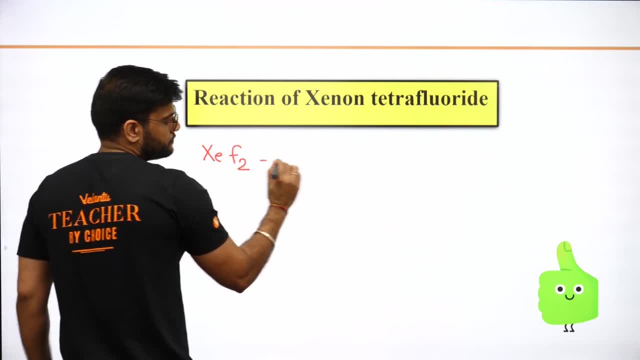 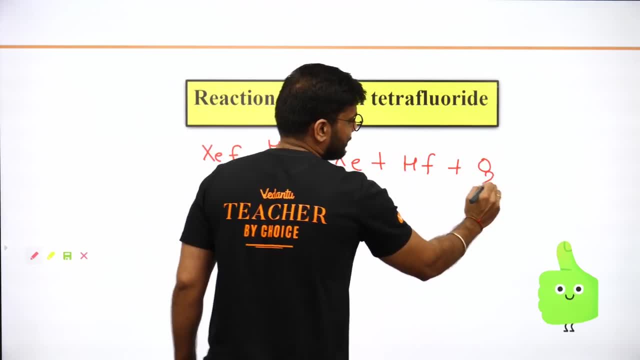 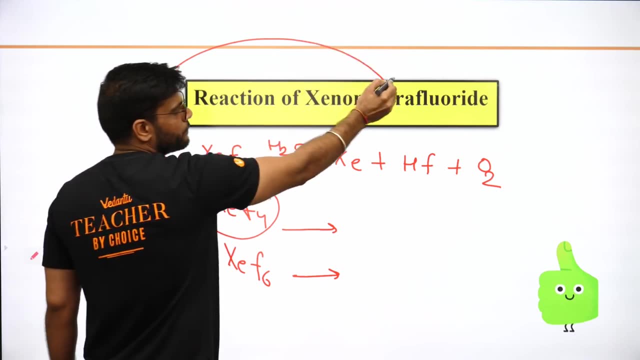 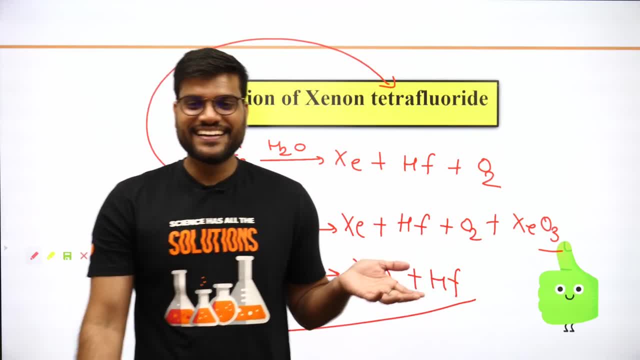 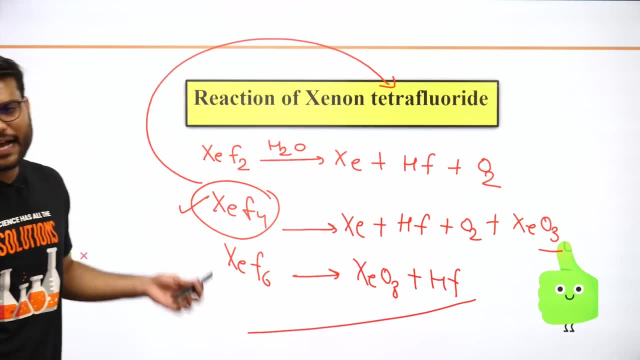 Remember, Remember. Everyone is happy. son Dhani is saying that I am happy, Everyone is happy. Today's vlog is ending. Okay, Come on. Finally, one is over here. Now let's go Note down this. 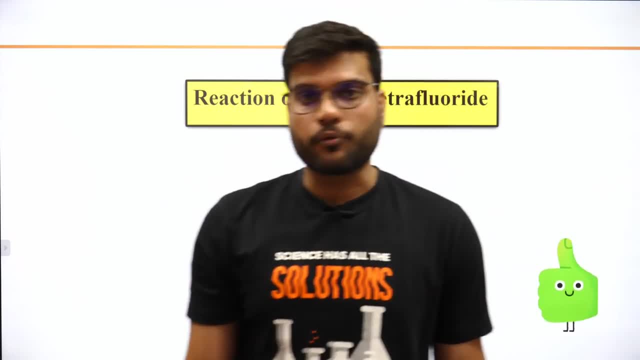 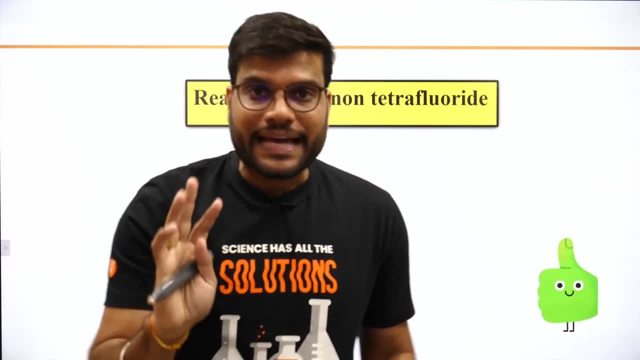 Towards the last chemical reaction. Now here he makes a complex compound, which is very easy. What will XEF4 do Every time he donates a fluorine And makes a complex PC? What I am saying, you can check it. 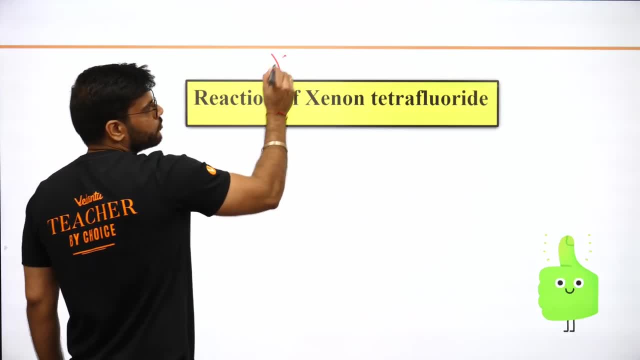 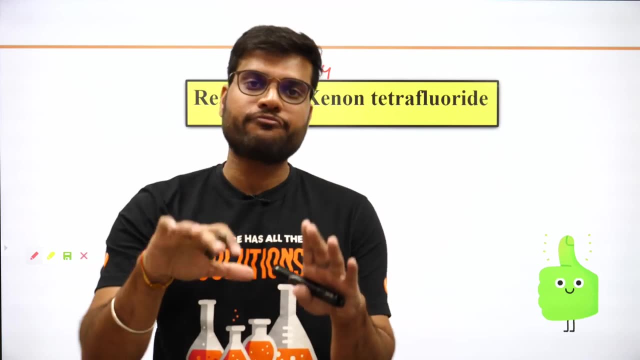 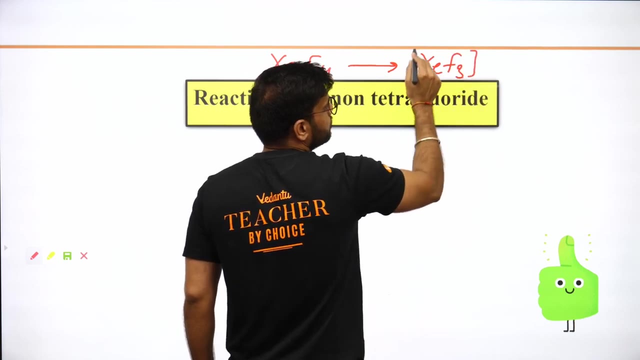 I am just saying this: Xenon tetrafluoride, XEF4.. Every time, whatever species will come in front, he donates an F- And he converts into what- XEF3- He will make such a compound. 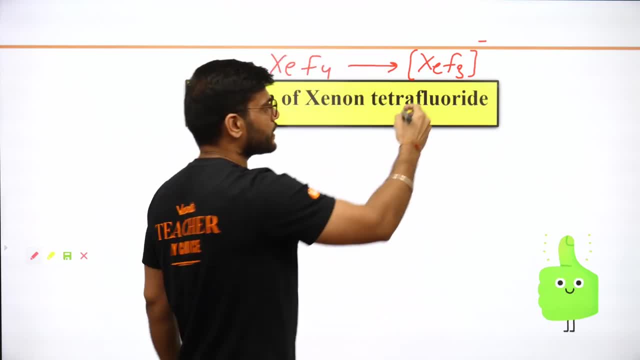 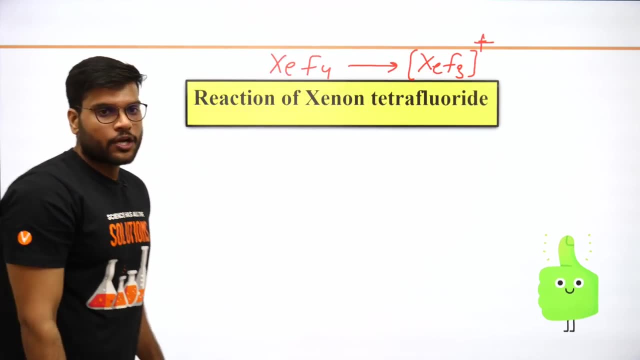 And he donates one fluorine to the front, Not minus but plus Because F- has gone. So this compound is a complex compound. It is a simple way. Now I will show you how it happens, So you just check. 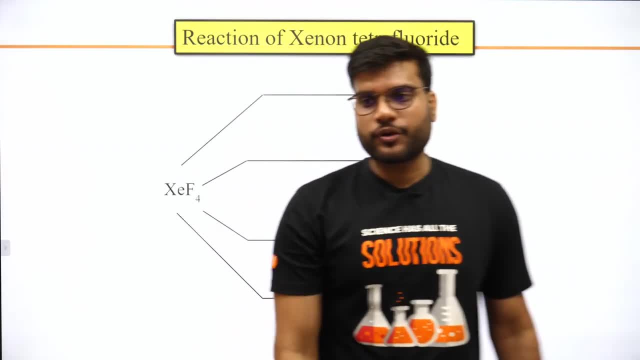 I am removing it. Okay. First reaction: Xenon tetrafluoride. Xenon tetrafluoride. There are only 3 reactions. There are 4 reactions And it is the same Every time. what will he do? 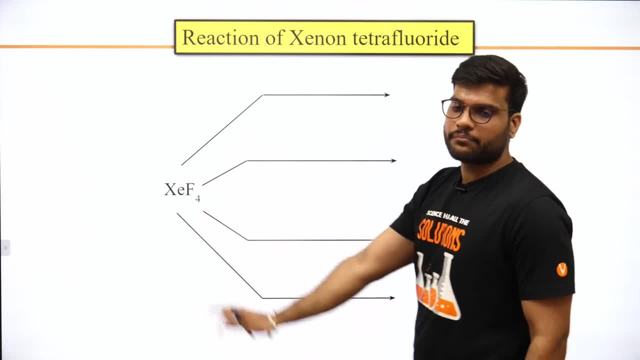 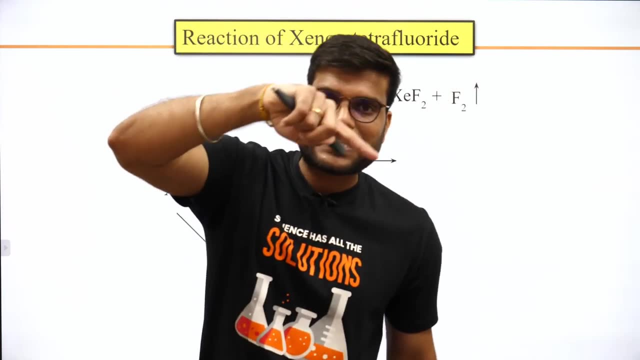 Every time he will release XEF4-1F-. That's it. So now you just check. Okay, There are more chemical reactions. Oh my God, I forgot There are 2 slides, So you have to put that in the next slide. 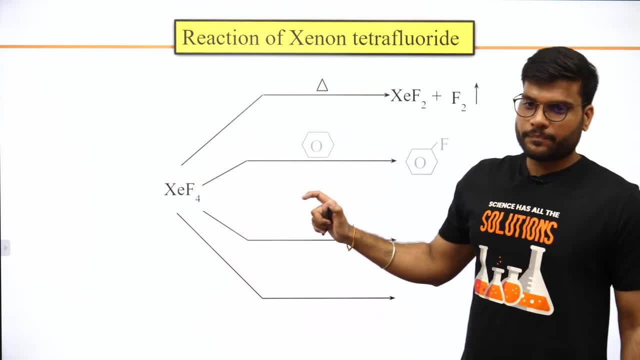 Okay, Now we will check this, Just check. If let's assume There are 4 more reactions, Let's read extra: Okay, There are 4 reactions. Are you guys ready Write these 4 reactions, These 4 reactions. 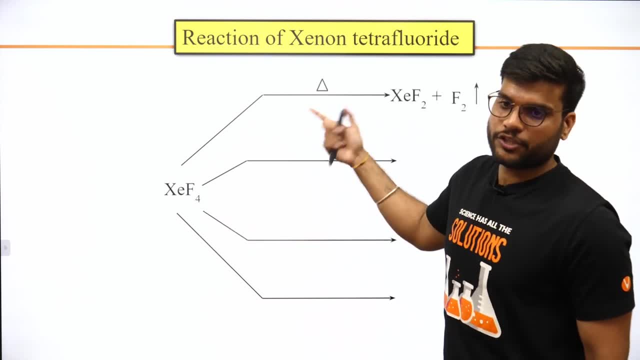 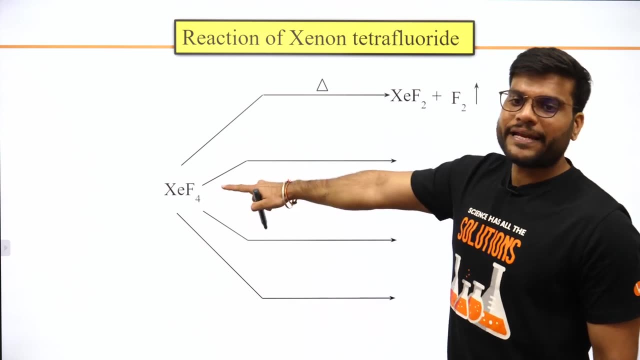 Let's assume that you have heated XEF4. So what will happen? if you have heated it? 1 fluorine gas will be released from here. It is very simple, Note down: If you have heated XEF4, then 1 fluorine gas molecule will be released from here. 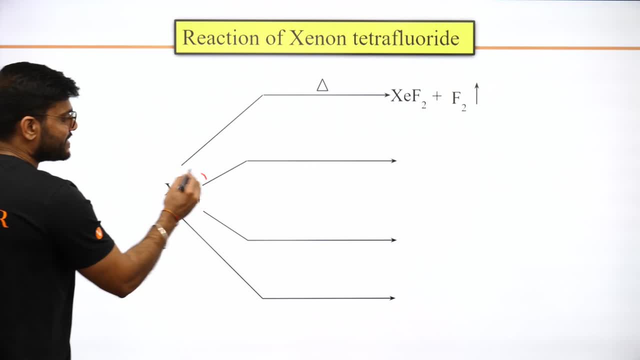 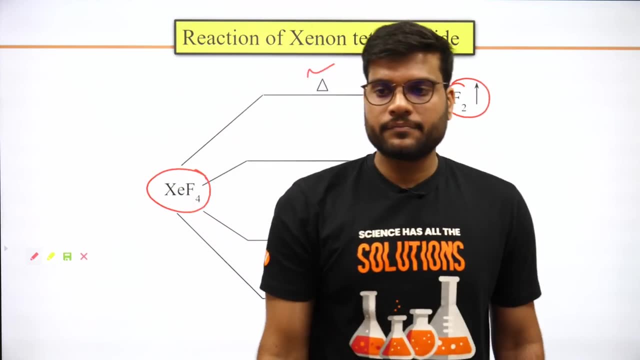 This is very important. Just check, See this XEF4.. If you heat it, fluorine gas will be released. XEF2 is saved. It is very simple. It is very simple. Remember, Write it all. If you heat XEF4,. 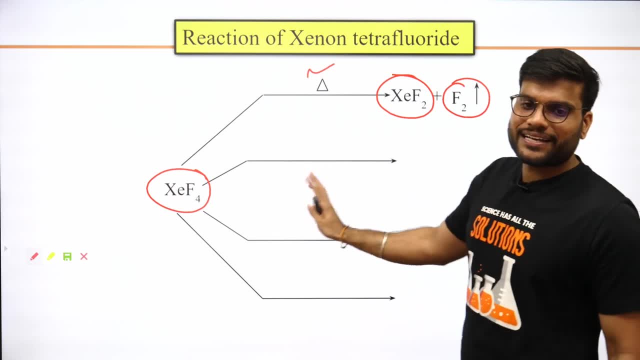 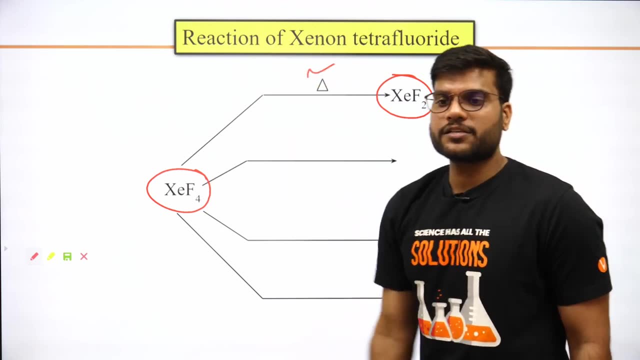 then XEF2 and F2 gas will be released. This is a very simple chemical reaction. Even a kid will remember it. Remember, You have released fluorine gas. I am moving towards the second chemical reaction And I tell everyone who is studying: well, 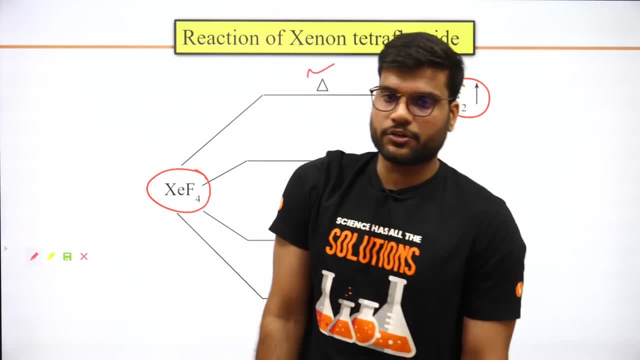 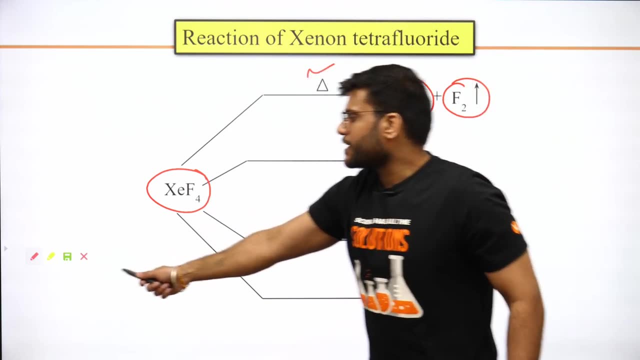 I tell everyone that please write this in the chat section. If you don't write, then there is no use. You won't enjoy it. Okay, So keep writing. The first chemical reaction is easy. The second chemical reaction: Assume that you have reacted XEF4 with benzene. 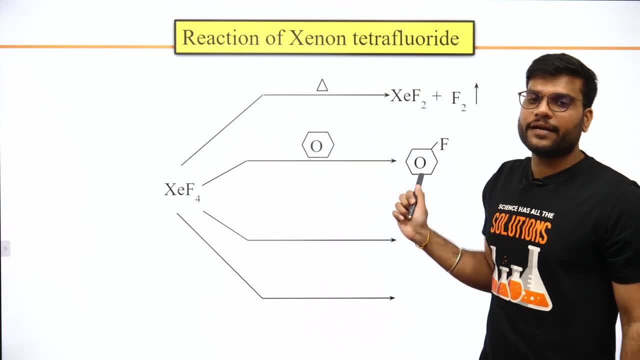 So as soon as you react with benzene, it will make benzene fluoride, Fluorobenzene, Fluorobenzene. We will call it fluorobenzene. It will make it fluorobenzene. So what is this? 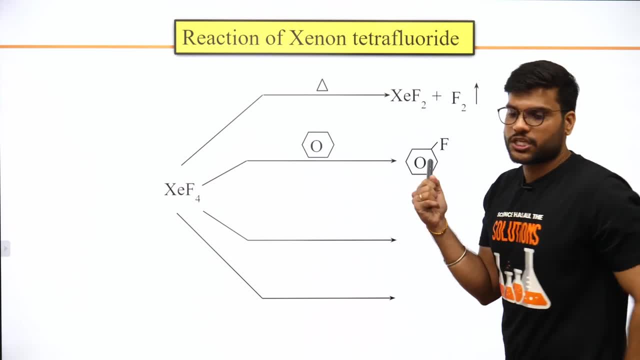 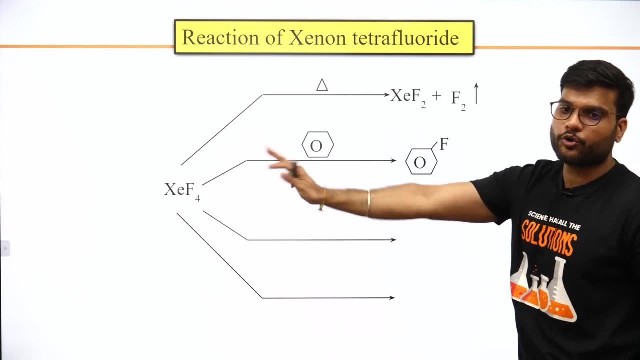 Fluorobenzene. It is very simple. This is called fluorobenzene. Write it Fluorobenzene. If you will react with benzene, then it will give F and make it fluorobenzene. Its work is to give fluorine. 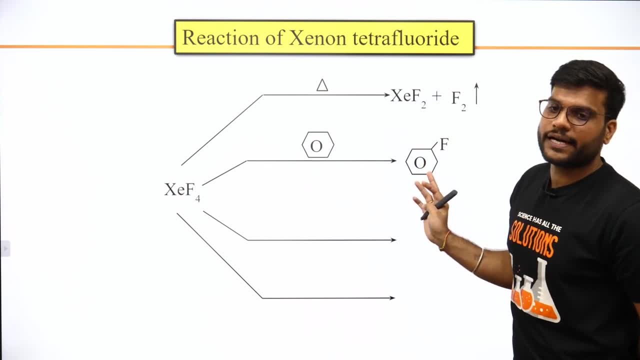 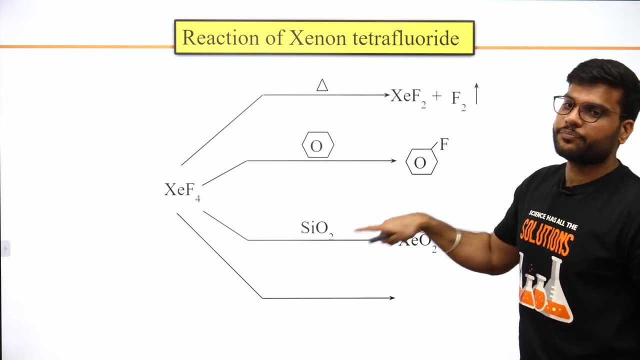 It has given fluorine at the top as well, as here It has become fluorobenzene. Check the next reaction. Assume that you have reacted it with SiO2.. And this reaction is important. In that case, as soon as you react with SiO2,. 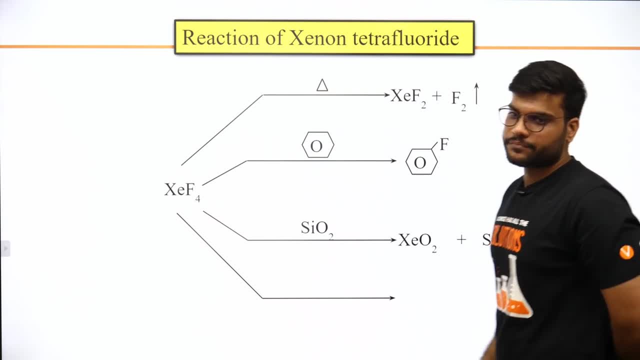 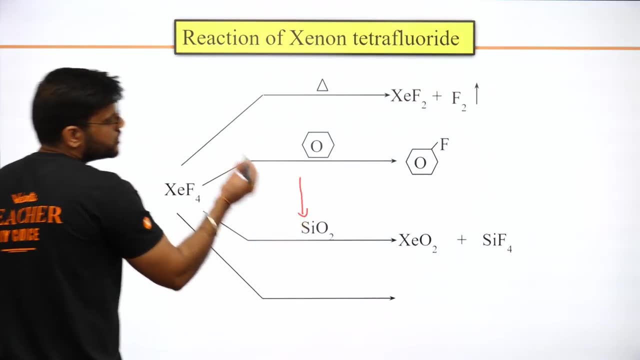 here it makes SiO2 and SiF4.. It is very important. Check it. This is very important. Look here. Everyone should know that. which group does silicon come in? Group number 14. So to complete its valency. 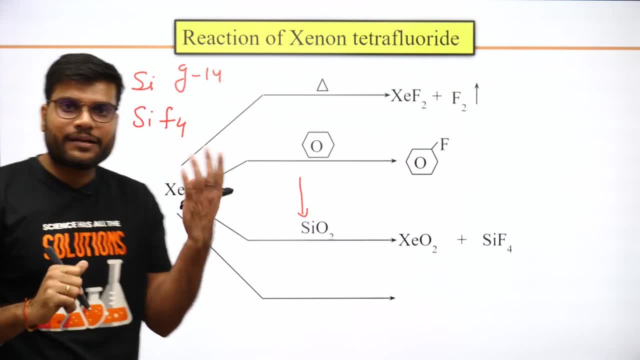 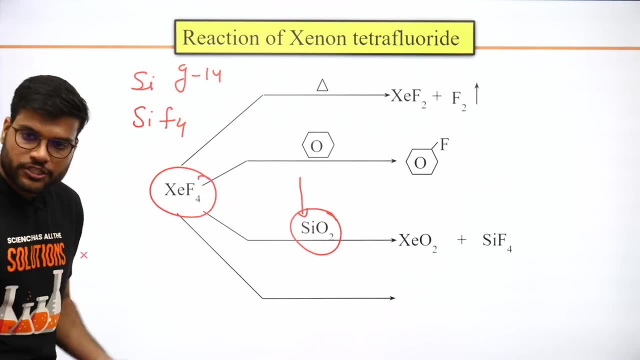 it has to make four bonds, So it will make four fluorines with itself. So here SiO2 reacts with SiF4.. Now think for yourself that it will take four fluorines with itself And it will take both oxygens with itself. 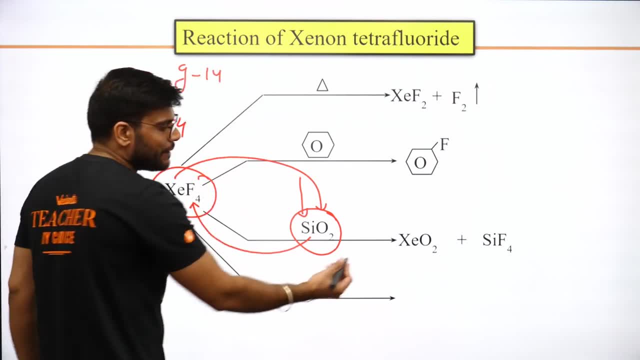 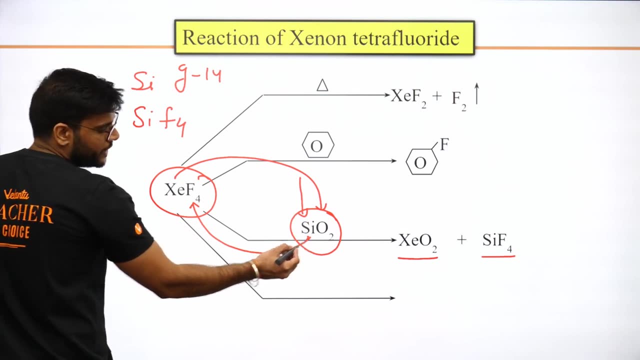 Only ion is being exchanged. So what will happen here? SiO2 and SiF4.. How easy is it? Check what is happening. Only silicon has taken four fluorines. This xenon has taken two oxygens from here, Finished. 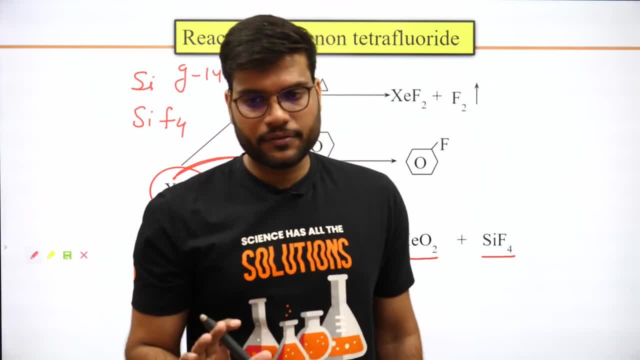 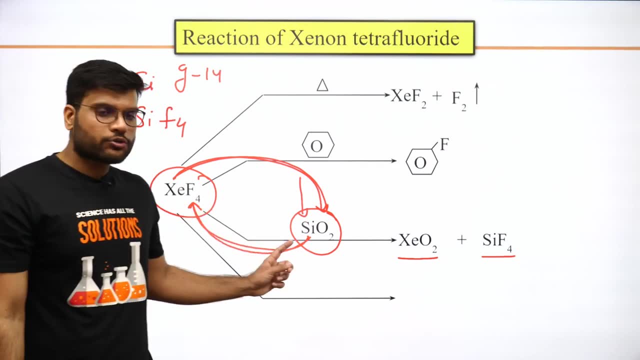 Is it hard? Is it hard? Is it hard? Write it quickly. No, sir, We got it. I say it again: SiO2 reacts with SiF4.. SiO2 reacts with SiF4.. Only ion is being exchanged. 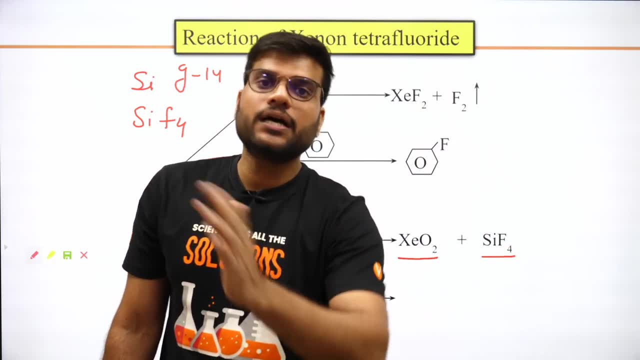 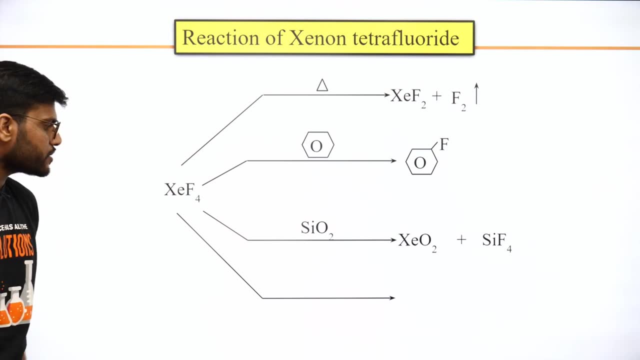 It will take silicon with fluorine. It will take xenon with oxygen. Finished, Did you understand? It is done. Now we are moving towards the last reaction. Whom are you making its last reaction with? With O2F2.. 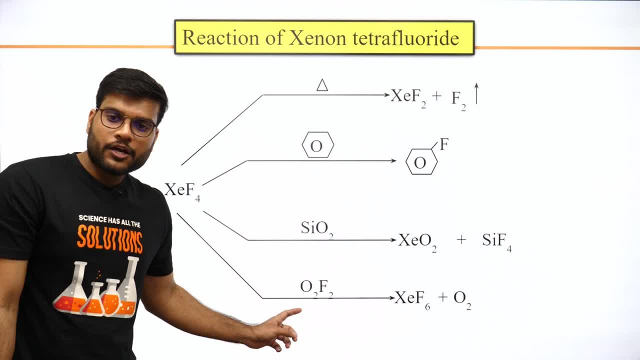 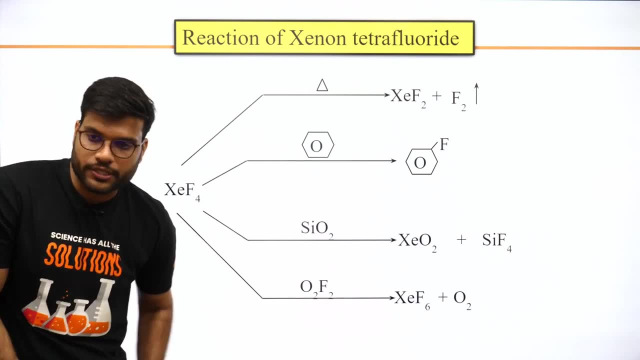 If it makes reaction of SiF4 with O2F2, then see from here What will it do. from here It will make its higher version. SiO6,, SiF6 and O2 will be released from here. This is also very easy. 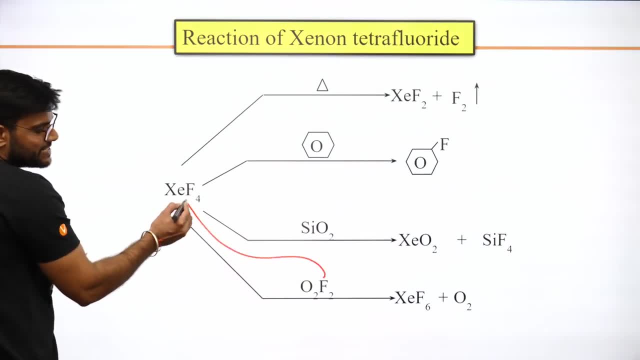 How will you remember it here? This fluorine will go with it, with its brothers, Oxygen will be liberated from here, which is very important. Just check it Okay, This is also very easy. So here, SiF4 will take fluorine and 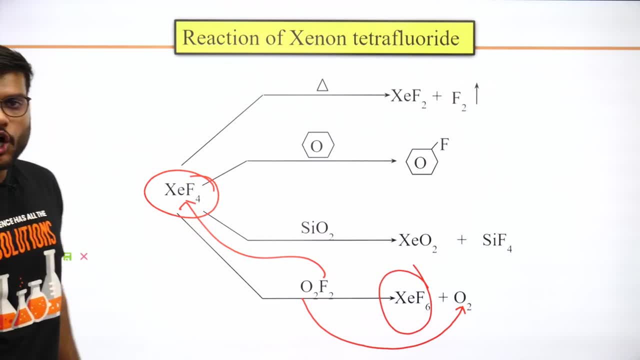 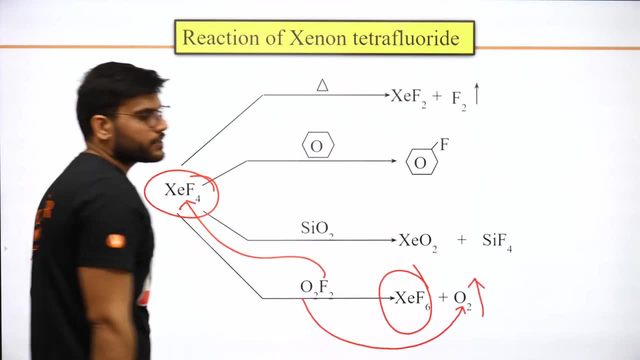 SiF6 will go towards higher version And oxygen will be liberated from here. It will be released. It will be released. It will be fun. So finally, oxygen gas comes out from here. So four more reactions have come. Did you find it hard? 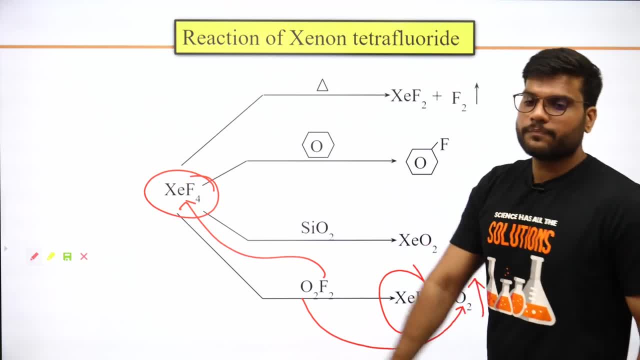 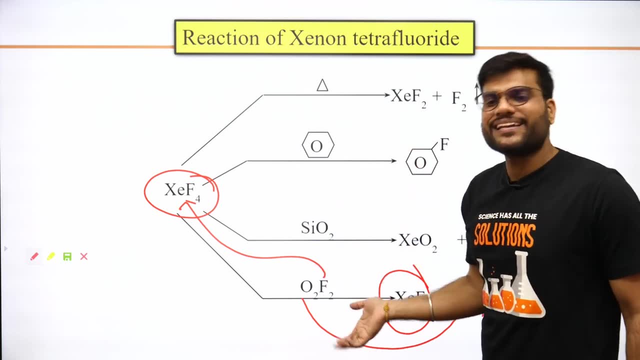 Is it hard? Write it once, You will remember it. What do I say? Heat XZF4, XZF2, fluorine out With benzene, benzene fluoride With SiO2, ion exchange, Nothing. Silicon fluoride and xenon dioxide. 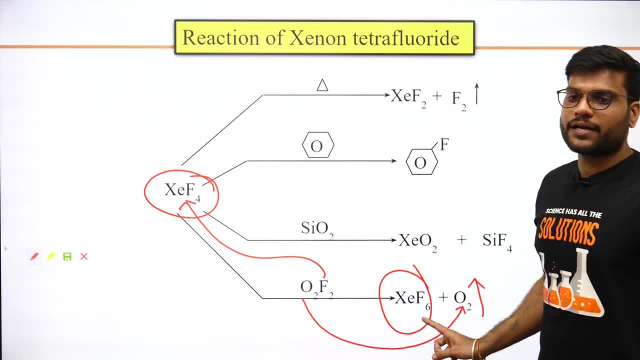 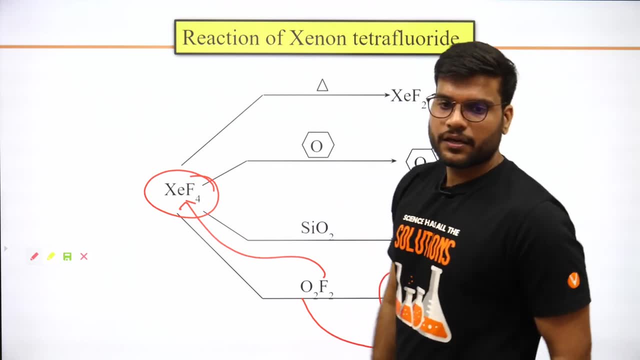 And O2F2,, XZF4 and O2F2, what are they making? by reacting together, They are releasing XZF6 and O2.. It is very easy, So easy, It is very easy. Okay, Write it once in the copy. 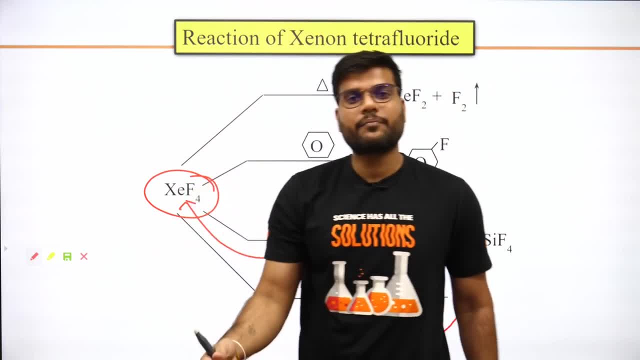 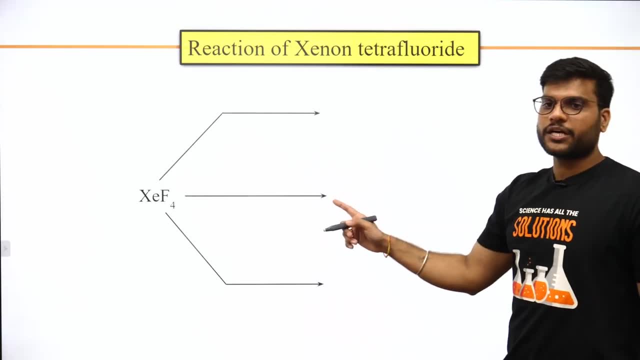 You will remember it. Now let's come to my important thing. I had said that it releases F- every time And makes complex compounds. I think it is the last. Now check the reactions of xenon tetrafluoride. Last reaction is 3.. 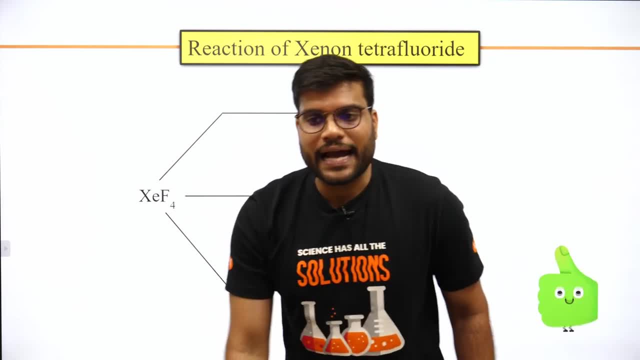 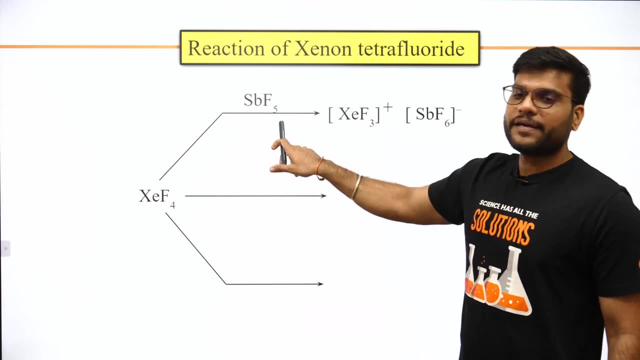 Only these 3 reactions. After that it is over. After that it is over. And what is this? Just check it. Assume I have made the reaction of XZF4.. SbF3, F5, right SbF5.. 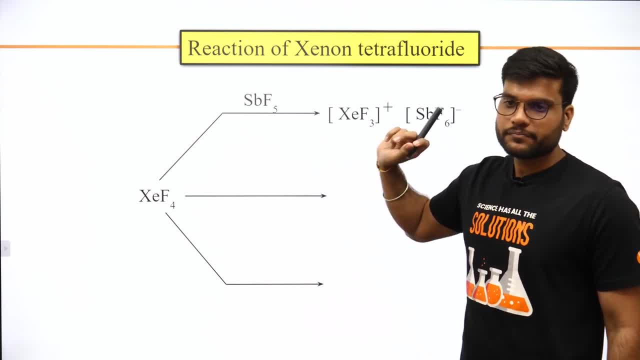 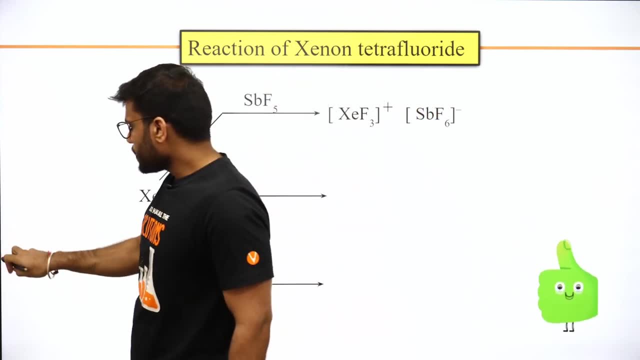 Antimony is done with pentafluoride. In that case, this one, fluorine, will be given to him. Now first tell me this All of you: Which group does this antimony come in? It comes in group number 15.. 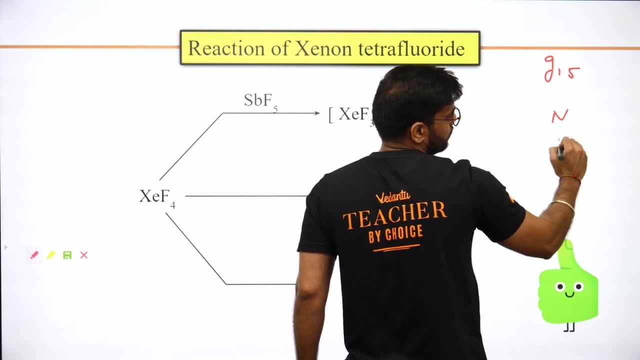 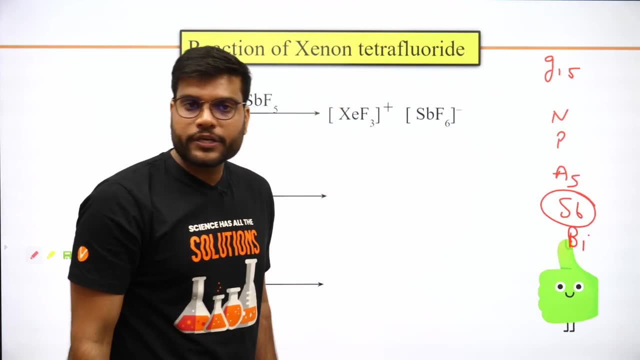 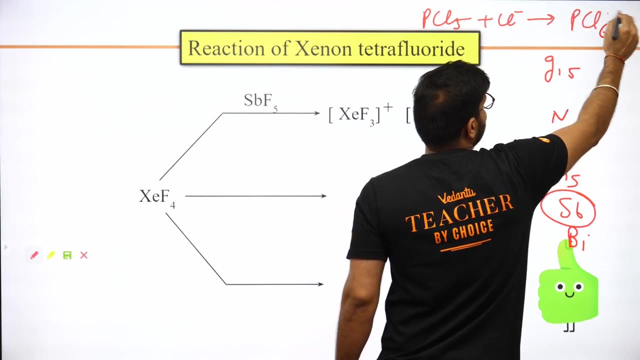 Do you remember? In group number 15.. I am telling you the method of remembering. Na P Sa. Between all of them- See this- came Antimony. Do you remember? Now, we should also know that PCl5 can make PCl6- with 1 chloride. 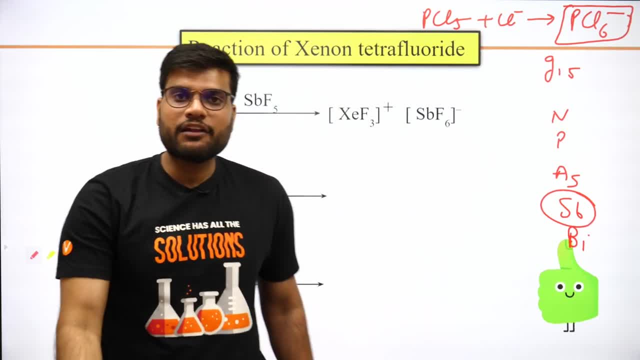 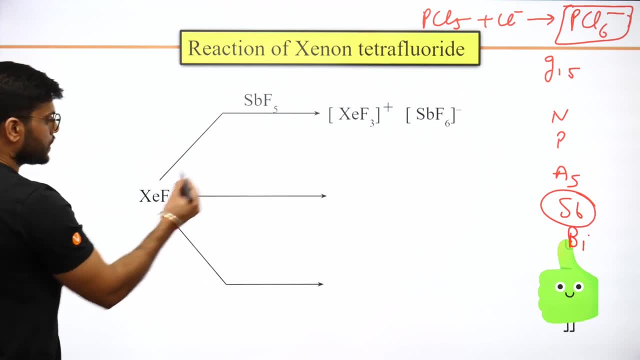 See, this: PCl5 can make PCl6- Does everyone understand this? Now? as soon as this can be made, then it can also be made. See, If XZF4 is made from SbF5, then 1 fluorine will go with it. 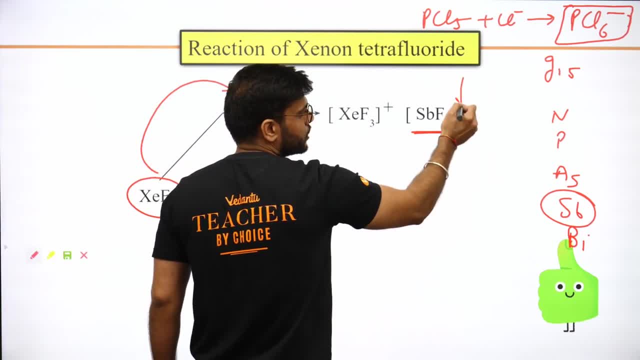 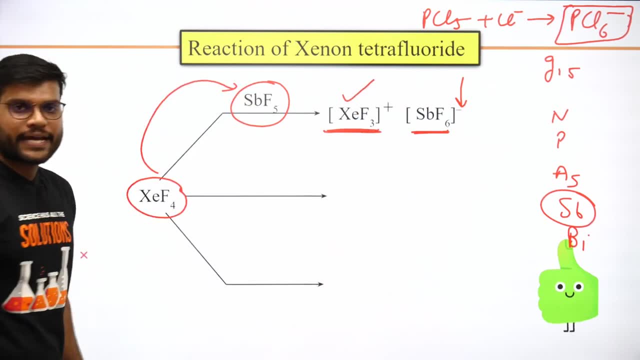 And what will it make? HbF6-? Just check, The same compound is also being made, The same. And what will it make from here? XZF3.. I had told you this, Do you remember? What is the special thing about XZF4?? 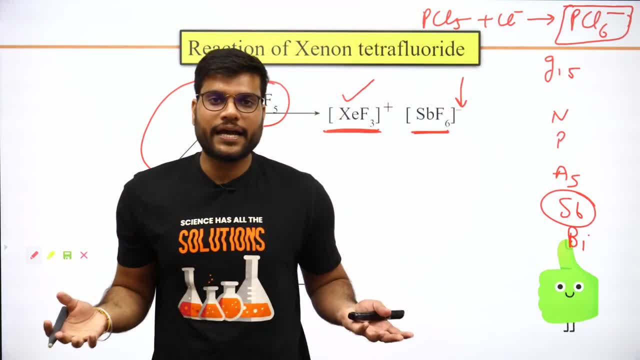 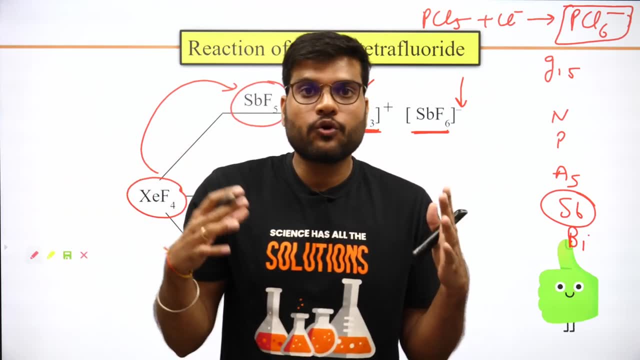 To give 1 fluoride ion. Take it. We have to give it, You have to take it. F- will give it to the person in front. You enjoy it. Your octet should be complete. You go above me. That's it. 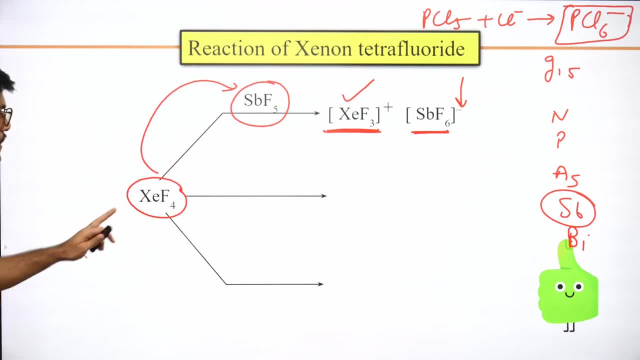 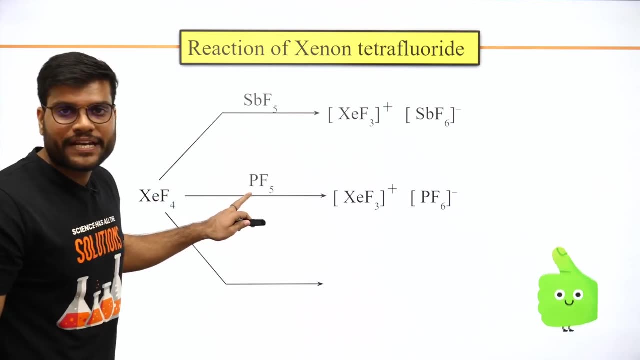 Is it clear? Now you come Last. This is our reaction. Now let's go. Suppose it makes a reaction from PF5.. So see that It comes above Sb and Sb Con. After 1,. 1 comes above. 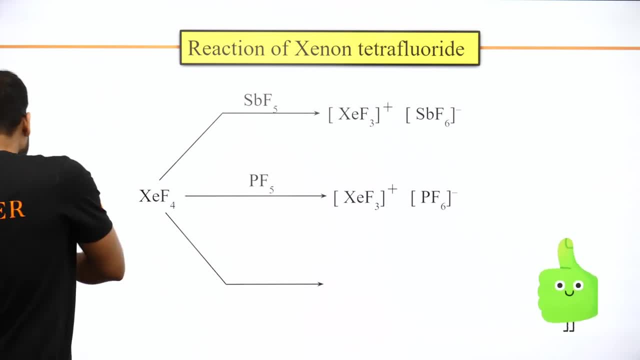 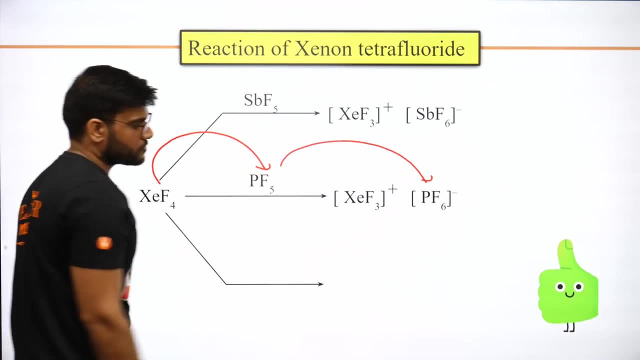 Phosphorus. So the same will do the same work. What will it do from here? It will take 1 fluorine, Just check. And what will it make? PF6- And in which is it converting Same Why? 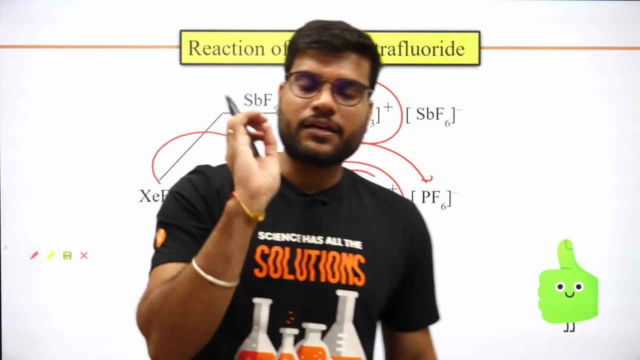 It is same. So is it hard? If we know the trick, What we have to do, Then it is not hard at all. I am telling the truth. Now, come to the last. Now you will be able to tell the result of the last. 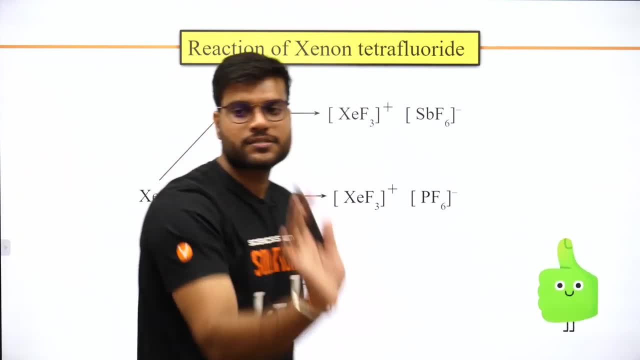 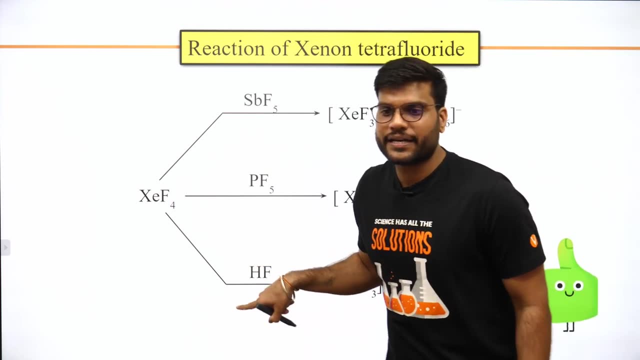 It is easy. Now you understood F- We have to stick it to the person in front, So the last is HF. What will happen in this case, In the case of HF? Yes, Give it 1 F- Just check. 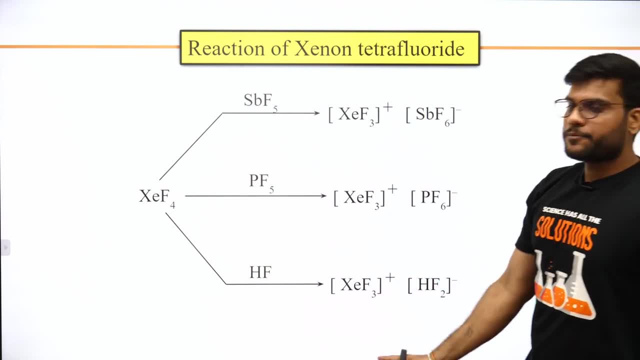 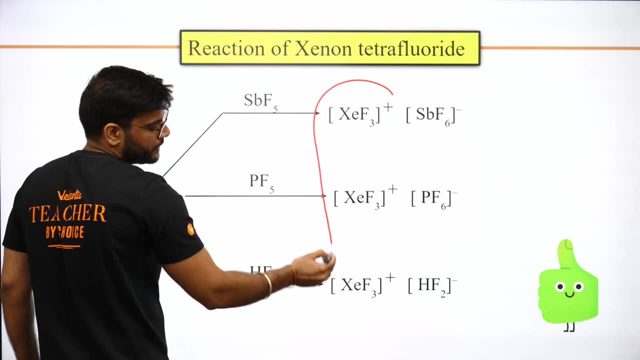 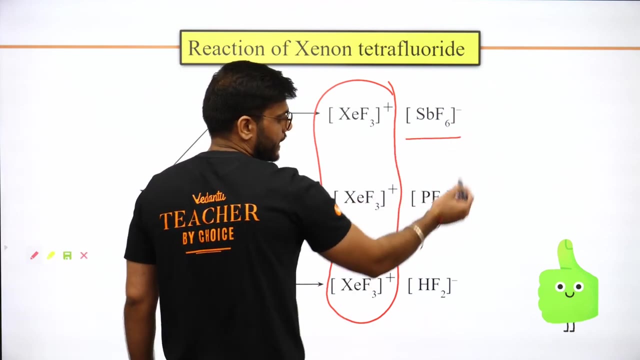 HF2- And it will make XZF3.. Now you check All three. You have done the same work in all three. Just check Here: this compound is common. This compound is common. Now this compound is left behind. This is 1.. 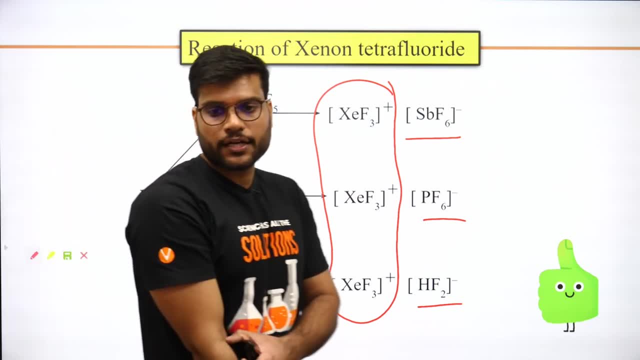 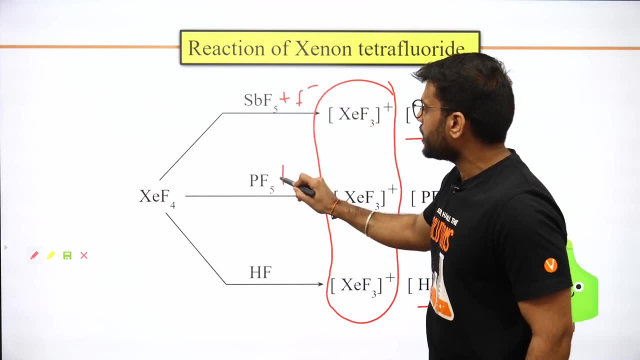 This is 2.. This is 3.. Check it, brother, Check it, And there is one extra fluoride in all. You will go from here. Put 1 F- extra. in all It is over. Put 1 F- extra. 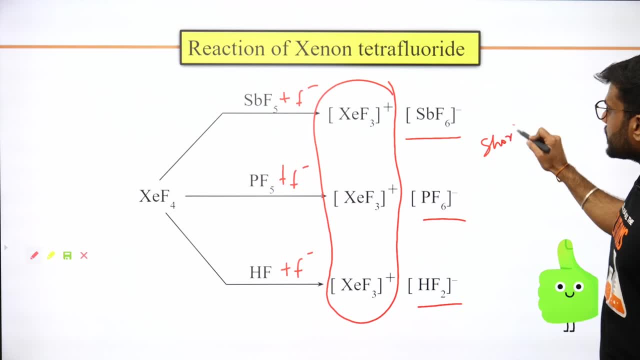 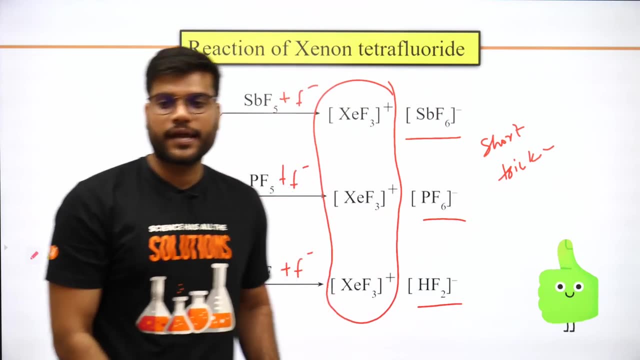 This is a simple short trick to remember it. I have told you the tricks so that you remember. So here our 18 number group is over. There is no easier way than this. You can note it down. Take a screen shot. Take a screen shot. 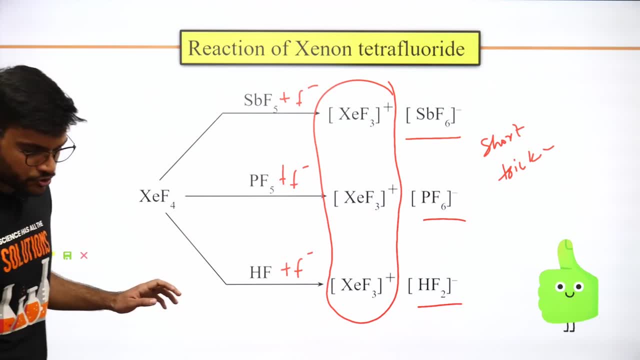 It is over. Take a screen shot: 1,, 2,, 3,, 4,, 5.. Take a screen shot, Come on. So finally, guys, We have finished the 18 number group. It is a very good thing. 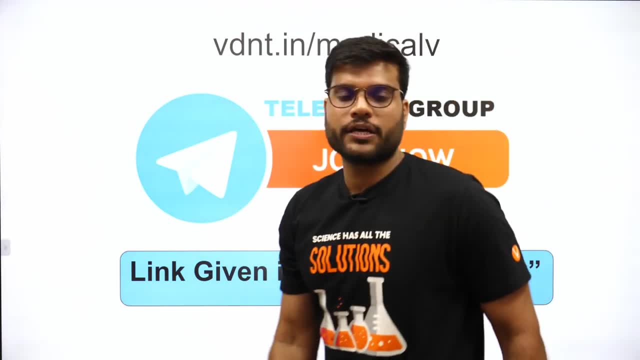 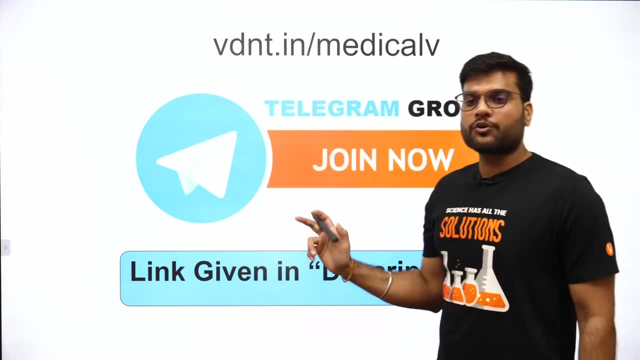 I will tell you all that you must join this group Because the new release will be in this telegram group, So you can join it at vdntin Slash. Join it. This is a telegram group which is very important for you guys. 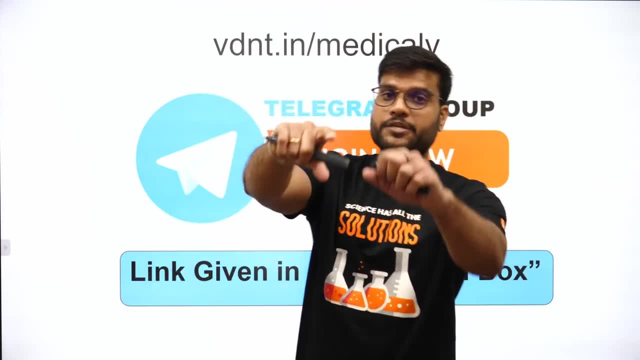 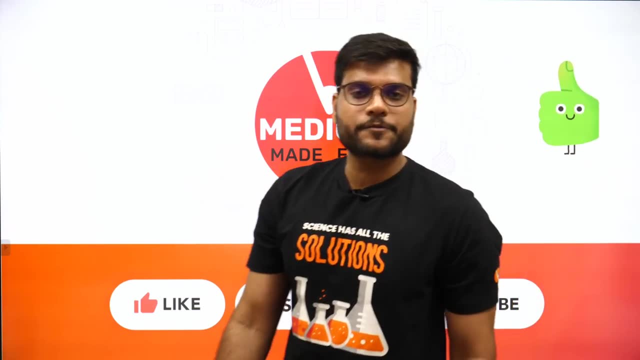 In the coming time we are going to make many series. I am telling you all that please join it, Okay. Apart from this, if you want to make Coaching Free India, then you will have to like, subscribe and share the videos. 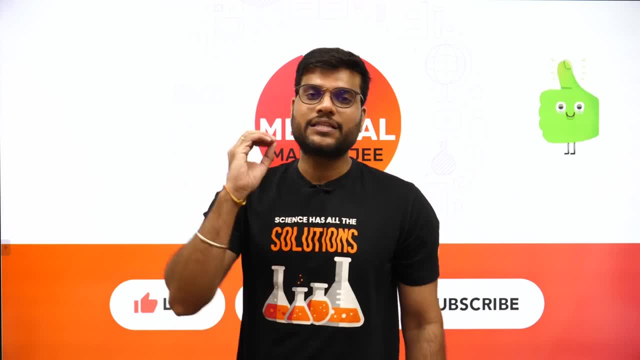 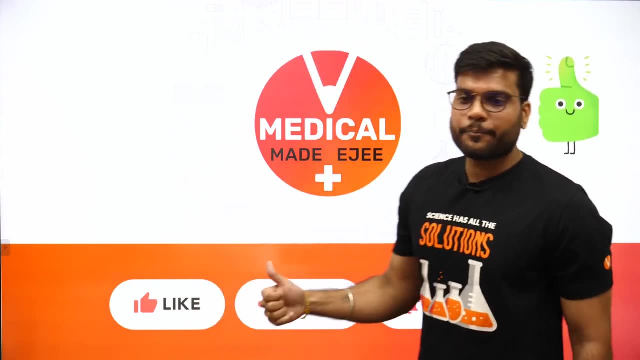 And how much time does it take to like? One click and like is done. Your 10 seconds can connect you directly with us. So connect with us. We will also like it a lot. So please like, share and subscribe, And it is very important to subscribe to the channel. 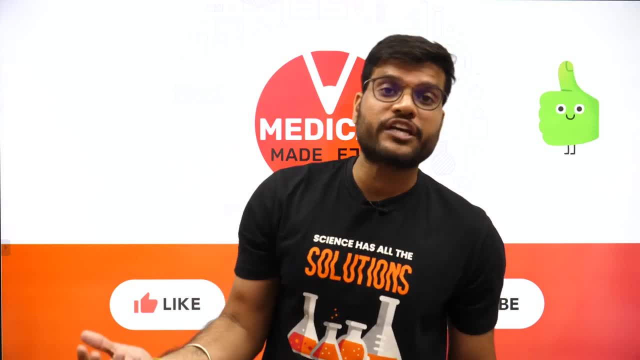 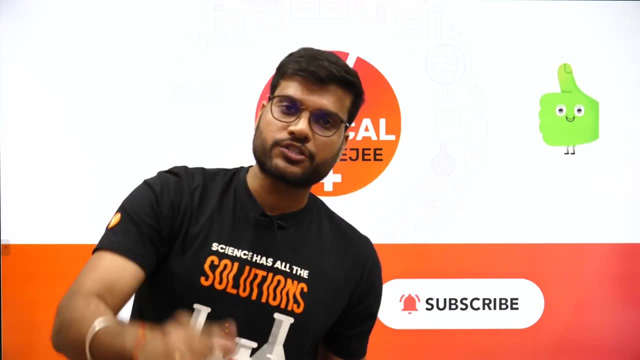 So that in the coming time, when there will be more live sessions, how will you get the notification? So do two things: Subscribe and join the telegram group. Whenever there will be live sessions, you will get its information, Because in the coming time, 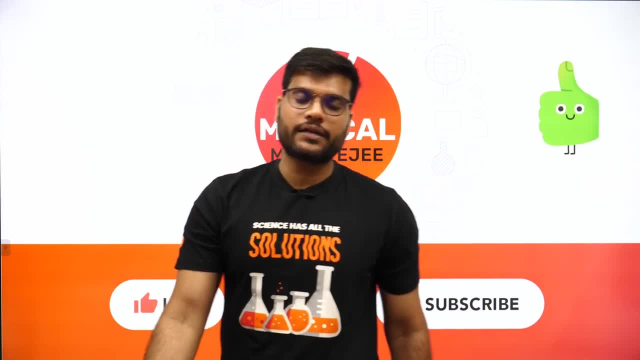 we are going to increase the frequency of live sessions for you guys And we are going to bring a lot of new things. Okay, So come on, guys. Thank you so much. Love you all. I think you guys have finished the P-Blog today. 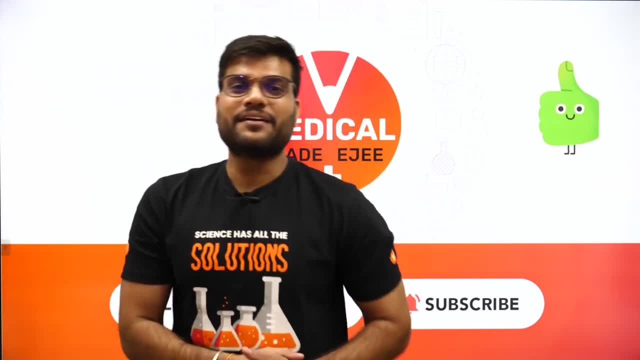 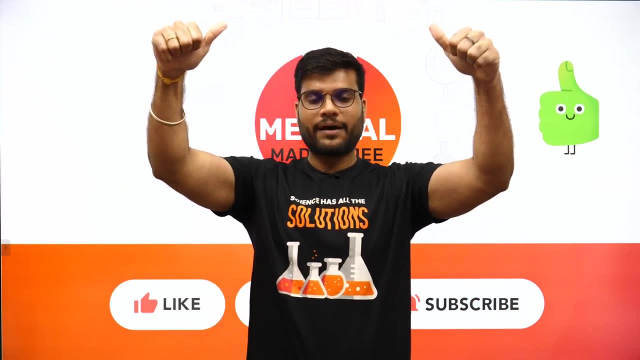 You must have enjoyed it. Right, It is over. It is over today. Okay, Come on, guys. Thank you so much. Love you all. This is Arvind Arora signing off. Bye-bye, Bye, guys. 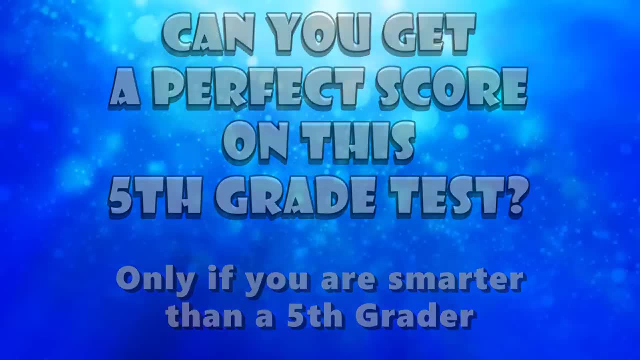 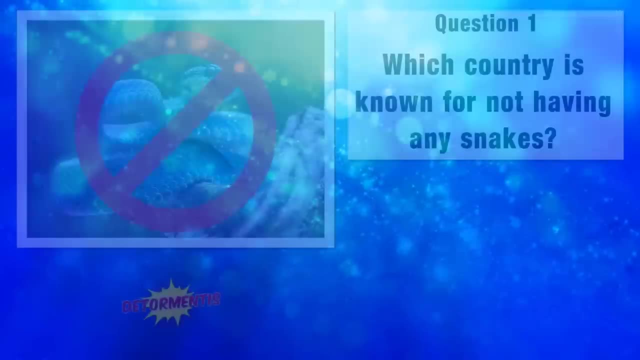 Here is a quiz that you will only be able to pass if you are smarter than a 5th grader. This is a collection of 20 questions that any student in the 5th grade should be able to answer. Let's begin. 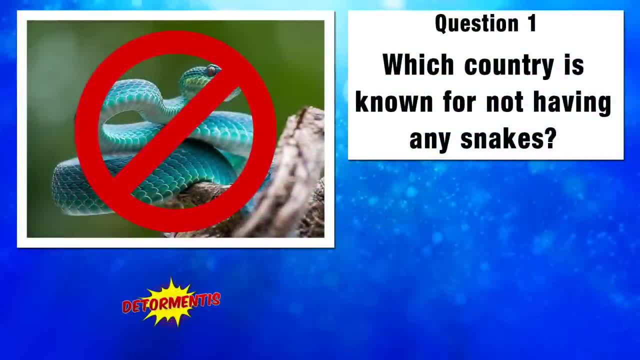 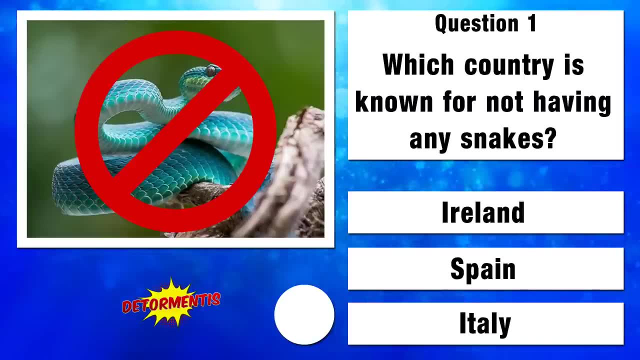 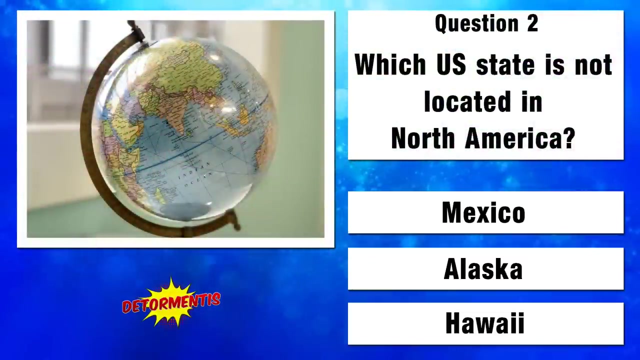 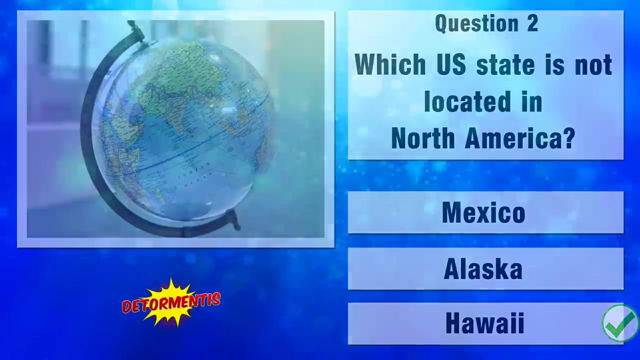 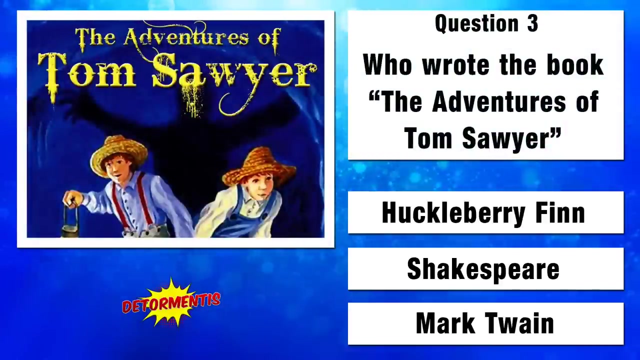 Question 1.. Which country is known for not having any snakes? Ireland, Spain or Italy, Ireland? Which US state is not located in North America? Mexico, Alaska or Hawaii, Hawaii? Who wrote the book The Adventures of Tom Sawyer, A Huckleberry Finn?